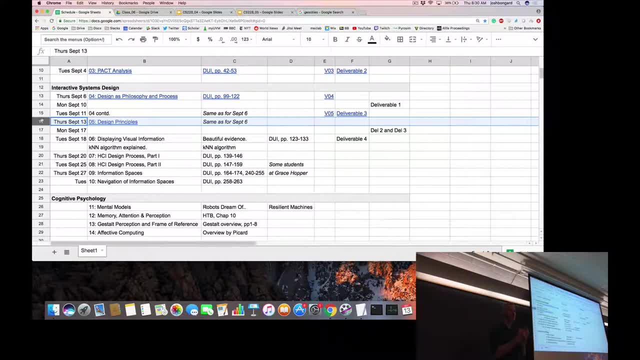 Jack the TA will be there for his office hours and also on Friday, So if you need any help with Deliverable 2 or 3, make sure to connect with Jack the TA to see if he can help you. While we're on the subject of Deliverables 2 and 3, any questions? So far, so good. How? 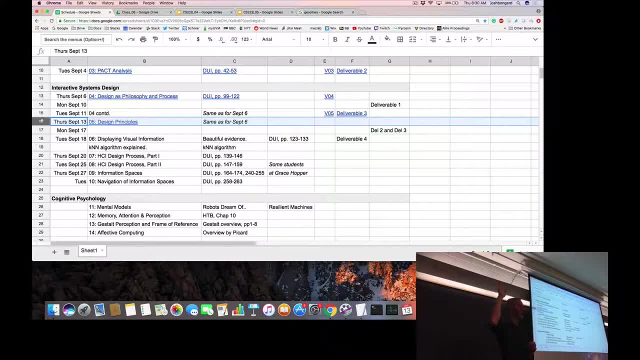 many people have dove into Deliverable 3?? Okay, about half of you. That sounds good. Just remember, it's pretty long, pretty involved, so don't leave it until the night before Again, friendly reminder, Okay, Okay. 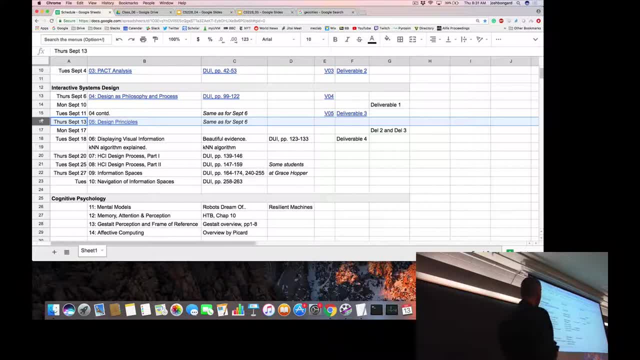 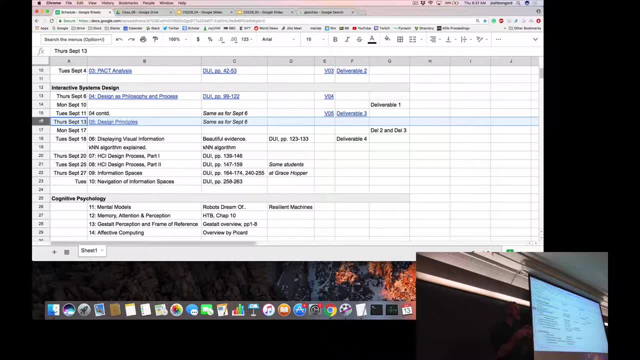 aspect of HCI design is trying to make a lot of these intangibles and these sort of vague aspects of what is going to become the interaction between your user and your system, to try and make them explicit right. A lot of them are missed during the design process and can. 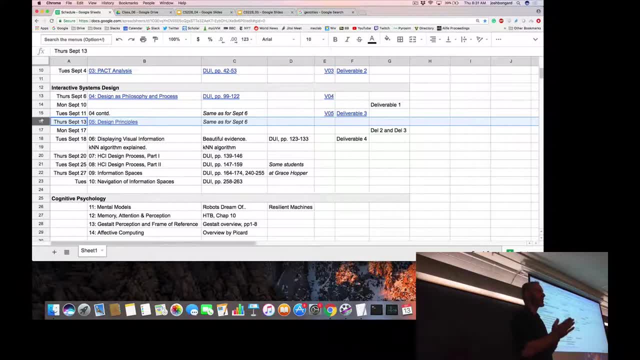 have a lot of time to look at them and try to make them explicit. So I think that's humorous or possibly disastrous consequences after your system is deployed. So just keep that in the back of your mind as we continue our discussion about design. The black art of HCI is recognizing, before it happens, what aspects of human diversity 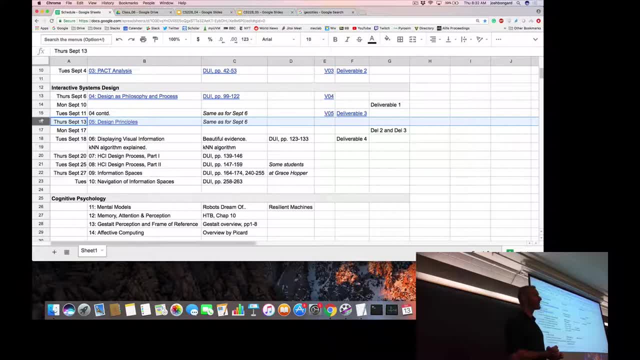 might cause an issue when the system is finally deployed. Okay, just a little bit about where we're going. As you realize, Lecture 4 is a little bit long. I promise we're going to finish it today and make our way through Lecture 5, which is a little bit short. 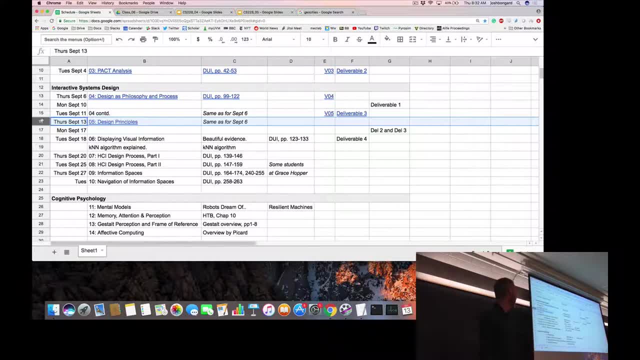 We may or may not get to the first or second slide of the sixth class, which I have not put up yet, but we'll definitely tackle that in its entirety next time. Next time we will also talk a little bit about Deliverable 4,. 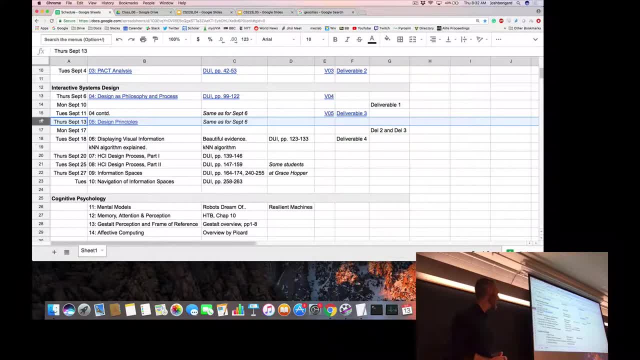 where you're going to be introducing a little bit of machine learning into your system. This is not a machine learning class, so we're going to use a very simple machine learning algorithm, which is known as K-Nearest Neighbors. Who has heard of K-Nearest Neighbors before? 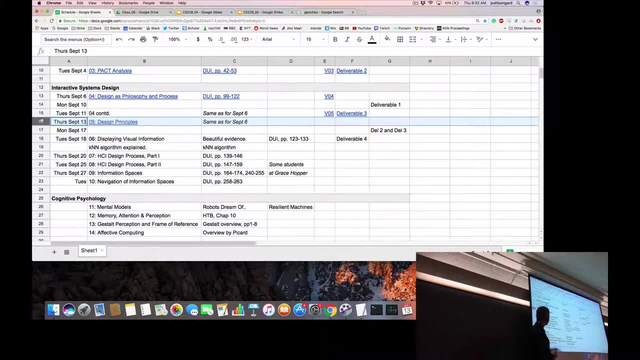 Just a couple of you. Okay, that's good news. We will take a fair bit of time on Tuesday to actually talk about what the K-Nearest Neighbors algorithm is and how it works, and you're going to then be implementing it in Deliverable 4,. 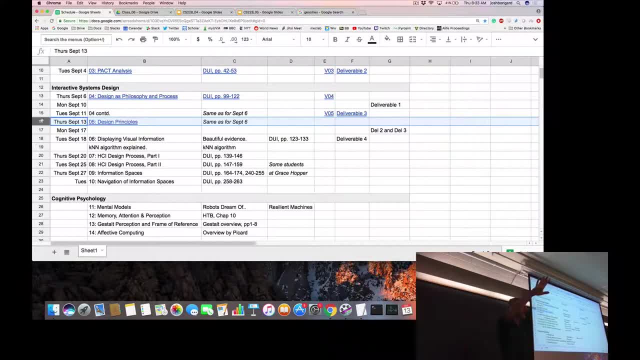 just as a reminder, to translate the XYZ coordinates of all the bones in the hand, to take those 120 numbers and turn them into just one number, which is a number between 0 through 9, and that number which is output by your K-NN algorithm. 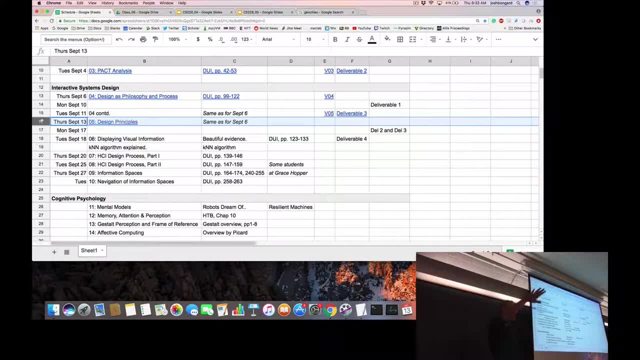 is going to be the algorithm's guess about which of the 10 ASL numbers your user is currently signing above the device, or that they're not signing any of the 10 numbers, right? So just as a reminder, Lead Motion out of the box comes with some machine learning. 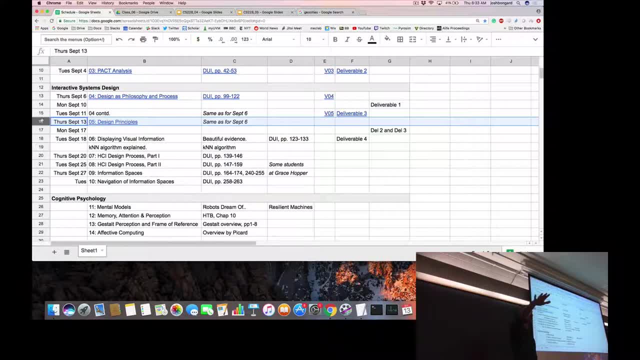 that takes the values of the pixels from the two infrared numbers and then it takes the values of the pixels from the two infrared numbers. and then it takes the values of the pixels from the two infrared numbers and then it takes the values of the pixels from the two infrared numbers. 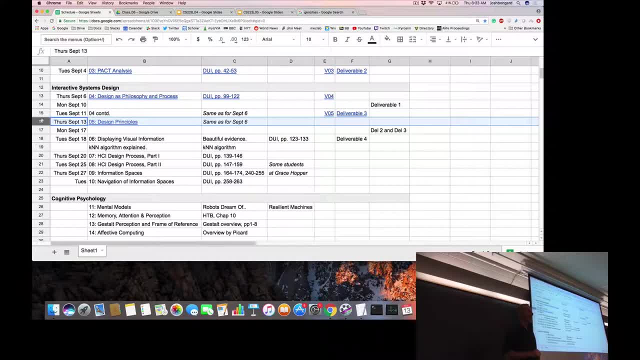 and turns that into XY and Z coordinates. As you've already noticed, most of the time it does a pretty good job, but it's definitely not perfect right? Same thing will be with your algorithm. Okay, after that, we'll continue on with our discussion about the design process. 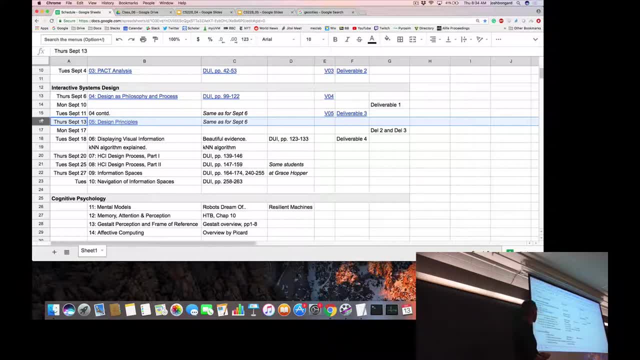 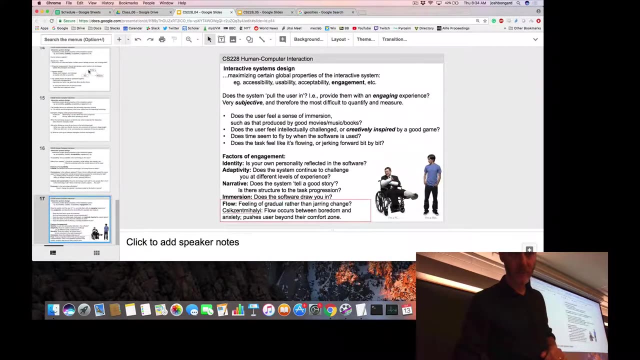 and talk a little bit about information, spaces and navigation, and then in a couple weeks we'll get to talking about not technology and design, but people. So let's jump in. So let's jump back to lecture four. We haven't quite finished lecture four yet. 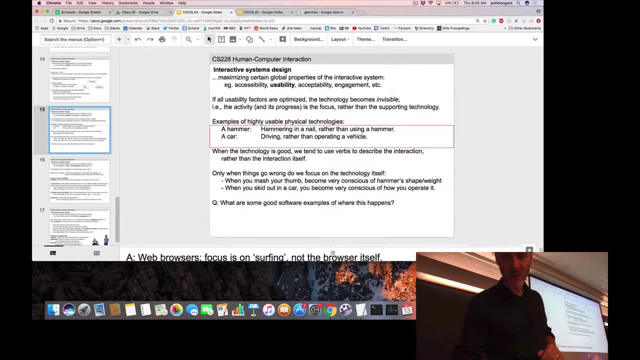 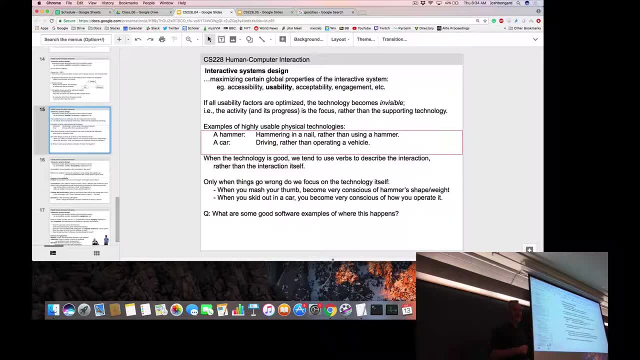 And we ended last time. We ended last time by talking about this idea of verbification. right, One of the things you'll realize in user testing of HCI is that often the user will say, ah, this is frustrating, I don't know how to use it, I'm done. 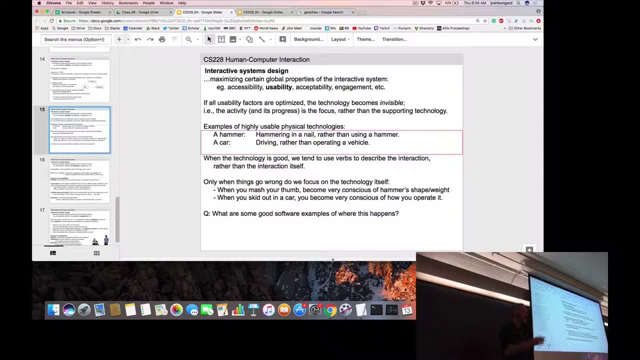 Or this was great, it was very usable, but there's a lot of vague terminology, right? So how do we actually figure out how the user, what aspects of your system are working well for the users and what aren't, And sort of tongue-in-cheek? we ended last time with this idea of verbification. 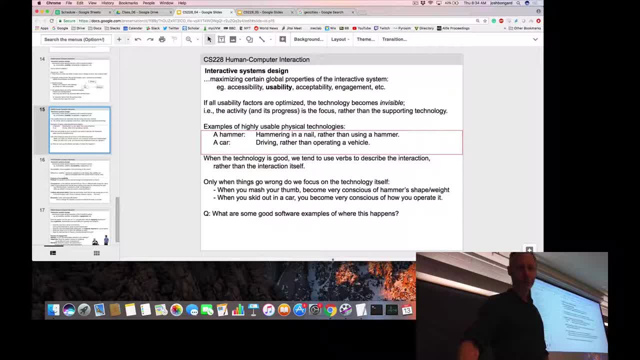 If you create a really great killer app, your users are going to verbify it. Okay, Just to take a step back. remember we were looking at these four global properties of an interactive system. So in software engineering we're usually trying to take a bunch of written requirements and turn them into code. 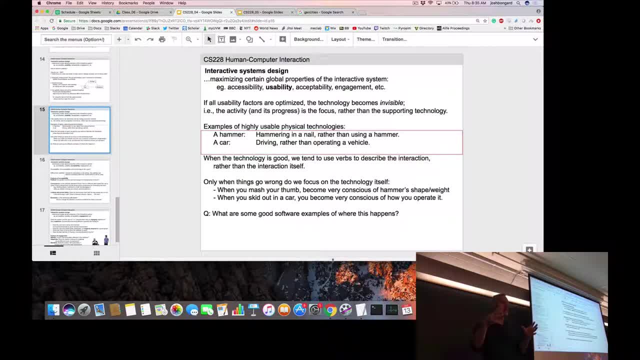 In HCI we're trying to take written requirements and turn it into code and also maximize or optimize non-functional requirements. So these are requirements, things the system should have or should do, which aren't directly related to the function of the system itself. right? 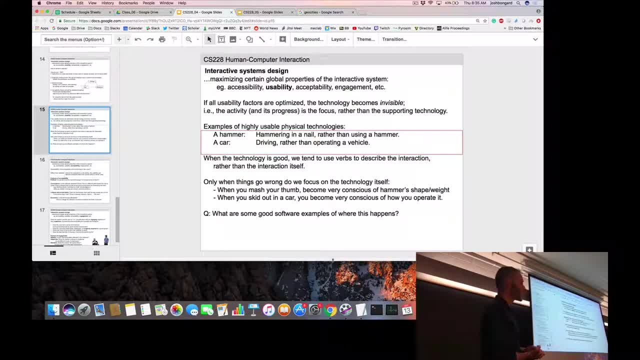 The system should be accessible, usable, acceptable and engaging, which again are kind of vague umbrella terms. So what exactly do we mean by these things? Last time we were unpacking some of these terms, We looked at accessible and usable. 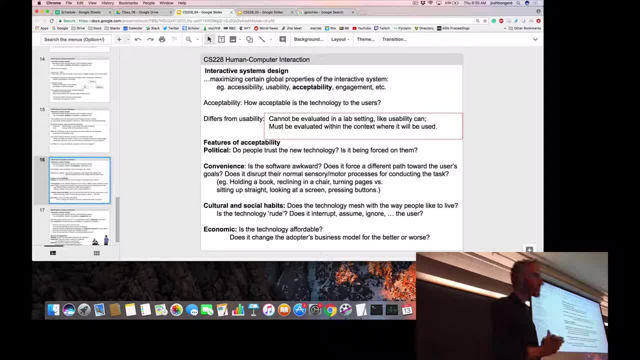 And usable. sorry, accessible and usable. let's move on to acceptable. And as we're moving from left to right in these four non-functional requirements, as usual we're moving from things that are sort of more objective and easy to measure. 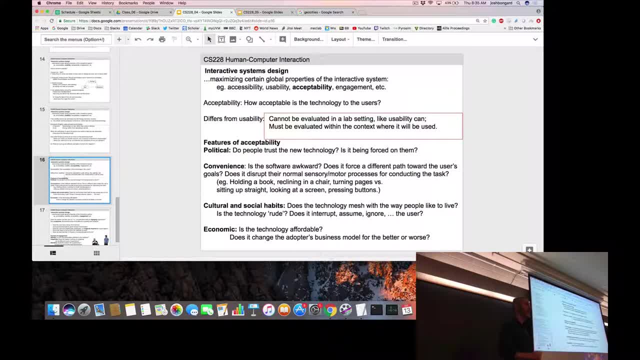 And when I say easy to measure, I mean easy to measure during a user interaction. You can deploy your system to a thousand users and see how many of them actually can use it. Now you know how accessible. it is. Pretty easy to measure. 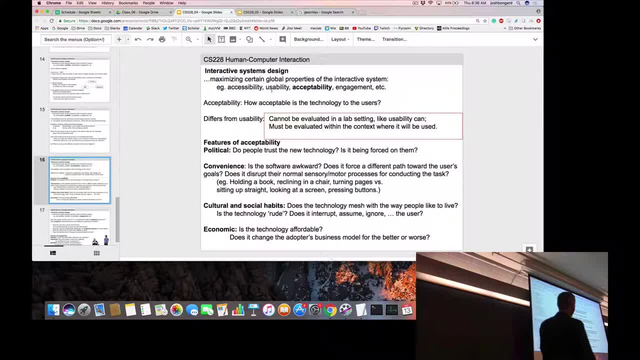 Usability is a little more tricky, but we talked a little bit about how to measure that. Acceptable and engaging become a little bit more subjective and a little bit harder to measure. Systems may be usable. They may have a beautiful interface, They may be simple. 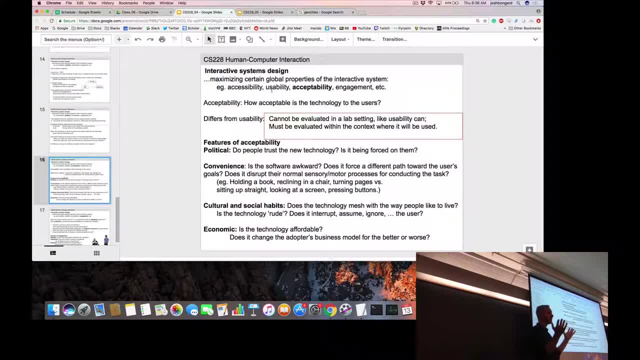 The user may require no manual. They understand how to use it, But when you deploy your system out into the world? so you've done all your user testing in the lab at the company that you work at with your users, They've come in, used it. 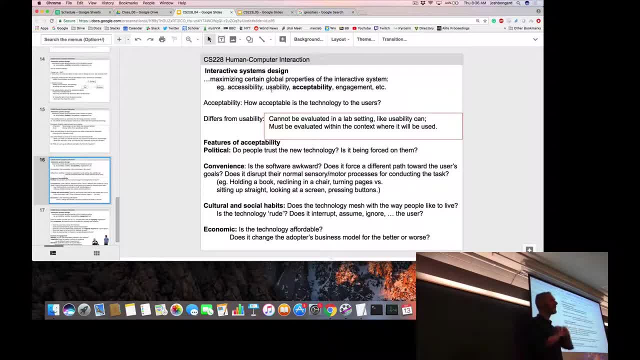 They said it's perfectly usable. I love it. It's great. You deploy it out into the world. No one buys it, Nobody uses it. Usability and acceptability are quite different. So just a take-home message from this: to remember the difference between usability and acceptability is. 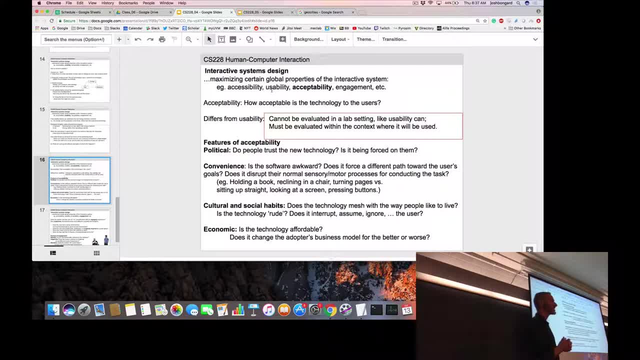 acceptability is usually not something that can be tested in the lab setting. It has to be tested in the field, Right. It has to be tested out there in the world. We already talked about one particular technology which was very usable but absolutely not acceptable. 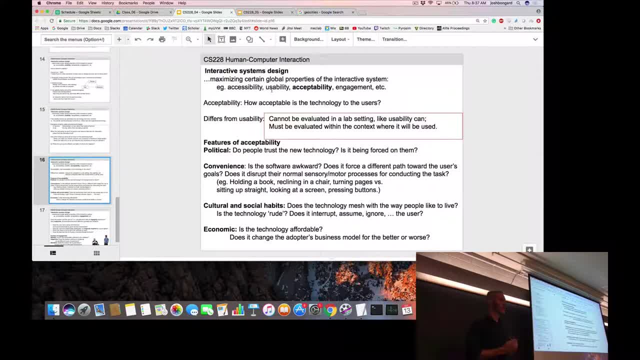 What was that technology? Google Glass. Google Glass right Works well for the people wearing it, But once people are wearing it and they go out in the world, other people didn't like it. Why didn't they like it? We'll talk about that in a moment. 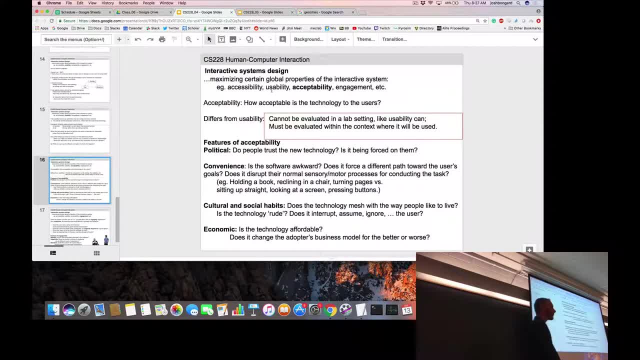 Okay. So again, let's try and unpack acceptable. If people don't accept it, why don't they accept it? So perhaps there are larger political reasons why people won't accept it. People may not trust the technology or it may be forced on them. 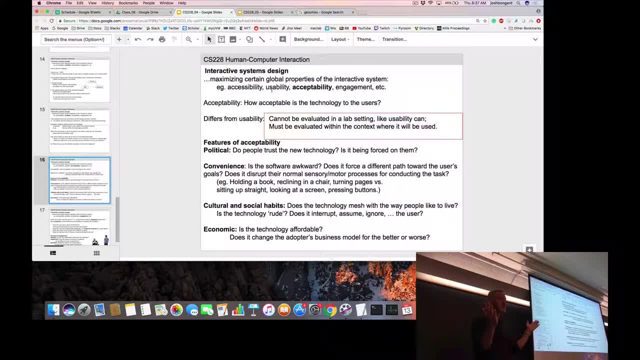 I've mentioned the fantastic software system called PeopleSoft before. I hope you have not experienced that here at UVM. But if you're a teaching assistant or a postdoc or a faculty member or staff- someone who gets paid at UVM- you've worked with this system. you have no choice. 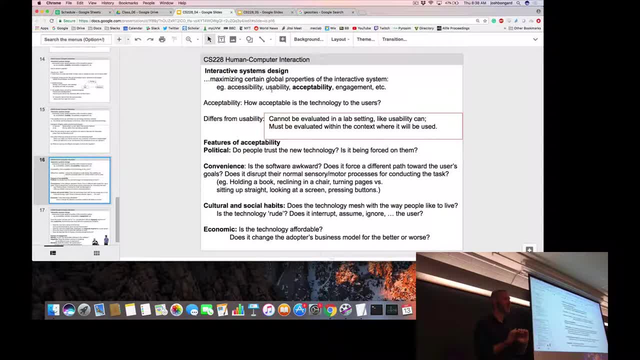 If you want to receive a paycheck, you will work with PeopleSoft. Unfortunately, PeopleSoft is also not very usable, but that's besides the fact, right? So is it being forced on people? How are people having to use this system? 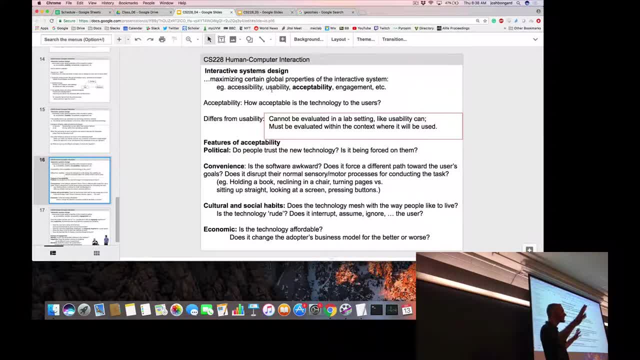 That's obviously important. That has maybe nothing to do with the system itself, It's the larger social context around it. Then there's the issue of sort of convenience or ergonomics, which we talked about before, which is kind of the fit of the technology. 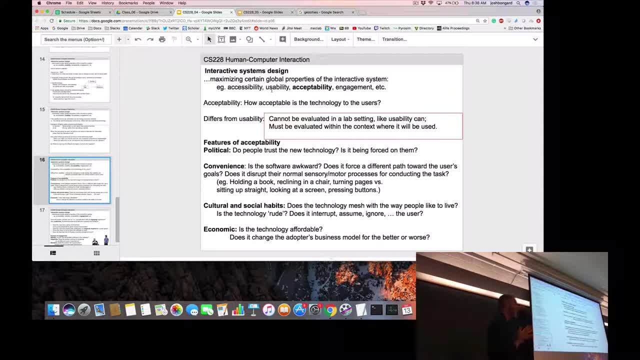 The fit of the technology with the person. If you're designing a new cell phone or a video game controller, something that someone is actually going to hold- then ergonomics usually means the actual three-dimensional shape of the system. Does it work? 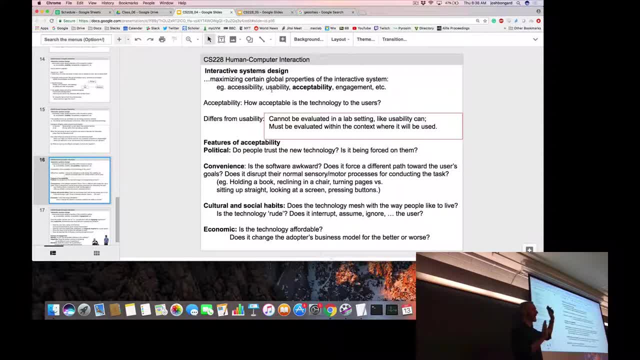 Before these things became standardized, there was a cell phone technology out there that had the pad, the keypad for buttons above the screen, which didn't work. It wasn't acceptable. Why not? Absolutely right. So it was thought that people might actually hold it and type like this. 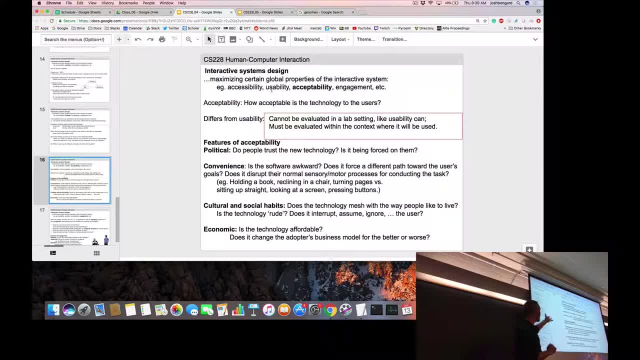 I know it seems crazy, but that was the idea. Then, when you gave people these crazy new things called smartphones, people tended to use their thumbs, which was just convenient. That seemed to be the way that you do it. For most of us, that is the way that we do it. 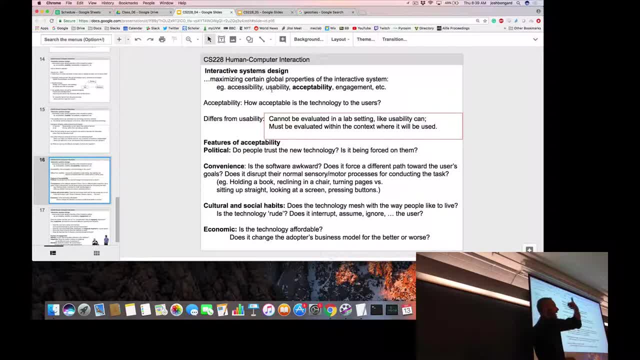 Of course, if you're holding it, you're holding it in that way and you're trying to thumb keys at the top, then obviously your thumb, the meat of your thumb, is occluding the screen. That didn't work very well. 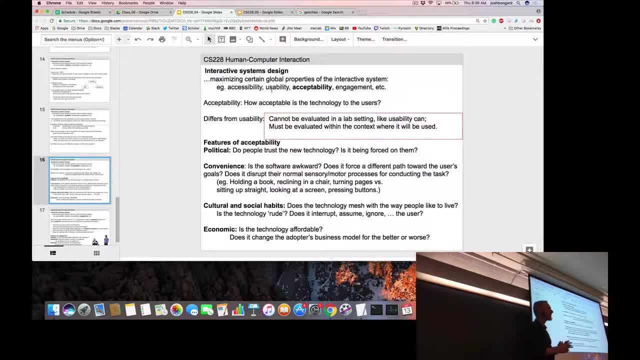 Those are sort of ideas about convenience or this idea of ergonomics, which is sometimes literally the fit of the technology with the person. Sometimes ergonomics means sort of a fit in a metaphorical sense. Do they interact with it in the way they would want to interact with it? 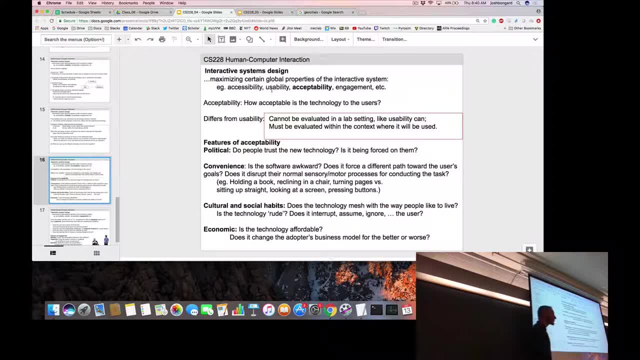 That was a very important issue Again when e-books were sort of trying to break into the market. how many people like to read e-books? Some, but not all. It took a long time before it was actually sort of comfortable for people to read an e-book. 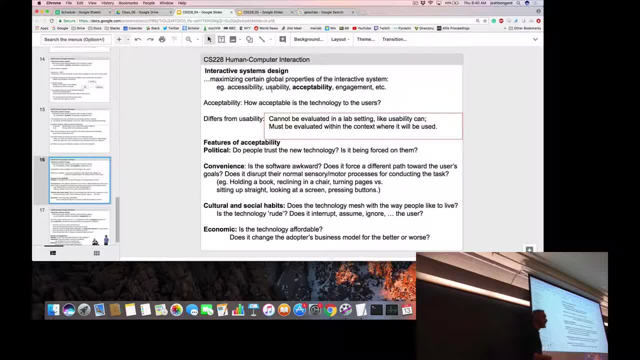 What's the reason? The reason is that a non-e-book, a traditional book for most people is kind of comfortable, right. There's no user manual for a book. You sit back, You can usually relatively easily find your place. You thumb from one page to the next. 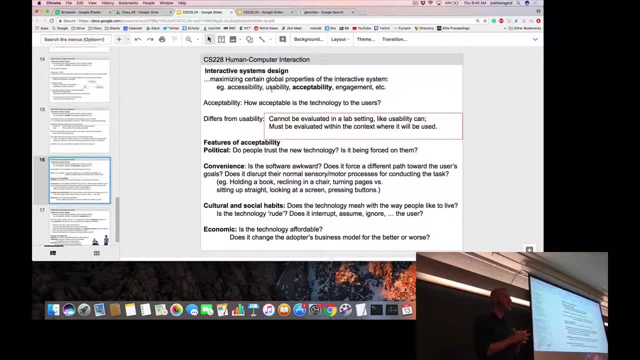 and off you go right. What were some of the issues about e-books? even if you don't remember those issues when they were being introduced, What would you imagine are some of the very important acceptability factors that you need to get exactly right? 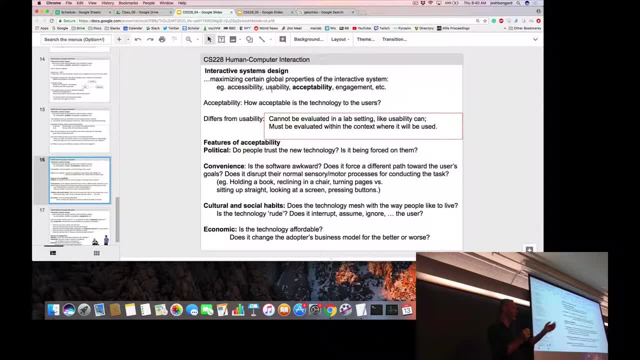 for someone to choose to pick up an e-book over a book. Battery life. Battery life is important, and that's true for sort of all mobile technology. right, Let's really focus on the e-book. What are some of the things that people tend to do? 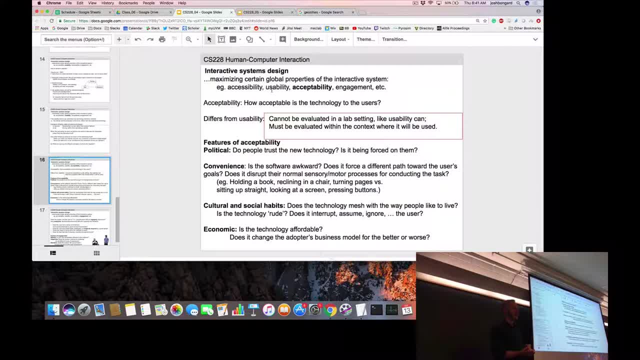 when they're reading an e-book. What are some of the things that people tend to do when they're reading an e-book? What's the main act of reading a book? A lot of them have like a shiny screen so you can read it outside. 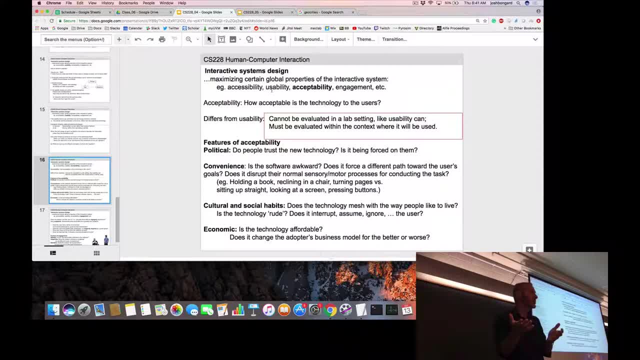 Absolutely A shiny screen. So what do people tend to do? They tend to read, sometimes indoors and outdoors. I don't want to have to have a book for when I'm reading outdoors and my e-book for when I'm reading indoors, right? 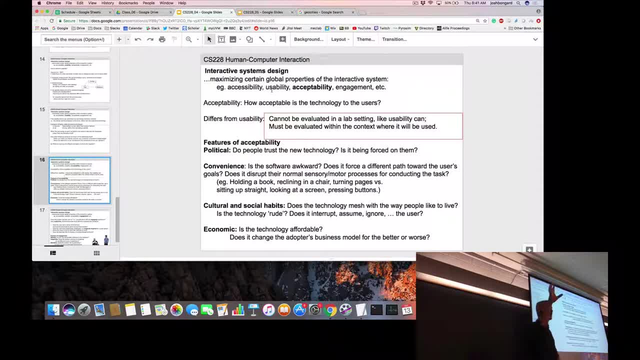 That's inconvenient. I don't want to switch back and forth. If I'm going to read novel X, I'm going to do it all on an e-book or on a book and, of course, reading part of that novel. sometimes I might be indoors. 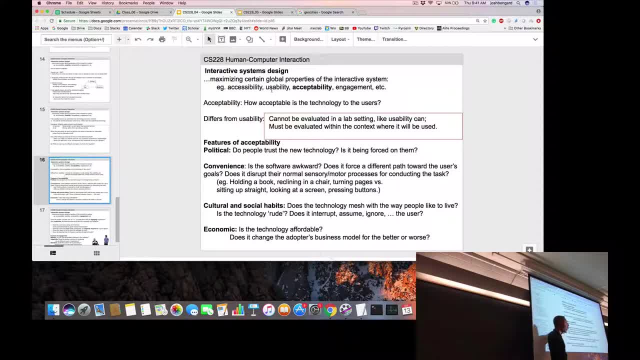 sometimes I might be outdoors. This is again all thinking about the C in PACT analysis: the context, the physical context around the act of specifically reading a book. So that was important. right To get the screen right to not be very reflective. 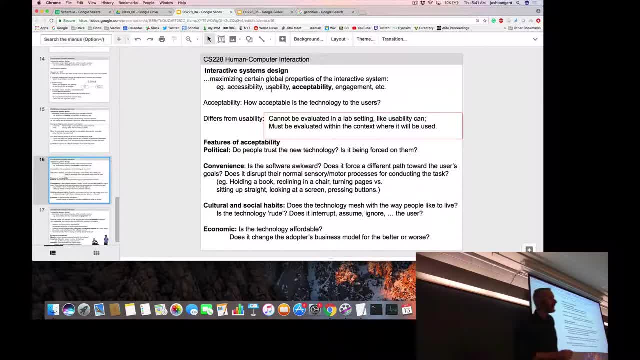 What else? The screen size was an issue. I just heard you put something like an old smartphone and you have to scroll just all the time because there wasn't enough space Scrolling, right? That's a pain, right, If you open an actual book. 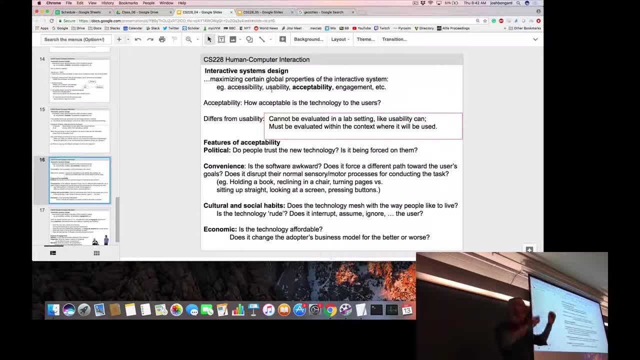 it says. it sounds ridiculous, but you're not actually scrolling anything with your hands. Your eyes, saccade, I mean your eyes are moving from word to word on the page, but you're not doing anything with your hands to focus one part of the page right. 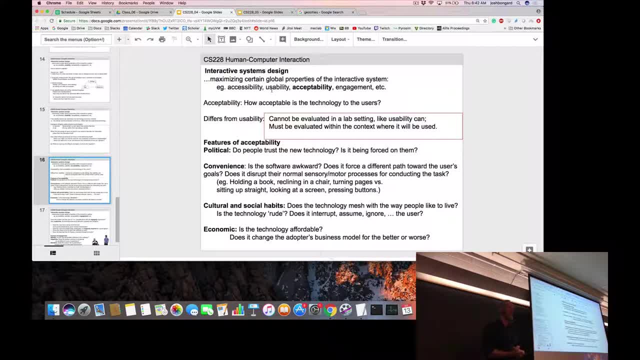 So that was a difference between early e-book interfaces and actual books, which was not acceptable to a lot of users. What else? Yep, Absolutely right. So getting the reader technology to the point where it was light enough or small enough or thin enough. 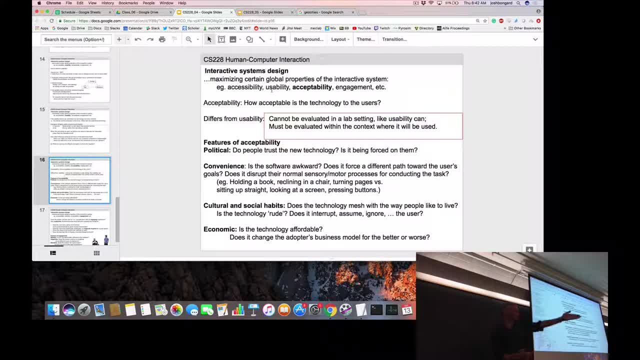 that it actually kind of felt like a book. That was important, Yep. So if you wanted to go back a bunch of pages, you had to scroll back. Was that a good thing or a bad thing? Sorry, It's a bad thing, right. 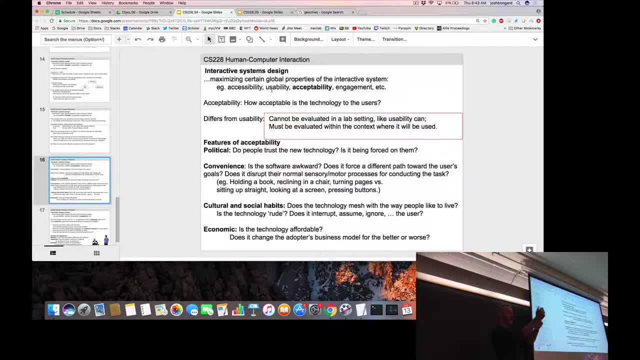 You have to kind of do that Often in a book. you can sort of look at John and go back about 20 or 30 pages and maybe one or two swipes. In the old days you had to do page by page right. 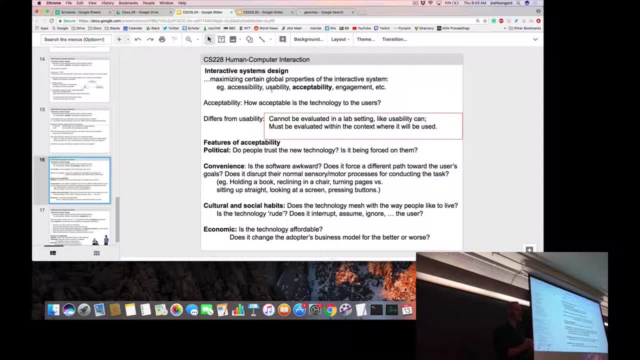 What else? Getting very close to one of the things that was particularly difficult, We just kind of indirectly mentioned it, Annotating that's important, right? So the highlighter, that was important as well. Keeping your place right. 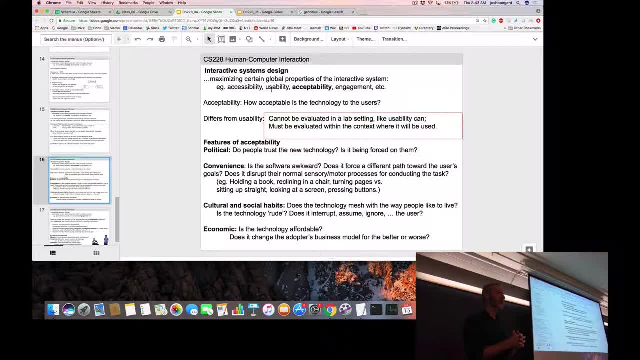 That was important. Think about the physical act of reading a book, Turning a page right. This was actually the sticking point for a lot of people, right, This or this or however you turn a page in your book. I don't know if that's still true. 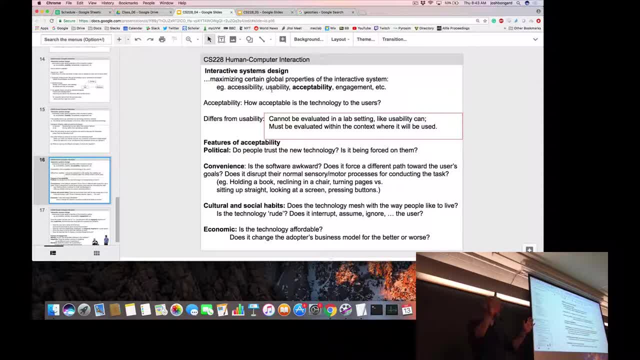 but a lot of the e-book interfaces went to a lot of effort to create the illusion of actually turning a page. So if you touch the screen and you pulled, the text would actually deform and warp and flip over, so it looked like you were literally turning a page. 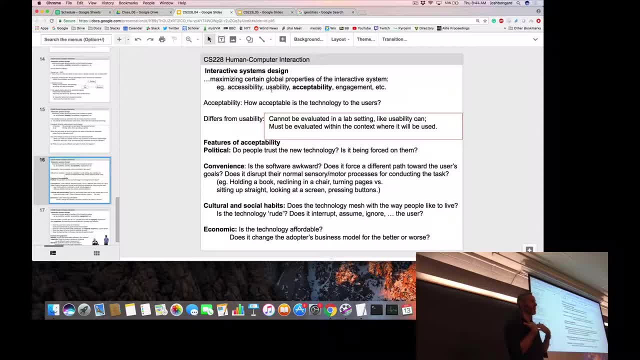 That was important for us old people who were really trying to go from books to e-books. Maybe that doesn't matter so much anymore, but there was a lot of effort that went into the act of turning a page in an e-book. That was the difference for a lot of users. 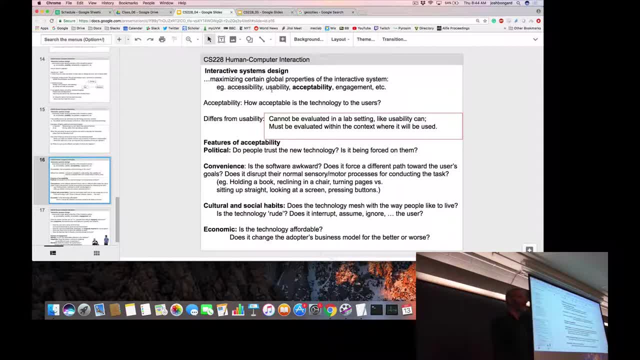 between whether an e-book was acceptable or not, Very, very important. Okay, Some of those aspects. again, you could count them as usability, The good point about being indoors and outdoors- not something you can really test in a lab, right. 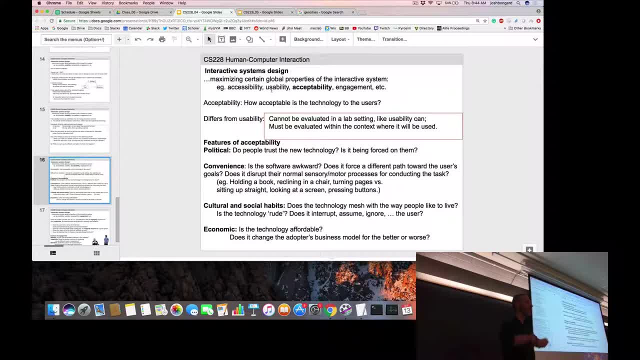 You can sort of try and get some of the interface right, deploy a bunch of e-book readers to readers, have them go out and do their daily activity and use the e-book on the subway, on the bus, outside. however they read during the day. 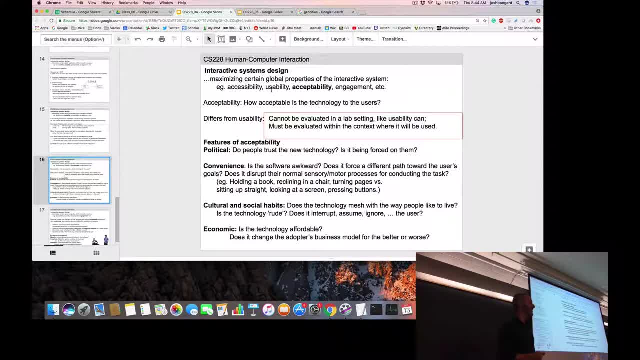 and see whether the e-book can actually stand up to that. That's acceptability testing. Okay, Culture and social habits: we've kind of talked about that before, So again now we're not really talking about the physical context so much. 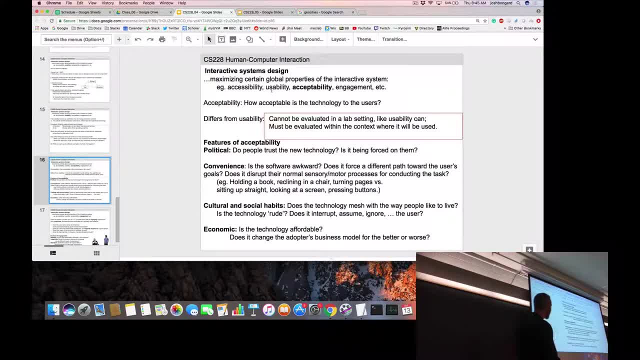 but more sort of: does it fit in with your life as a whole? Does the technology mesh with the way people like to live? Is the technology rude? Does it interrupt, assume, ignore the user, and so on? right Again, a little tongue-in-cheek here. 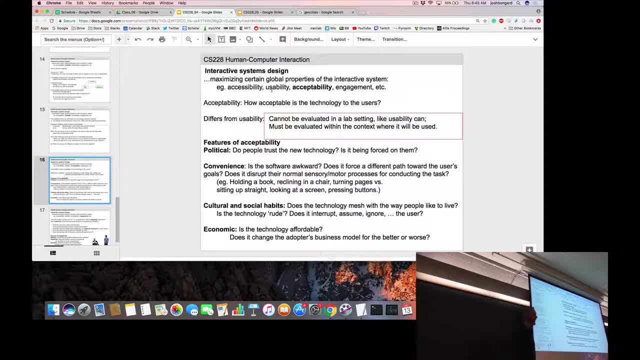 but we do want to make sure that our technology is polite. What do we mean by politeness or rudeness, Or can you think of examples of rude technology or polite technology? I know people like to put out Duolingo. Okay, It's a very aggressive notification. 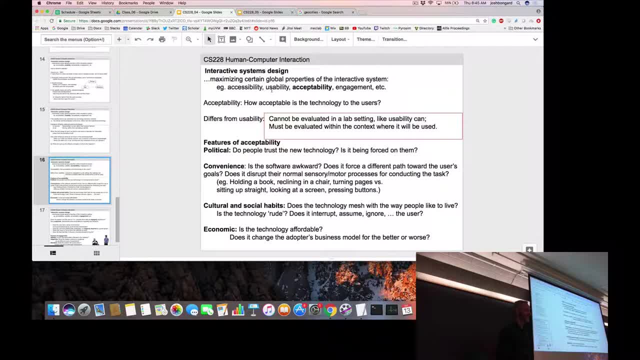 when you stop doing its lessons. So it'll be like: Hey, where'd you go? Hey, come back, Absolutely Like repetitively says something. That's very true, right? The Duolingo system is known for this aggressive notification system. 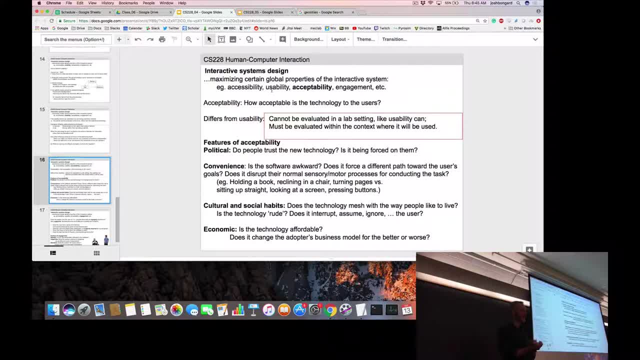 And you said it reminds you, but it's not an it, It's a he or a she. Yeah, it's an owl. The owl, That darn owl right Looks lovely and of course it's an owl, so it's wise. 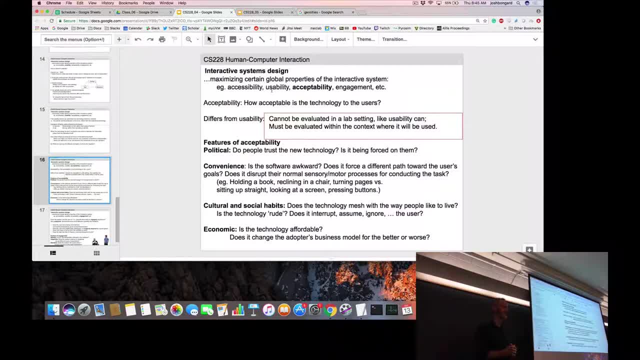 It's all about learning. It's calling you to a noble purpose, right? I know you're scrolling through Instagram. Whatever you're doing, it's not as cerebral as what you should be doing, which is spending time with me learning another language, right? 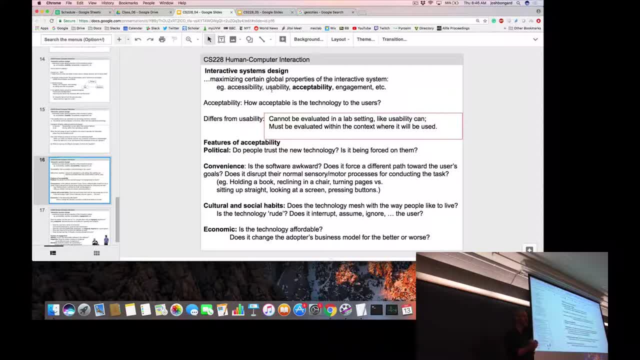 So they thought they could get away with some of that aggressive notification because again, it's not calling you back to social media, It's calling you up to learning and language and so on. right, But again, I don't know, It might make you feel bad. 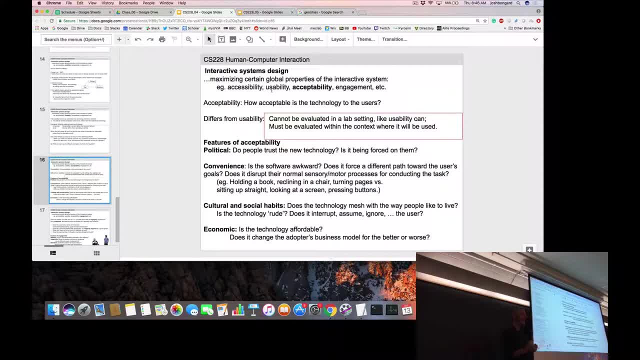 but in a way it's being not maybe rude, but a little uppity. right, You spend time with the owl? Yes, A little less complex, but microwaves that don't stop beating in the middle of the day, Absolutely right. 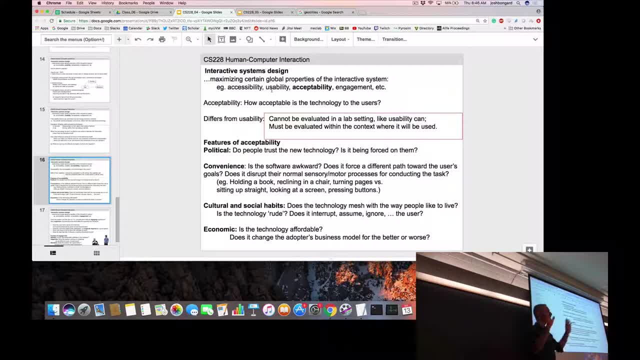 Our world in general. right Notifications. Thank you all. This is our fifth lecture and I have not yet heard a cell phone beep. Thank you for that. In the old days, not so much right. We're all, as a society, learning how to deal. 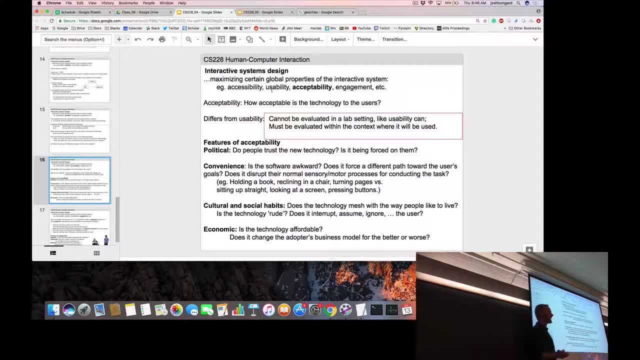 with all our devices which are constantly notifying us about all sorts of things. right, In the old days it wasn't rude, because there just weren't that many devices and there weren't that many apps. There weren't that many apps, right? 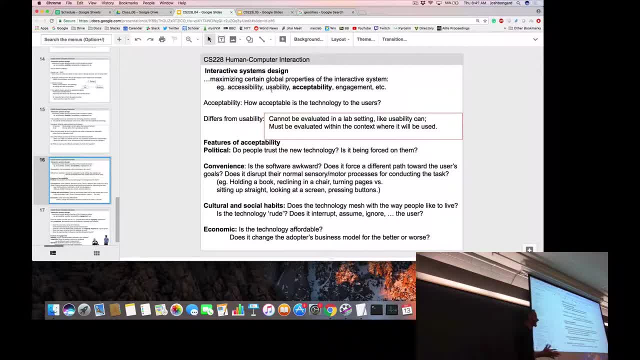 But more devices, more apps, more notifications. Collectively, our society has decided that that's kind of rude right. Generally speaking, it's polite now for us to turn off our notifications, or it's polite for an app, by default, to assume non-aggressive notifications. 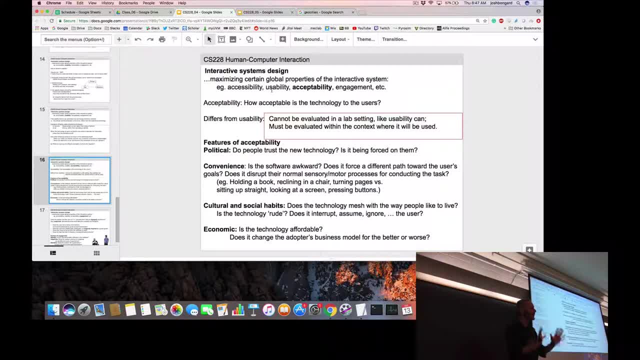 and if we want to ramp it up, okay, right, Again a subtle thing, but an important thing, Maybe a little bit more obvious: Economic aspects of acceptability. Is it affordable? Does it change the adopter's business model, for the better or for worse? 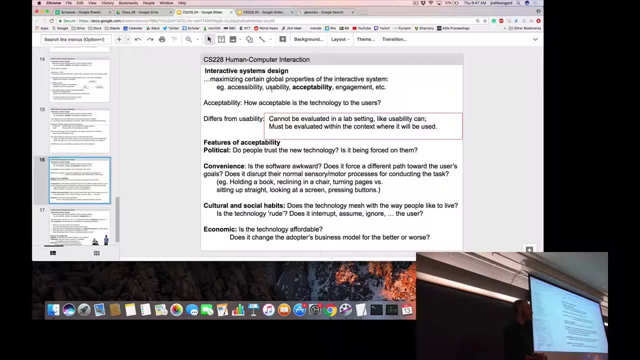 Maybe your software is free, but it's not acceptable because if I do take it on it's gonna start to change other aspects. I'm gonna have to buy add-ons or other things, right? So cultural, economic, sort of ergonomic or convenience, political. 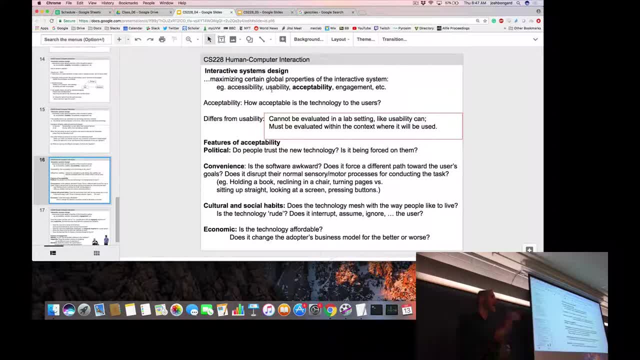 all these other features might take something that you've spent a lot of time getting the interface right. It's beautiful, easy to use, It's usable, not acceptable. Okay, let's move on to the last one: engagement. This is the one that is most subjective. 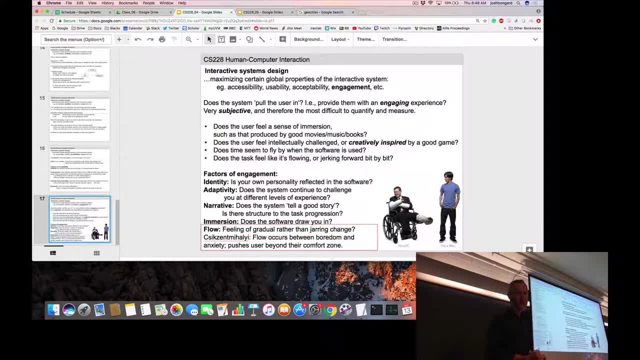 and very, very hard to measure. This is the one that video game designers spend most of their time on, but more and more other kinds of interactive technology designers are also thinking about, which is basically speaking when the user interacts with their system. 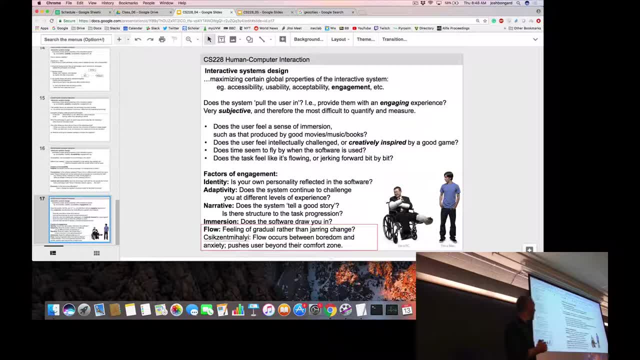 does that system pull the user in? Are they engaged with it? So again, this is very subjective, but you can ask the user: do they feel a sense of immersion? Did they fall into the system like you do into a good movie or a good book? 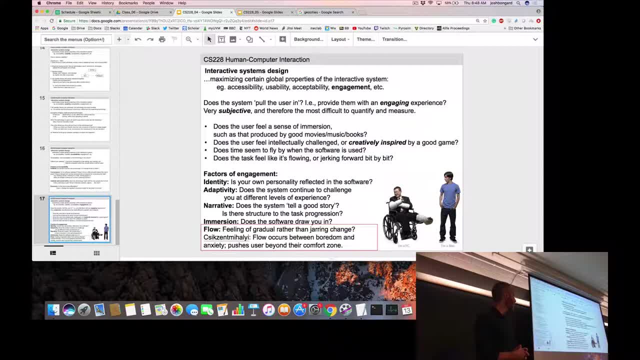 Does the user feel creatively challenged or creatively inspired by a good game or by the system itself? right? So we're gonna talk about adaptive software and your final project is also gonna have to be adaptive As the user gets better and better using the system. 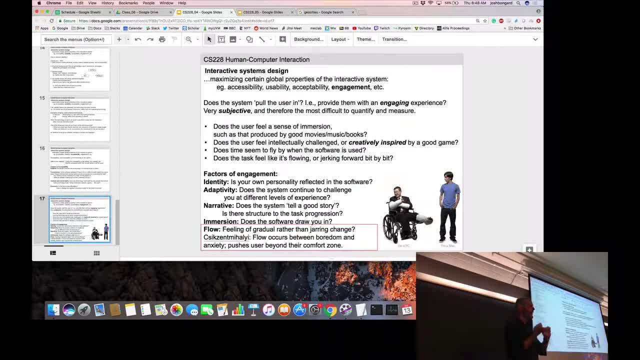 an adaptive system has to infer that the user is getting better and possibly change the interface or change the interaction to keep the user engaged right. There's a very fine line when you're dealing with a game or, in your case, educational software: teaching, ASL. 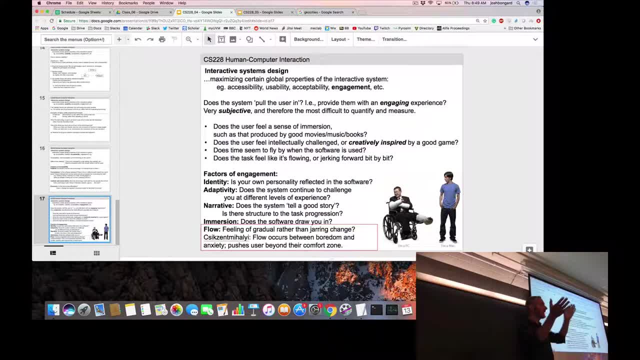 There's a very fine line between boring your user and frustrating your user right? How do you make sure they're in the middle? This is an idea that's been around for quite a while. in psychology, It's now commonly known as flow, after a famous book written by Csikszentmihalyi. 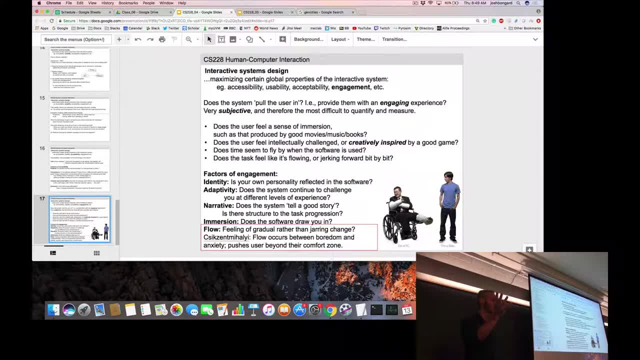 Don't worry, I won't ask you to pronounce that last name on any of the quizzes. It's a great book actually, if you haven't read it. It talks about flow, or optimal experience. So in this book he interviews people at peak performance. 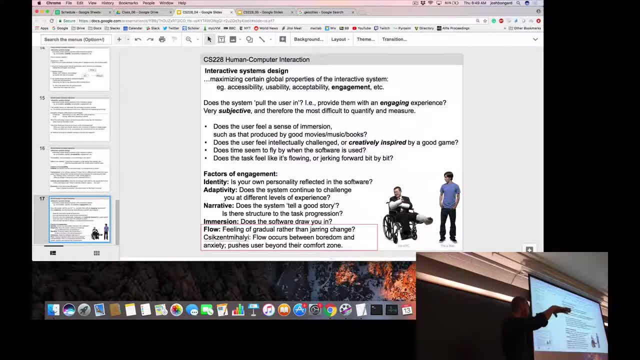 a lot of different domains- sports people, intellectuals, creative types- when they're in the zone- which is another sort of word for this idea. what is their subjective experience? And most people, and you probably have this experience yourself when you're in the zone. 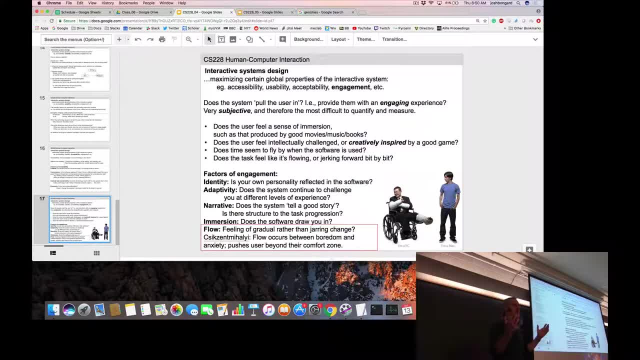 it sort of feels like time slows down. You know exactly what to do next, You don't feel anxious, You know what's happening and you're just flowing through the exercise. There's no effort required, right, If you make a great video game. 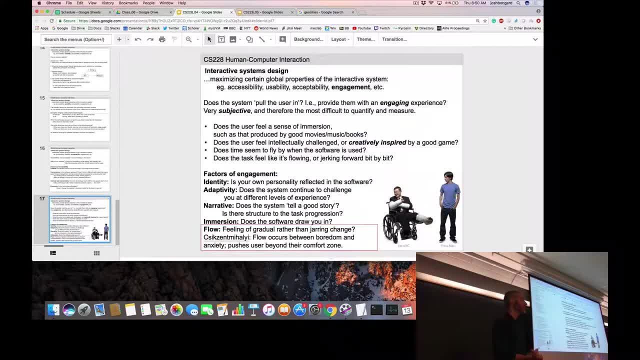 or you make another great immersive experience where you're trying to entertain the user, possibly teach them something, where there is a bit of a challenge there. can you get your users to report a sense of flow right? They may not know what flow is. 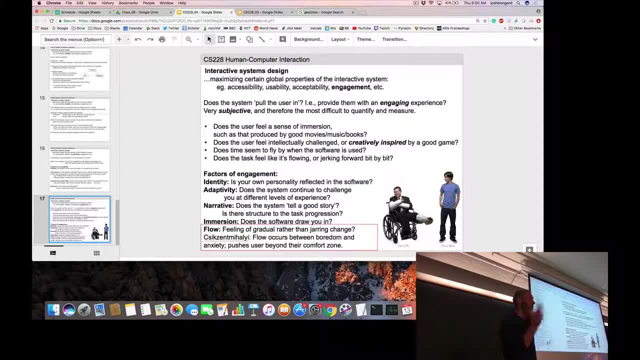 but they might describe some of the features or what it feels like when you're in that optimal experience. right, They were really in sync with the game or with the system. right, It was a real back and forth. It was effortless. A whole bunch of time passed by. 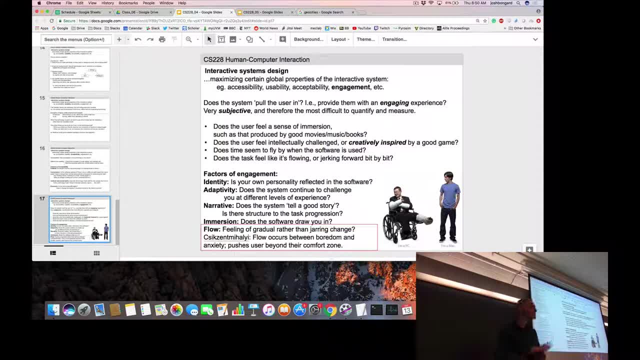 It felt like no time at all. I came away knowing all the 10 numbers of ASL. It was great. It didn't require any effort on my side. On the other side, you know your system isn't engaging if they're frustrated, right? 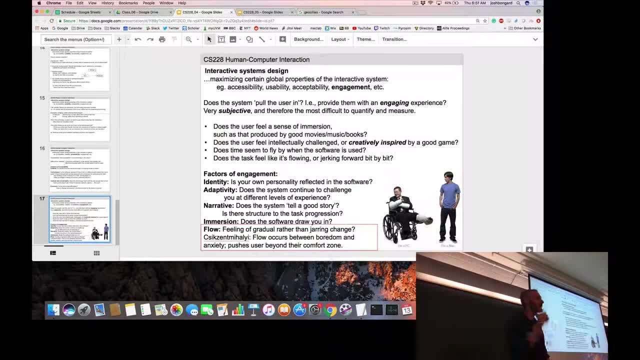 It took a lot of effort to make even a little bit of progress. I had to push against the system to learn just even one of the 10 numbers. It was extremely difficult, Okay. So again, this is a subjective thing. So 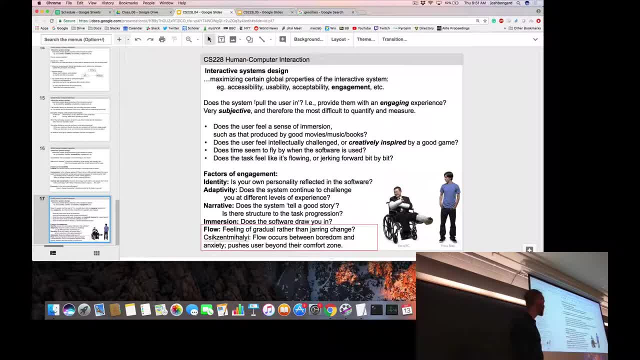 how do we actually try and optimize engagement in our system? Well, again, let's try and unpack this. One of the things that people report in engaging systems is the system sort of matches their identity or their philosophy. They see themselves somehow reflected in the system. 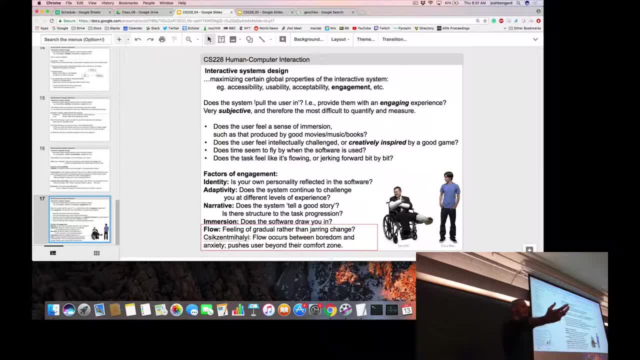 or they see their philosophy reflected in the philosophy of the system. Apple exploited this back in the day with a series of advertisements about I'm a Mac and I'm a PC. Do people remember this? Are they still going right? Which of these two individuals? 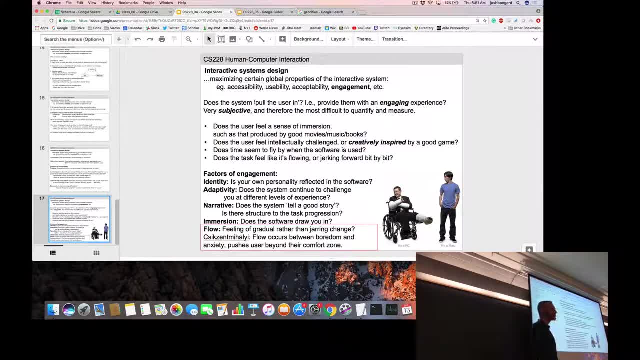 do you want to associate with? Maybe neither, or identify with right. So the Mac over here, right, He's young, good looking, He's always in fashion, He's always relaxed. No problem, We'll figure it out. 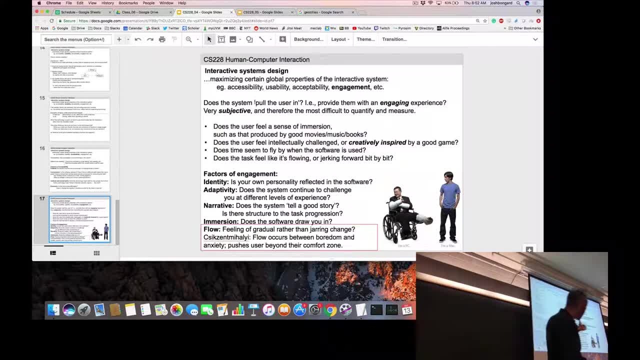 right. The other fellow, unfortunately a PC. He's always in trouble. He's wearing a business suit, right? It implies that Windows machines are just for, you know, office, boring things. You wouldn't use it in your normal life. 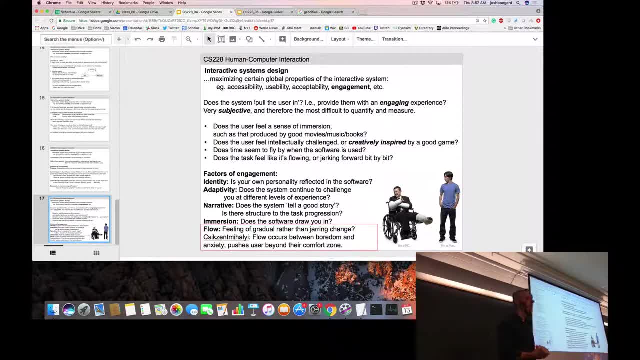 There's a lot of subtle messages hidden in this advertising campaign, but at root, obviously they were exploiting the fact that you might associate with one individual over the other. right Adaptivity: we already talked about this: Can your system adapt and keep up with you? 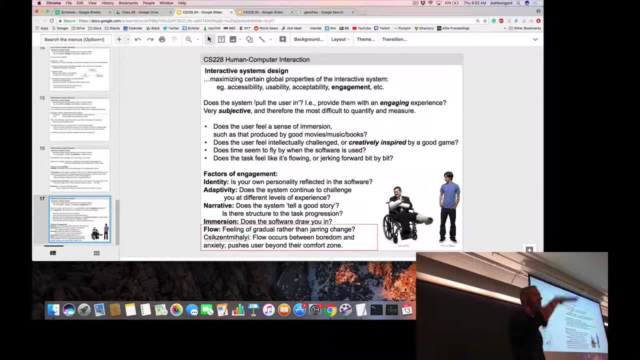 so that you stay at that middle level of feeling challenged. It's not too easy then. it's not too easy that you're bored, not too difficult that you feel frustrated. Does the system tell a good story? right Again, this is important in video games. 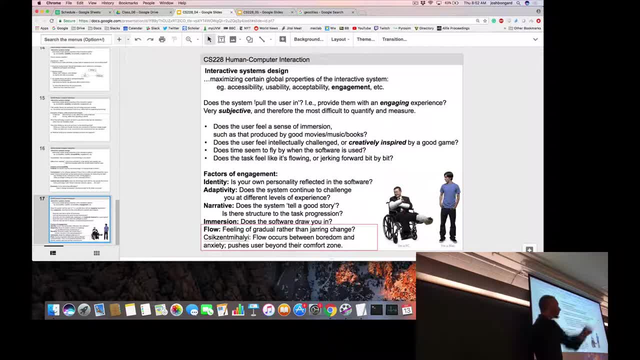 There's a beginning, a middle and an end. There is some sort of goal at the end. As you're interacting with the system, you can clearly tell at any point in time whether you're moving towards the goal or away from the goal. 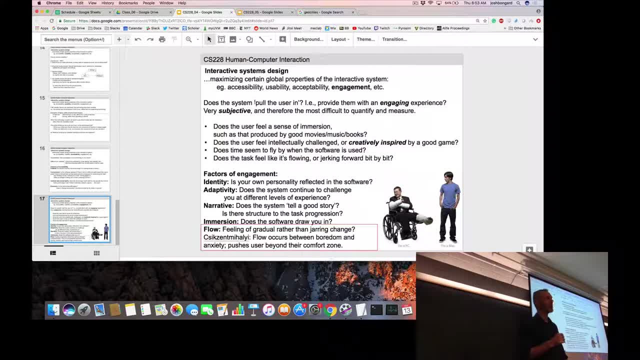 How much further do you need to go to reach your goal, and so on. We'll talk about that more when we talk about navigation and information spaces. Often, when people get frustrated with software, they say they're lost, right, They don't know. 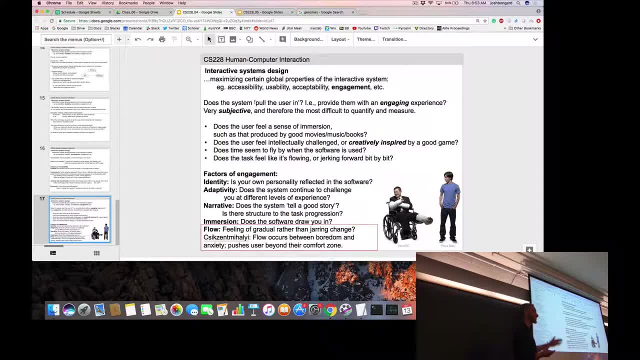 where they are? How do you help people navigate through a complex interaction with a software system? What are some examples of non-video games, other systems, where you've felt this sense of narrative? You can feel yourself moving towards the goal and it's clear. 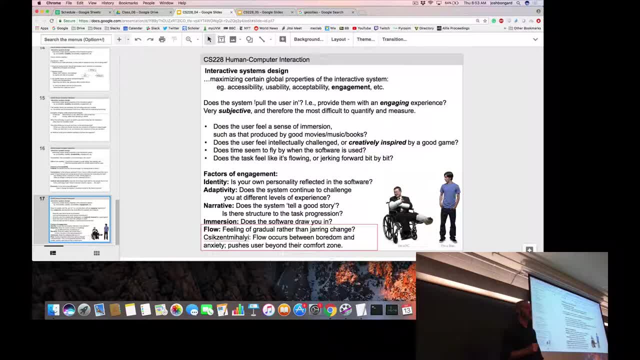 at any point in time, sort of where you are and where you're going. Someone cites Cops and Pigs, and I think that's one of the things that's really important in video games. What are some sort of like section headings at the top? 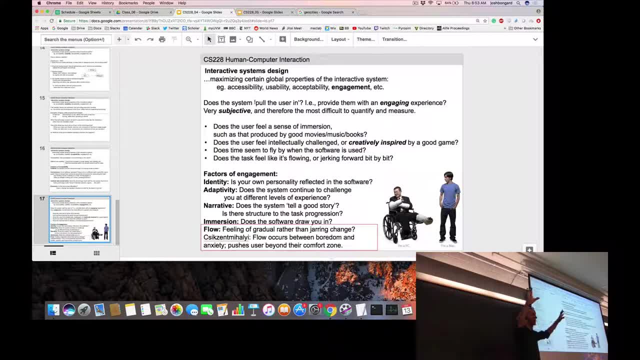 I'll see what you want to see from the column. Okay, so at the top of a website you often see section headings. There may be main pages and subpages. Remember our discussion about the parable of Tempus and Hora. hierarchical organization. 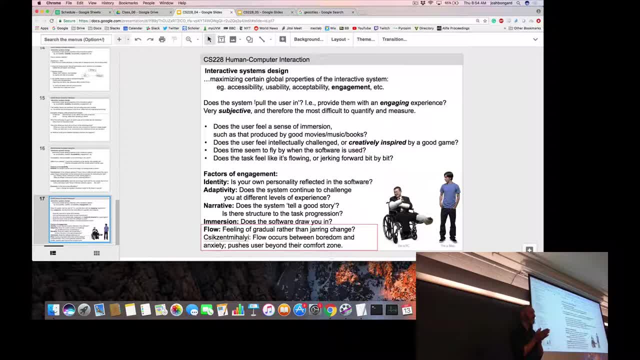 Hopefully, right this moment, you know exactly where you are in this course. We're in Theme 2.. We're in the second lecture of Theme 2.. We're at the end of the sec- we're reaching where we're going. Lecture 5 is next. 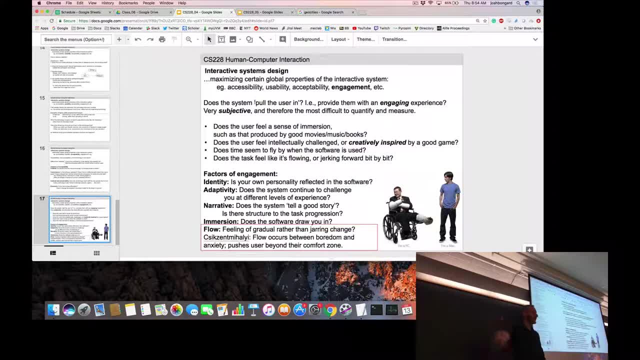 and you know, next week we're going to reach some new theme, and so on and so forth. What are some other examples of technology that provide that feeling of narrative? I was going to say filling out the FAFSA form, I don't know. 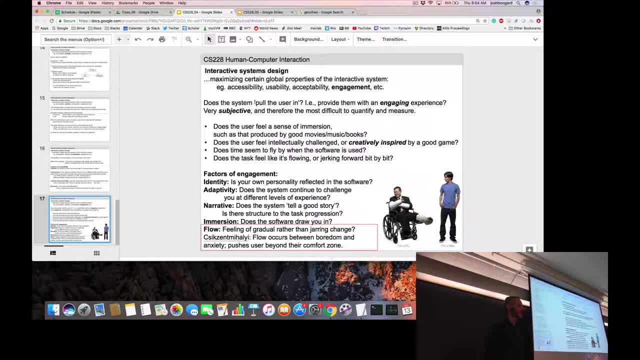 what that is. Tell us a little bit more about that. It's a federal aid form and like it's called Principal Modularity and like if you keep, you have to like fill out the form at the end of the project. Gotcha, right. 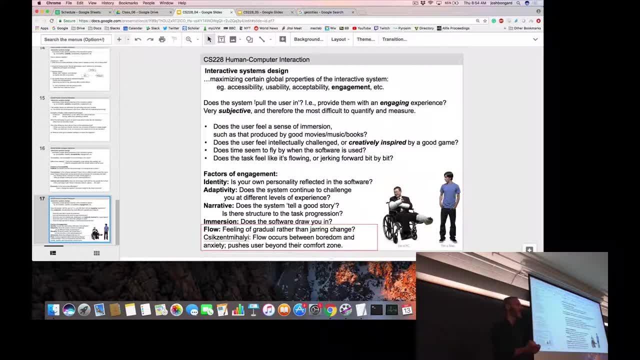 So filling out complex forms on the internet it's a lovely experience, right? So luckily people have started to figure out how to make this a little bit easier so you don't get lost filling out a complex form. I hope, filling out all of the steps. 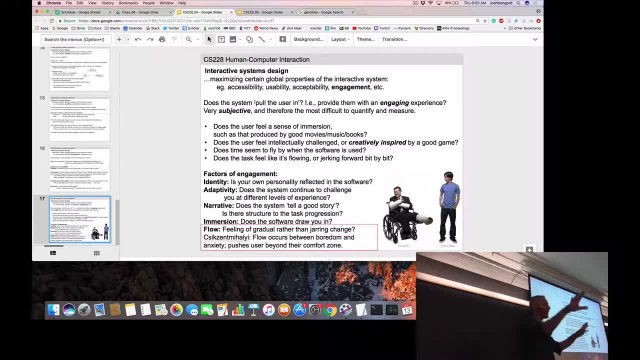 in the deliverables is not too confusing. I know sometimes there's 18 D-I and so on: Go here, go there and so on. right, So when you're performing a complex task which has got a lot of moving pieces, you might not be able. 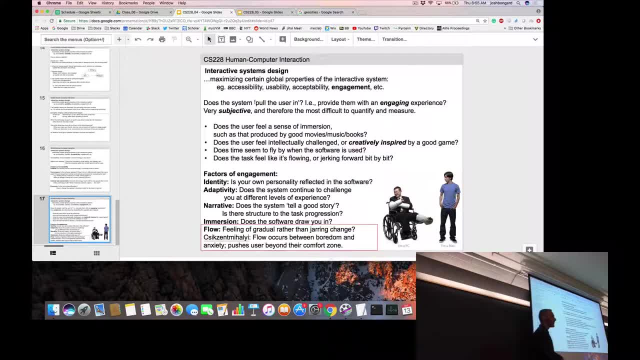 to do it all in one go. This idea of hierarchical design is very useful in helping people understand the narrative and where things are going Okay. immersion again subjective. does it draw you in right? I'm sure you've all had the experience of reading a great book. 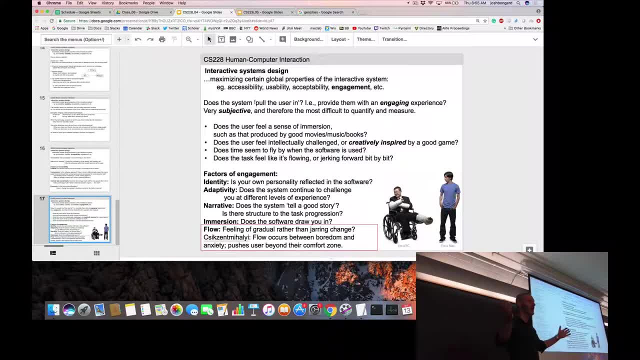 or watching a great movie and you just get lost in it. You forget everything else that's going on. It's kind of technologies where you've had that experience Again. video games is kind of an obvious example. but what about other systems? VR, right? 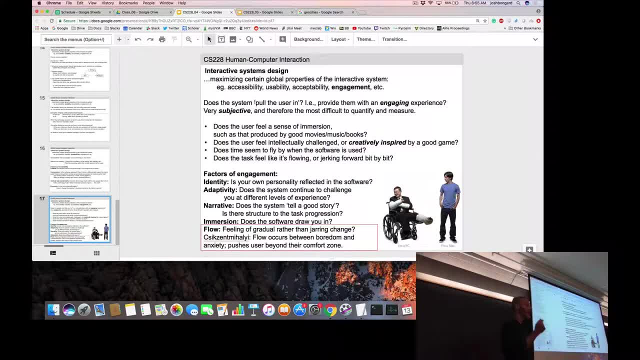 This is going to be the ultimate in immersion, if they get this right. and again, it's interesting that VR has taken so long until just recently that they're starting to get it right. right, This was VR was promoted as the killer app in the 70s. 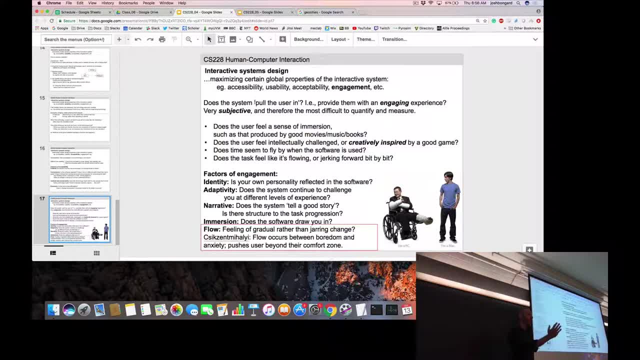 It wasn't The 80s. okay, the 80s is going to be the 90s, 90s, the zeros. we'll see right Or 2018.. We're still, maybe almost there. We're going to spend. 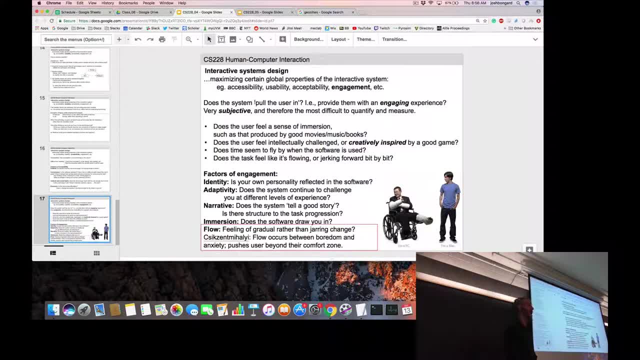 a fair bit of time at the end of the course talking about virtual reality and why it's so difficult. Obviously there are the technical challenges: right, Real time, I need to keep track of head motion and all that. Why else is it so difficult? 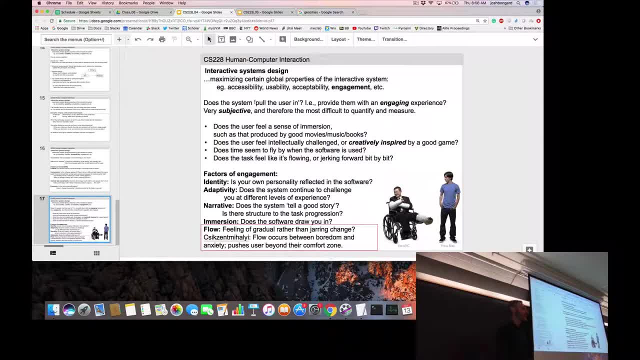 to get immersion right with VR technology, Because you can't really do the whole moving around thing unless you have a large enough room. Ah, you can't do the whole moving around part unless you have a big enough room. That was true, And again, 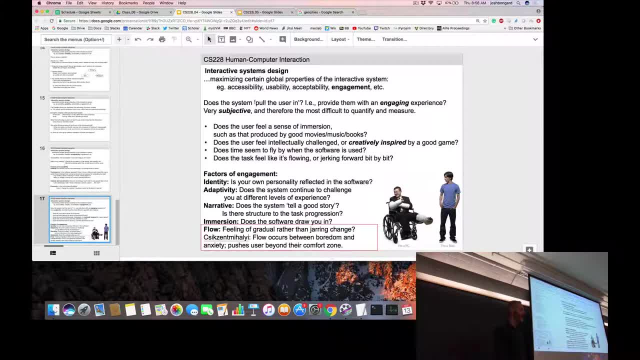 we're going to talk about that. right, You can't move and do VR at the same time, Or can you? What's the solution other than having a huge room? Anybody know Those omnidirectional treadmills- Omnidirectional. 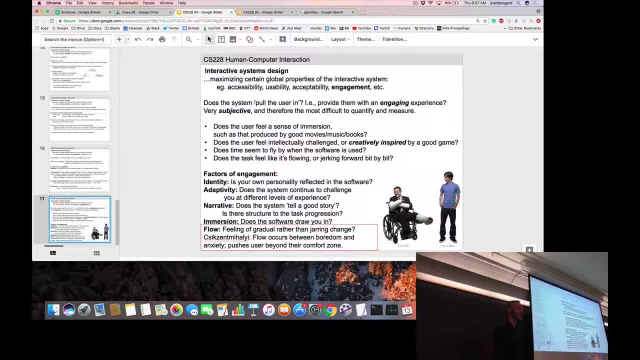 treadmills is one possible solution. We'll look at that right. So remember, at the beginning of the course we talked about humans. They take input, sensory input, They cogitate and produce output. But remember our discussion about John Dewey. 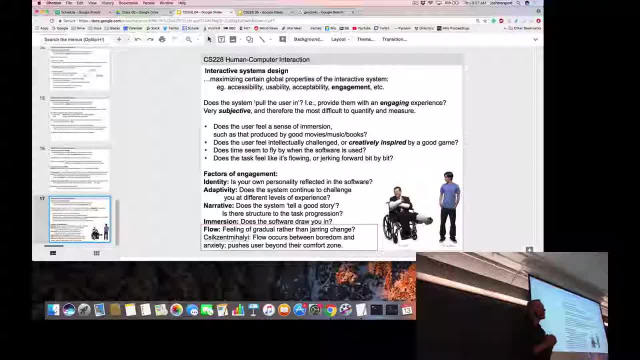 who tried to invert that whole process And Dewey said: we push against the world first. That's the primary thing. If you don't know what to do, somebody who doesn't know what to do with leap motion, they can sit there and look at it. 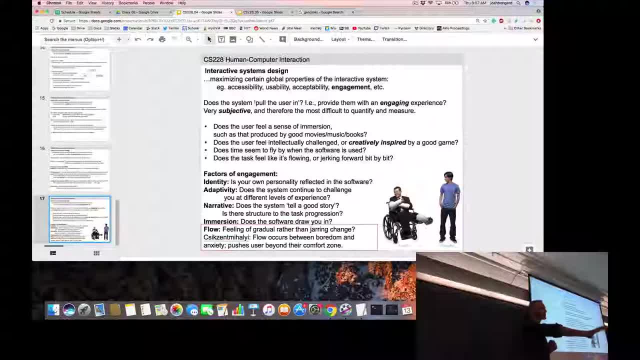 all they want, Nothing's going to happen. Most people will do something like this: or tap it or pick it up or shake it. They'll interact with it and that's how it pushes back. So when I push against the world with my legs, 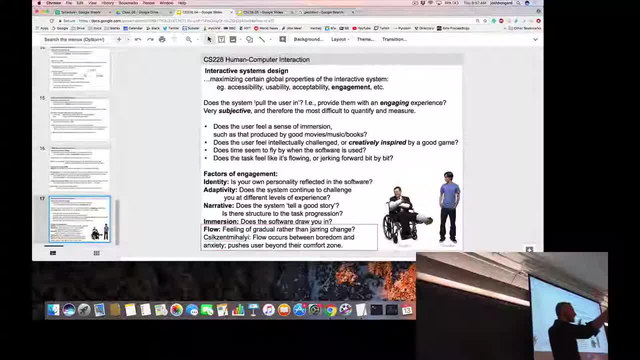 and feet. there are particular kinds of sensory repercussions that I expect when I'm walking. So either I need a big room or I need an omnidirectional treadmill, which again is tricky For those of you that run on non-omnidirectional. 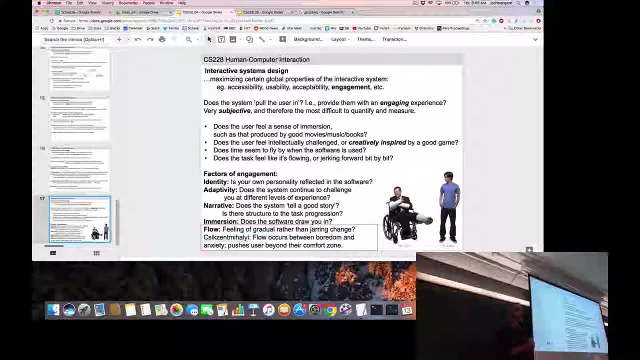 treadmills: have you ever been at the gym and you run on a treadmill for a while and then you step off the treadmill? why? Something to do with the physics of your body. It has absolutely something to do with the physics of your body. 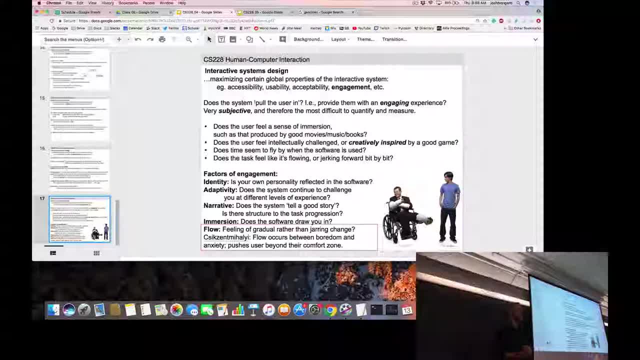 and also your brain. Remember, the brain is a prediction machine, so there's a mismatch there that's going on. that makes you dizzy for a few seconds. You're expecting the ground to keep moving. You're expecting the ground to keep moving to some degree. 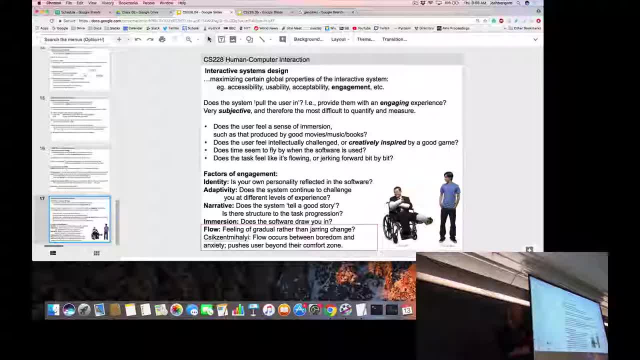 It's not actually that so much. We're getting really close, though, but it is expectation. so if you step off the treadmill, your brain is expecting something and it doesn't happen. What is it Not really? So if you run right? 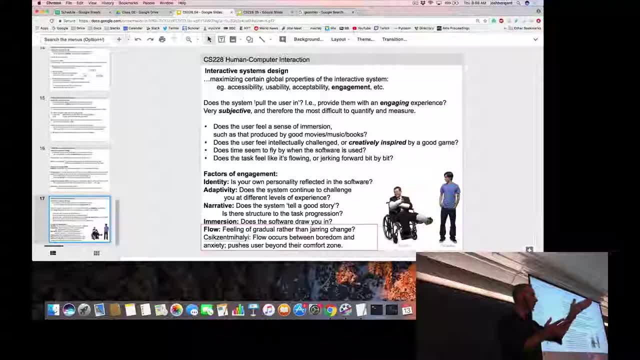 you're moving and even if you stop running without a treadmill, you don't have this experience. So it's not that your brain is used to your legs moving and then your legs stopping. It's not just the motor system, right? Remember? 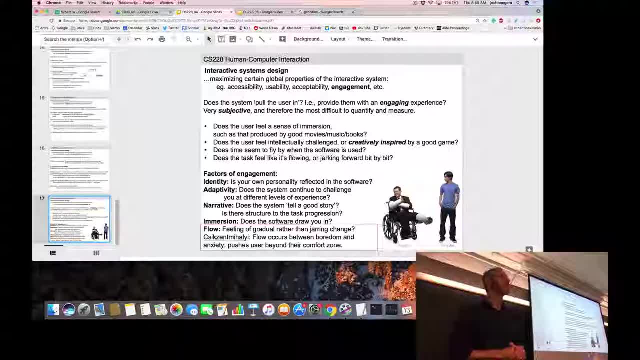 if you step off the treadmill, you're expecting the ground to keep moving, and it doesn't happen. Exactly right. So you before you for all the years that you've been around, before you ever step on a treadmill for the first time- 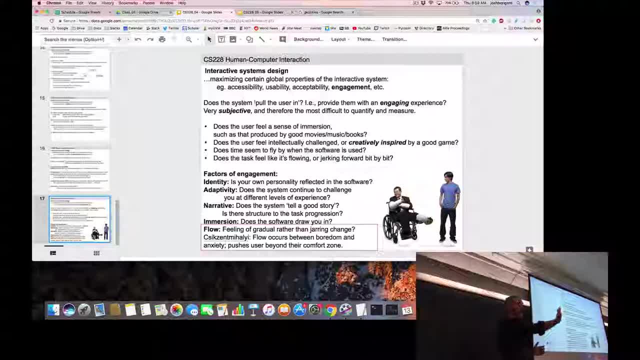 your experience has always been: when you move, the world moves in the opposite direction, right, Always. It's so clear. Your brain builds up that prediction When you step on a treadmill. a treadmill is weird in lots of other ways. So your body. 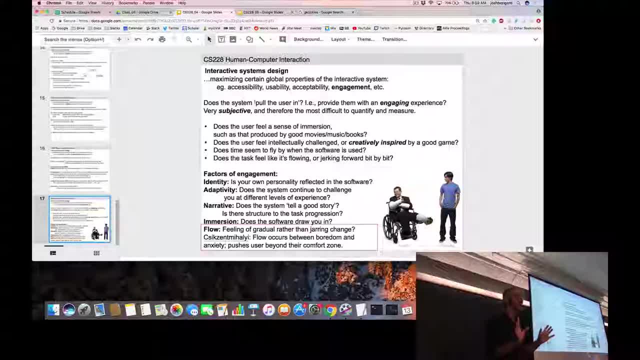 is feeling that you're now on something that's very different. So your brain is now already prepared to deal with things that are going to break its prediction. So often you're not as dizzy when you start running on a treadmill. Your brain says: 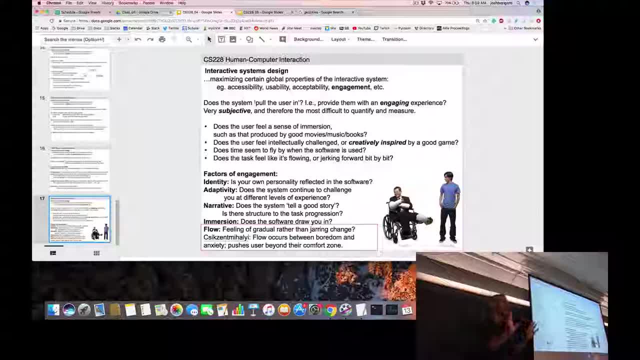 okay, something weird is happening, all right. So your brain says, okay, I'm in a weird situation now where I have the experience of running. the world is not moving. Okay, you're on the treadmill and your brain builds up a prediction. 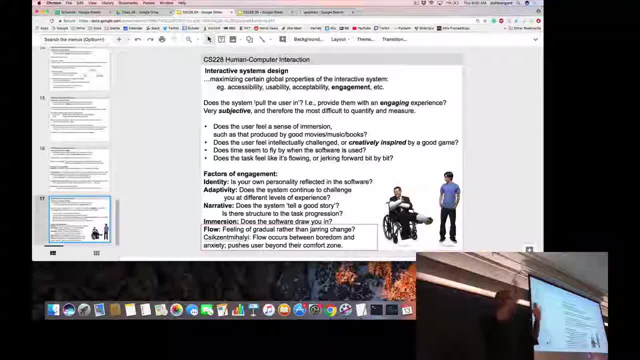 during that period that as you run, the world doesn't move and says, aha, I know the new situation. Then you step off back into real, the real world, and suddenly that prediction which is built up over the last half hour is broken. 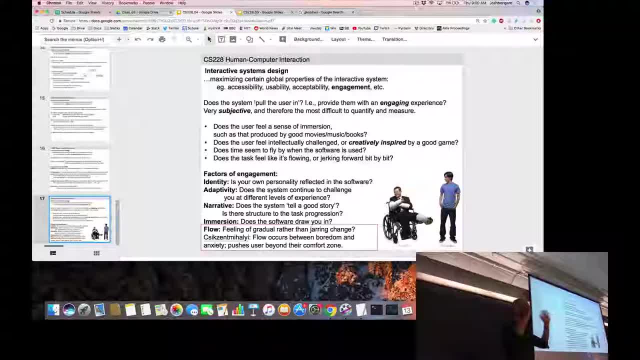 and you feel dizzy for a second or two until your brain says: actually, now I remember this is normal, not the treadmill. Okay, So again with VR. unfortunately, even with a lot of sophisticated technology, we're interacting or perturbing. 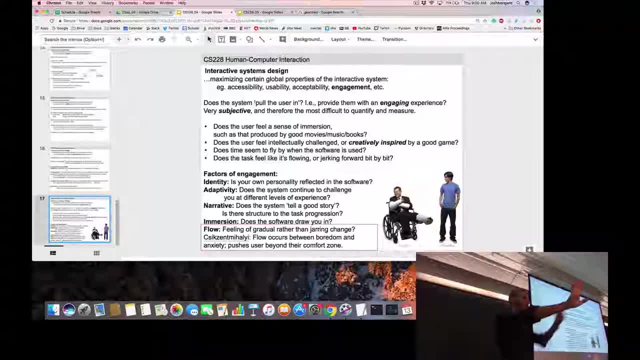 all of those sensor, motor sensor feedback loops and the predictions your brain has about sensory repercussions for actions. One of the reasons that VR did not work in the 90s and the zeros is that, even as the headsets were getting better and better, 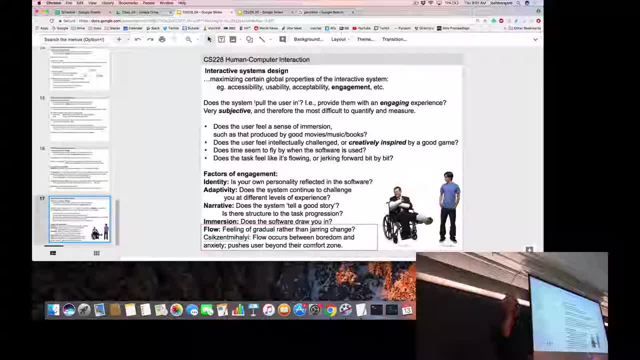 as someone wearing the headset moved their head. what they saw was correct in the sense that it would move in opposition to the movement or, sorry, it moves with your head. What you saw moved with your head. That was right. but there was something else. 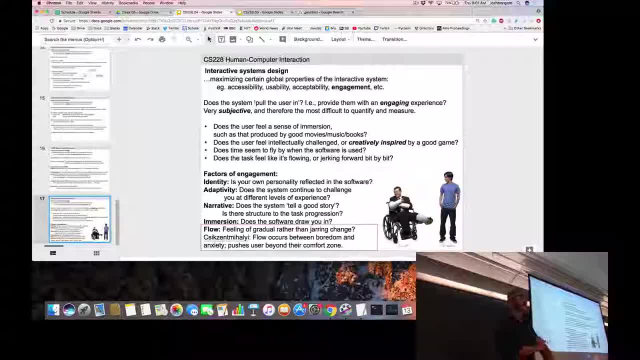 that was still wrong. that actually made people nauseous when they wore these headsets. So when you're moving your head like that, you expect to see a different part of the world, but you're seeing the same part with the headset. That's true. 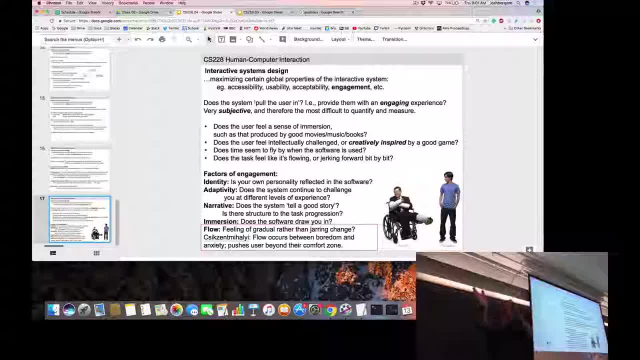 but again, that all got worked out relatively early on, right? So whatever the virtual world was that you were looking at, the right part of the world would come into view as you turned your head, but still people were getting nauseous or dizzy. 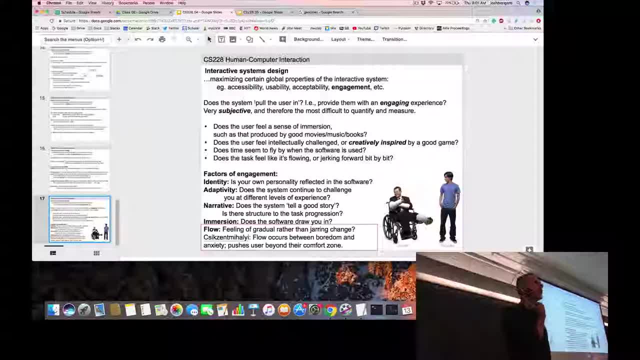 because it wasn't moving fast enough, right? So in the 90s they got it down to a tenth of a second. In the 2000s, a hundredth of a second wasn't enough, right? You know that when you move. 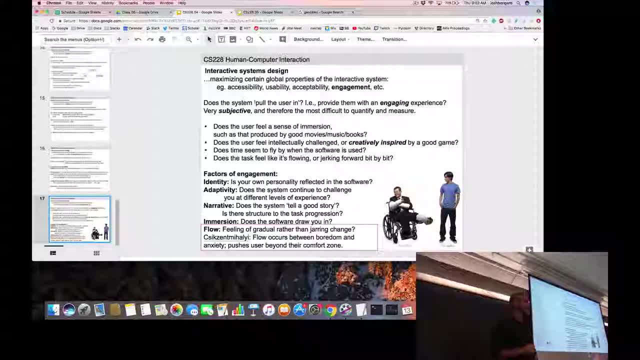 your head. the visual repercussion of that movement is instantaneous, and any light of a lag is extremely disconcerting, right. So it's only now that our computer technology is fast enough. There is still a lag, but it's small enough for most people. 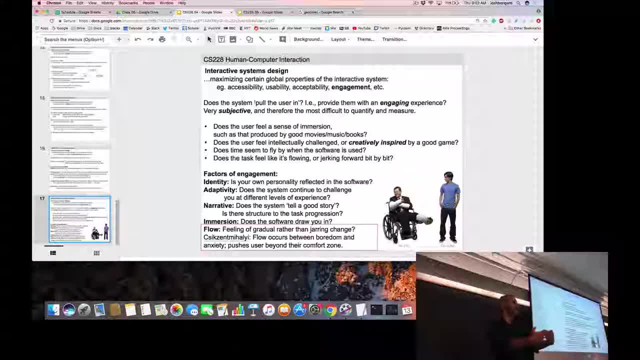 not to be able to detect it, and that seems to be the main barrier that we've finally gotten over: that people wearing VR or their brains can deal with all the other broken expectations, like when I'm walking. it's not quite right, but generally speaking, 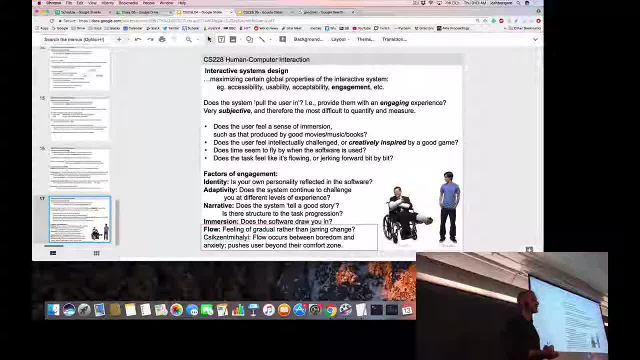 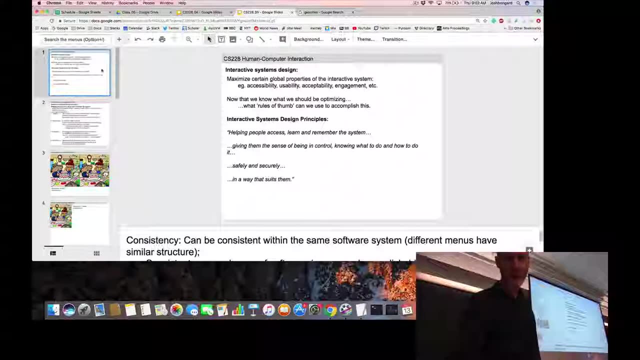 when I do this, the world responds appropriately: Okay, Okay. So I think that finishes our lecture on interactive systems design as it relates to these non-functional requirements. Let's move on now to design principles and, as you'll remember from last time, 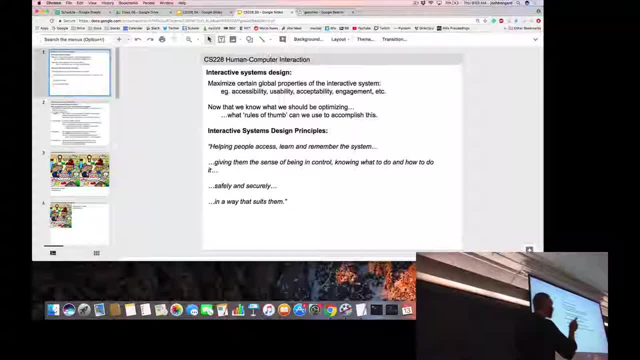 as you remember from last time, design principles are kind of these rules of thumb right, So we kind of know what we're doing now. We want to design accessible, usable, acceptable and engaging. How do we do it? What are the rules? 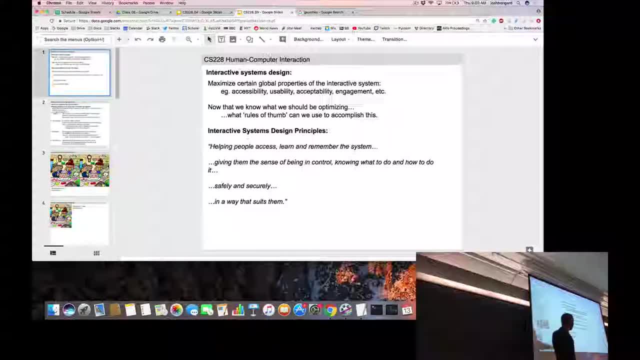 of thumb that will help us to do that. Unfortunately, in the book it gives you again a long sentence with a lot of vagaries in it. We'll try and unpack this. Generally speaking, these design principles are going to help people access. 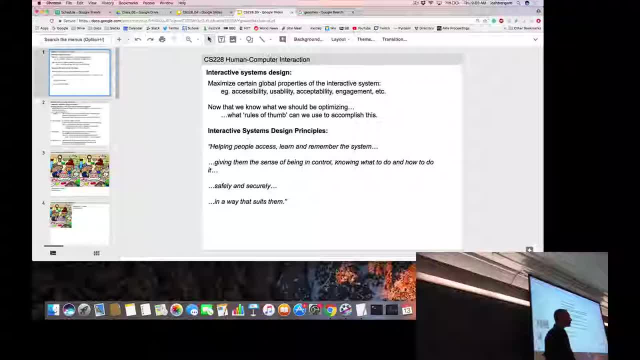 learn and remember the system. We've mentioned that before Giving them the sense of being in control- This is important: Knowing what to do to save time safely and securely in a way that suits them Kind of vague. So again, let's try and unpack. 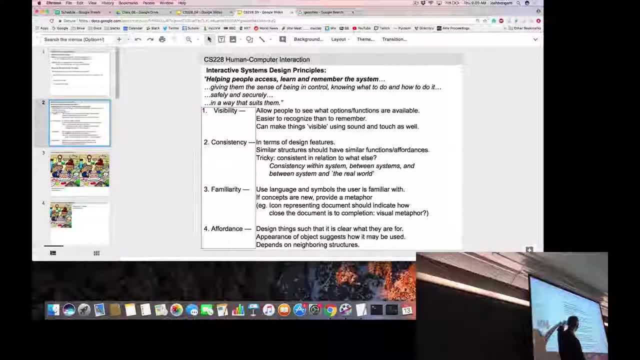 these into a few design principles, So we're going to try and maximize these aspects now. The first one is going to be visibility, So we need to make sure that people can see or hear or know somehow what options and functions are available to them. 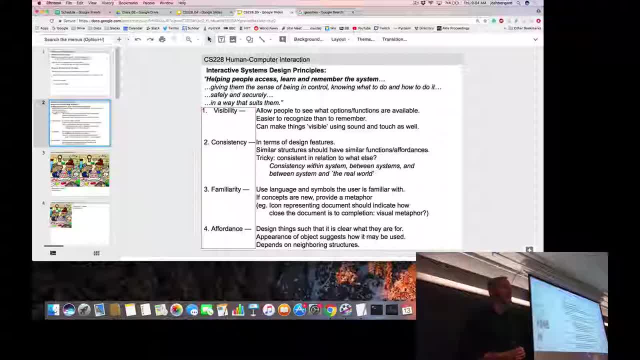 And our first design principle here is that we're going to try and make things recognizable rather than memorable. We mentioned memory is important, but it would be great if people don't have to remember a whole bunch of things to use your system. So we want: 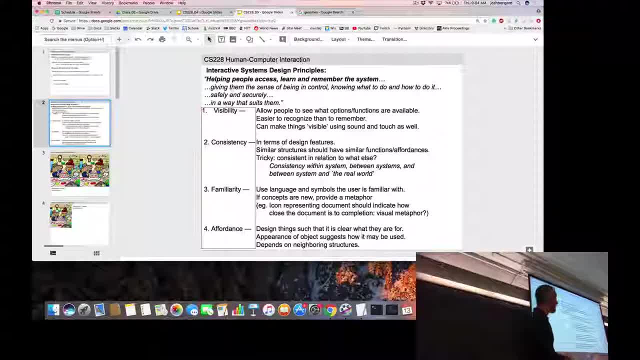 to make things visible so that they can sort of see what's going on. This one's tricky, however, because we don't want to put too much visual or auditory clutter in front of our users. Remember, keep it simple, stupid Lots of pop ups. 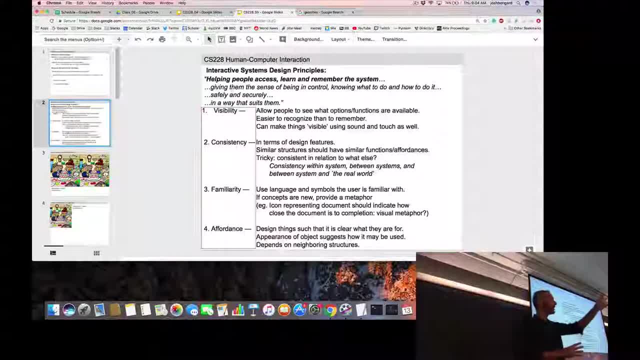 and notifications and suddenly there's an alarm bell or a ding. I want them. you want your users to focus on what's happening, but you also want them to be able to recognize things. So how would we possibly make more things visible without adding more ink? 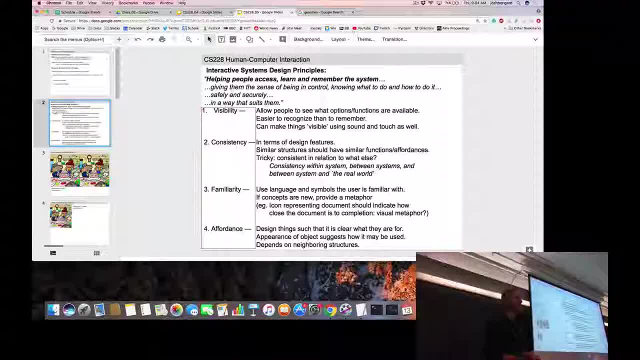 Remember, we want to maximize the data to ink ratio. We want to use as little ink, as little flashing fonts and different colors and things moving on the screen as possible, yet make things more visible Seems kind of almost impossible In the next theme of this course. 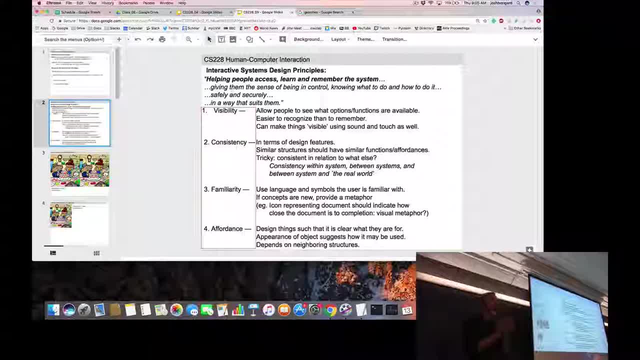 we're going to talk about cognitive psychology and people, and also aspects of our visual system. There are aspects of our visual system that we can exploit to make more things visible without having to add more ink. Here's a very technical drawing to make this point here. 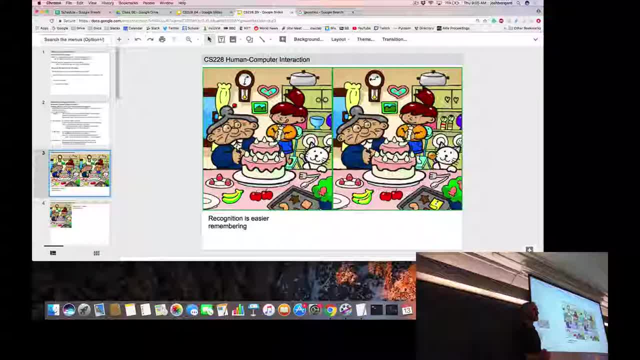 You probably all played this game before. How many differences are there between these two pictures? I'll give you a minute to figure it out. See how many you can find and count them. I'm going to ask you how many you found, not what they are. 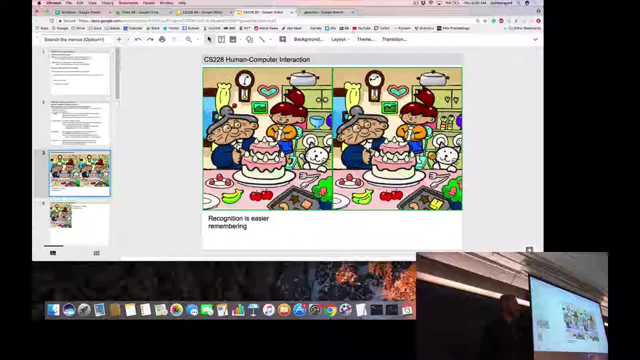 How many? Ten- Anybody find more than ten. Twelve: Anybody find more than twelve. You have fourteen. Oh, not bad. Okay, you guys are awake this morning. Okay, Here is exactly the same picture. How many? 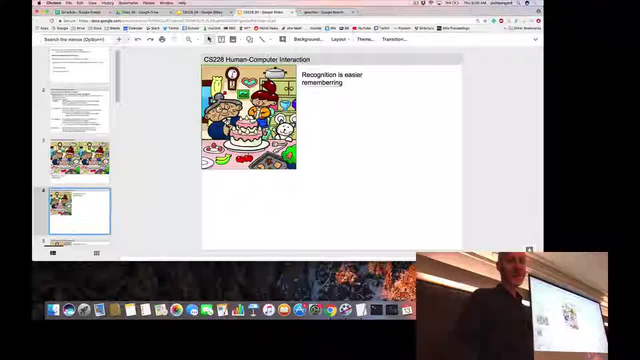 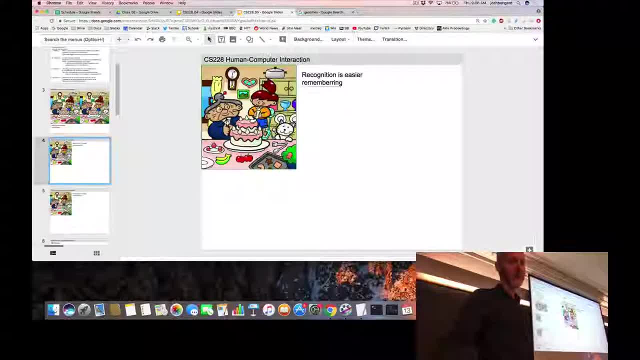 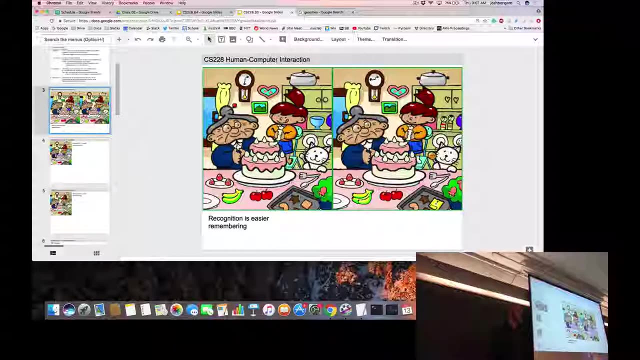 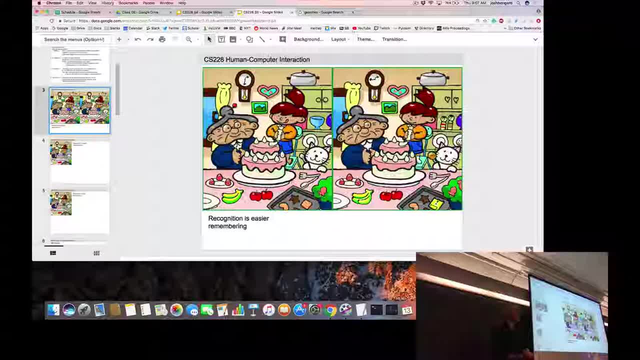 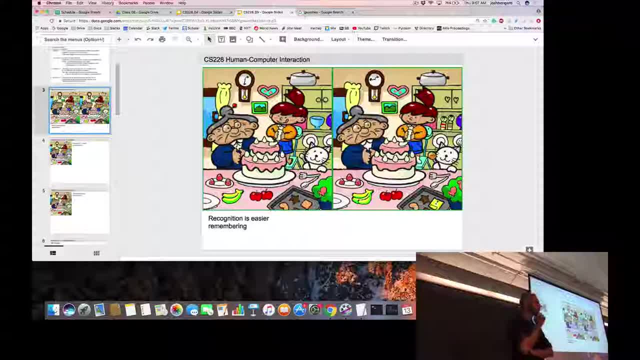 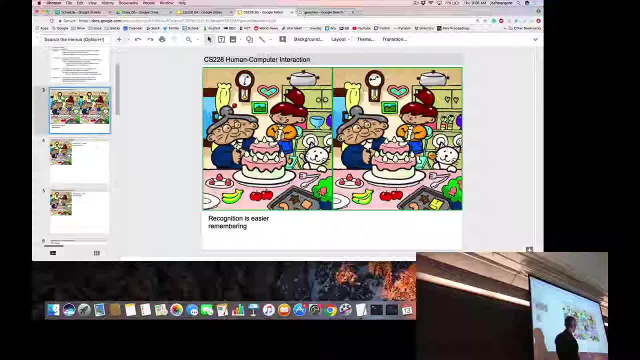 to the next, you might see this and you see three strawberries. you know they always add or remove a strawberry, right. so you're looking at this and if you look at this, this is actually still in your visual field, but it's off to the edge, and the edge of your visual field is not very good at detail, or 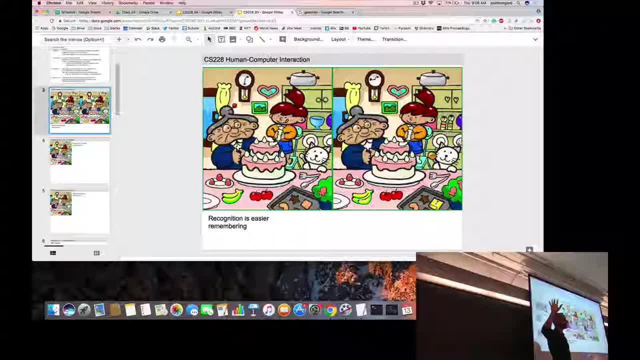 counting. you know that there are strawberries over here in your visual field, but you can't count the number of strawberries in the right hand image until your eyes move, your saccade, your eyes jump and your brain is a prediction machine. it remembers and you got to store this piece of information. 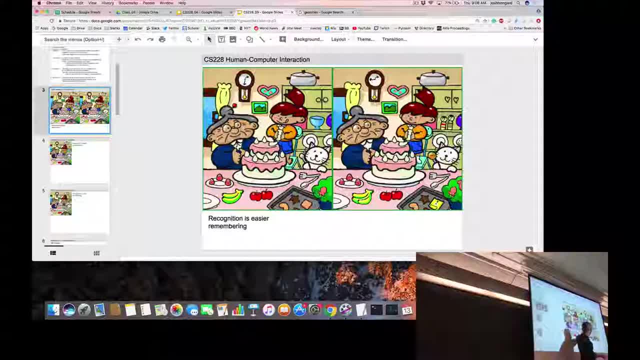 you got to remember that there were three strawberries there. and okay, there's three strawberries there that didn't remove a strawberry in this, this case. right, so there is a sensor motor loop going on here. you're pushing against the world and observing how the world pushes back. 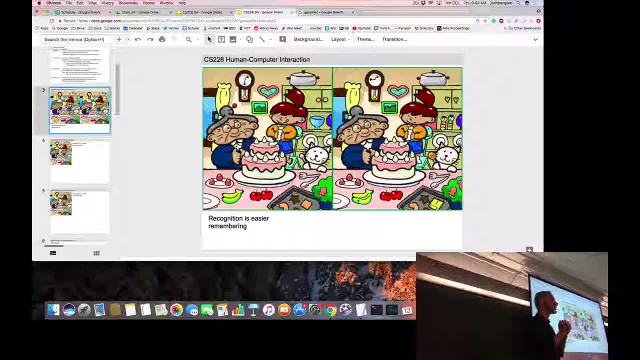 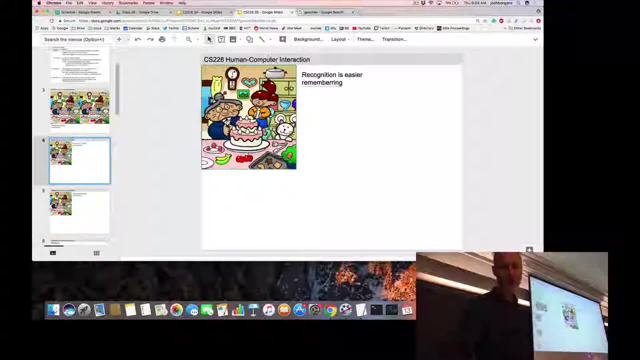 you're pushing, in this case by moving the, by using the muscles in your eyes to move your eyes, and you're seeing how the world pushes back. are there three or four strawberries when you land on the, when your eyes land there, on the second image, and you got to remember how many there are if you look at the strawberries. 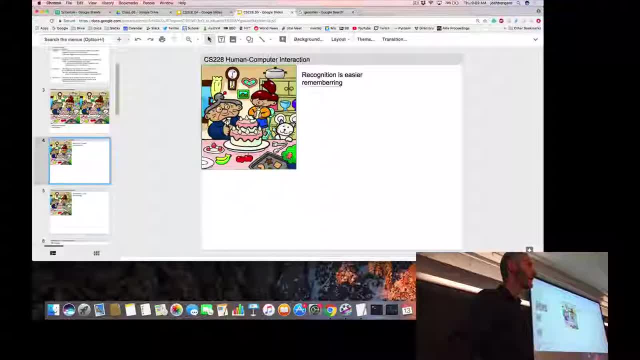 here. if you're looking at the strawberries, you don't need to count that there's three. the motion part of your visual system just reports no motion, which equals no change. right, Pretty easy. Okay, the number of strawberries is easy. The shape of the frosting on the bottom layer of the cake not so easy to see. It's possible. 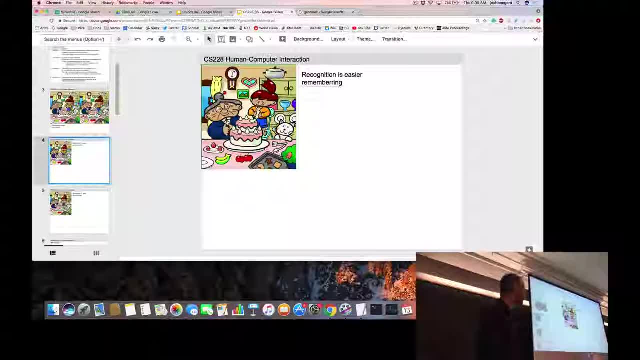 but difficult, right, Okay? so obviously this is a bit of a cartoon example here, but this principle of exploiting some aspect of the human visual system, which is that we can use motion as a metaphor for change, or there's a, not a. I guess it's a visual metaphor. 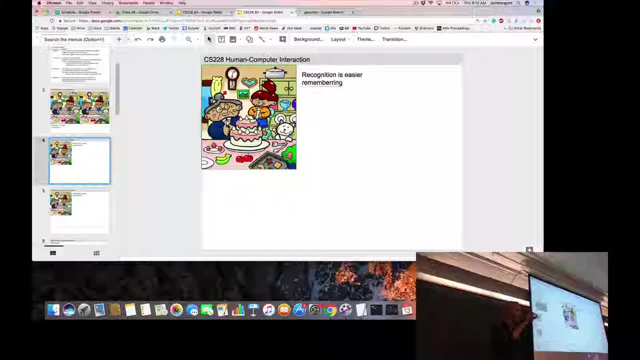 but it's also sort of an animation metaphor here. Movement equals change. That's important, right. We can exploit that. This system is actually used by certain security companies to detect Trojan horses. So when new computer circuits or electronics are designed in the 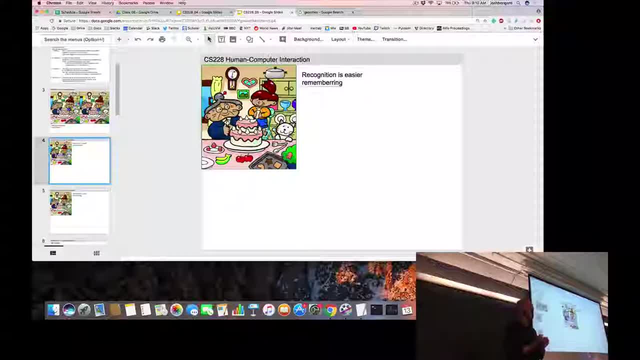 United States. those designs are often sent to another country where they're manufactured and in some cases, where they're being manufactured, a black hat in that country or in that factory will introduce a change to the electronics that is very small and very subtle. 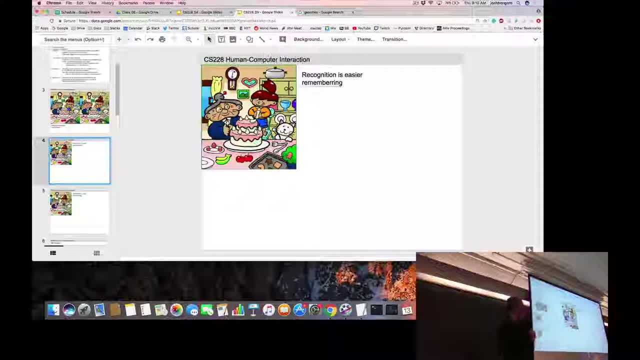 so that when the electronics comes back and is incorporated into a weapon system, for example for the military, unbeknownst to the designers of the chip and the people that install the electronics into a weapon system that there's now a backdoor in that. 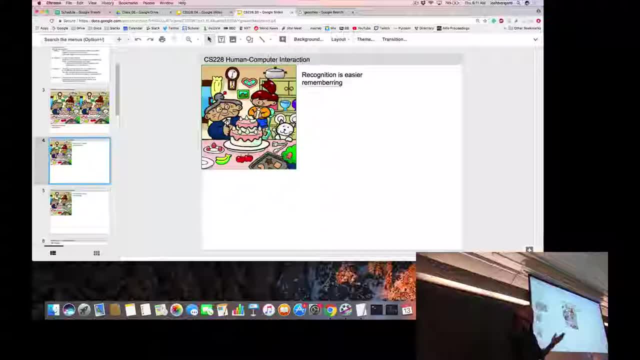 that circuit. So how do you know that the manufactured circuit, when it comes back, matches exactly the design specifications of that circuit? It's tricky. Sometimes the Trojan horse is purely software. That's obviously hard to find, But sometimes there is a very 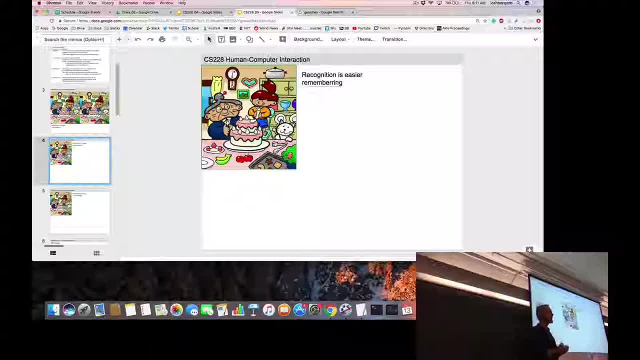 very minute change in hardware that is very, very difficult to detect. What's the easiest thing to do is to take very careful still photographs of all of the circuits that are coming back, match them up and play this game And sometimes, if you see a subtle change, 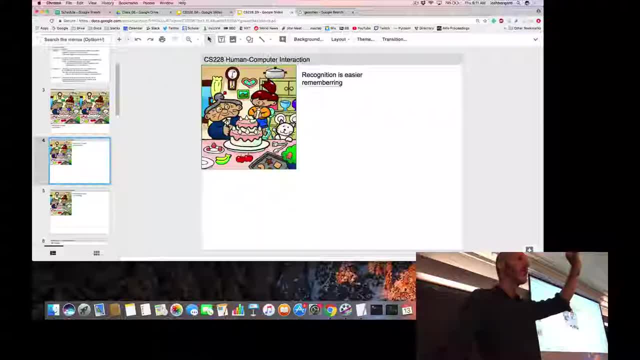 this particular diode is sitting here, but now it's off a couple nanometers compared to another chip. that is often a good telltale, for interference Doesn't always work, but again sort of a simple trick applied to a very, very important and serious problem. Okay, It's taken. 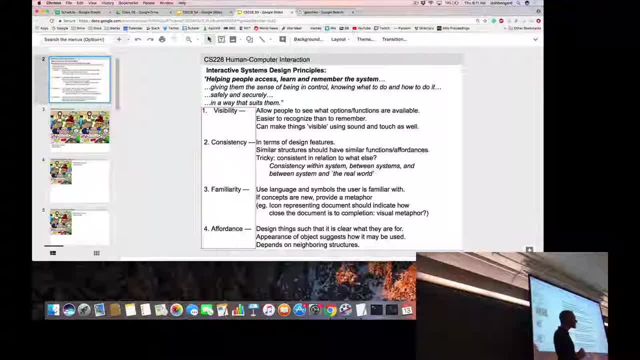 us a little bit away from HDI, but I think you get that Consistency is important Across all the pages in your website or across all the parts of your app, or if you work for a company that develops multiple apps, you might have. 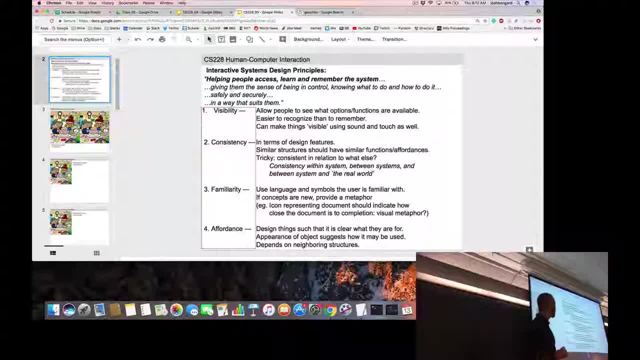 a common sort of style or consistency across apps. Sometimes, again, this is obvious, so that might be visual consistency. Everything in your system is a particular shade of blue, never a particular shade of green. That's an easy one, But sometimes you want the consistency. 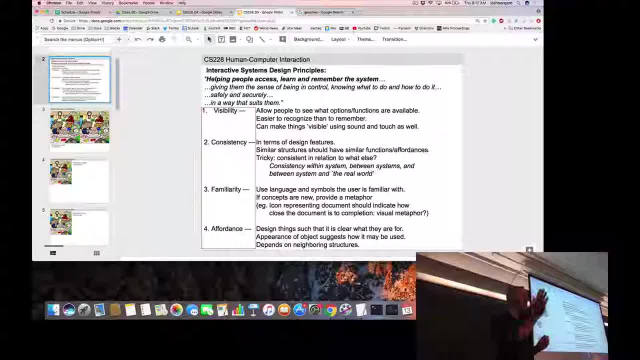 to be cognitive right. You want sort of the brain, which is a prediction machine, to sort of know that the way in which you interact with this system across different parts of the system are consistent. Consistency might be within the same system, between different systems or, as we've 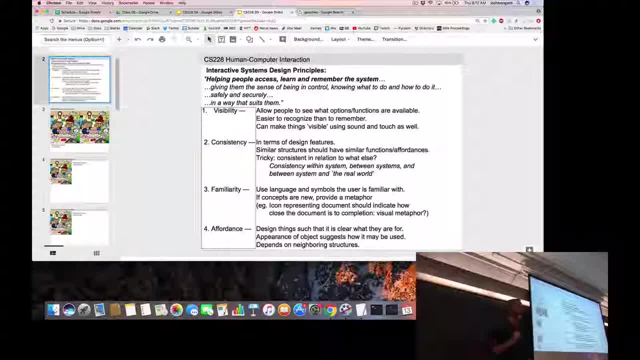 talked about with metaphors before, between the system and the real world. What are some aspects of cognitive consistency, Consistency that you know of in apps or websites or other kinds of software? Using like a floppy disk symbol as a save- Okay, Using a floppy disk symbol as a save right. We talked about that before- as metaphors. 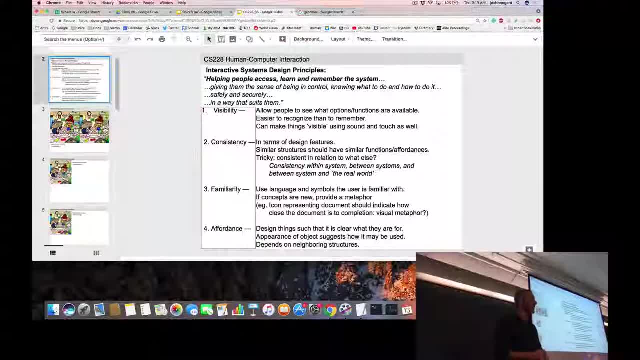 If you want to have a little icon for save in your system, it's often a floppy disk. How many of you have actually used floppy disks? A couple of you. Oh, wow, Great, Okay, Good to know, Awesome, All right, Someday no one will put up their hand, but for now I'm going to give you a. 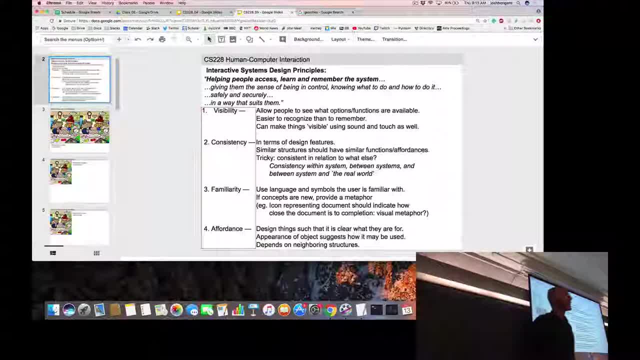 couple of examples: Arlo, Can you say that again? Windows Explorer, Windows Explorer, Exactly Right, It looks like an actual paper file or a folder. The very idea of folders and files, right? This was a metaphor invented right at the beginning of the computer age. 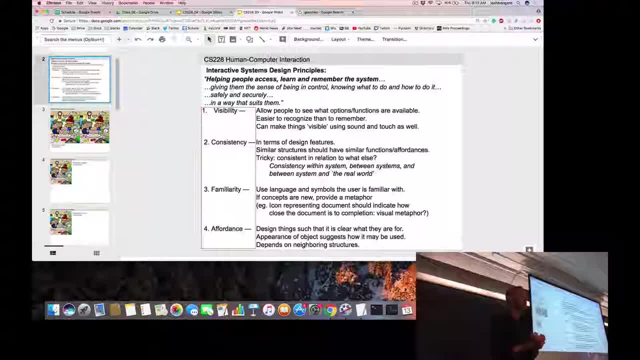 when GUIs or graphical user interfaces were introduced And they're kind of universal Right. Imagine you created a new system where people needed to store information and retrieve it and you use something other than files and folders. That would be very jarring You. 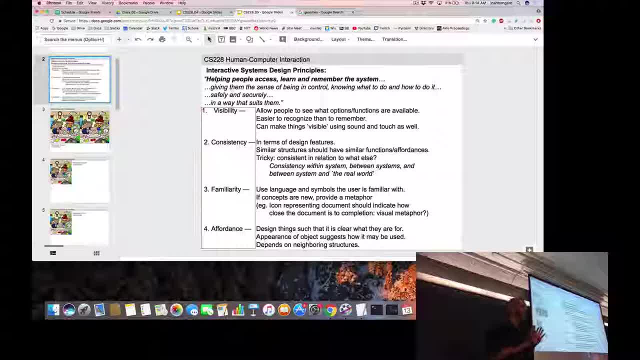 better have a very good reason for breaking that expectation that in your system things are being saved and loaded back from files And those files, or that information is hierarchically organized in folders. Yes, Looking for the settings button, Absolutely Right. 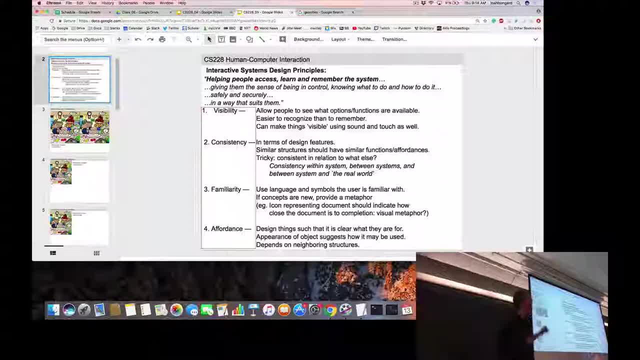 So where things are to be found. Again, that comes back to navigation Right. Where are the settings on this? I always know they're top left somewhere Or top right, depending. Right Depends on the program. Depends on the program, Right, If I see that little circular gear right, that in the top. 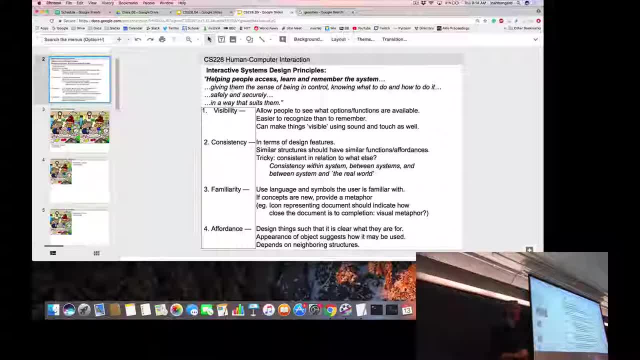 right, that's usually settings. Okay, Let's carry on. So again, familiarity: Some of these are obviously related: Use language and symbols that the user is familiar with. And again, if you have to introduce a concept that's not familiar to your users, like the fact that you're going to save information, 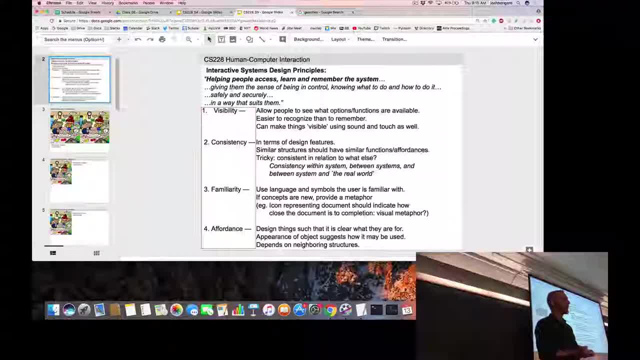 by waving your secondary hand in and out of the frame or field of view of the motion device. not many people are familiar with that particular form of interaction. You're going to have to provide a metaphor or give some sort of signal to the user about what they're supposed. 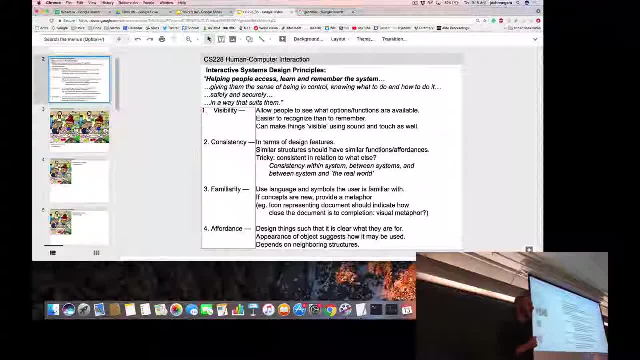 to do. You're going to find this particularly challenging in the final project. When you're doing your user testing, you can't cheat by turning to your roommate and say: listen, here's what you have to do. one, two, three. Remember, your user does not speak English, Right They? 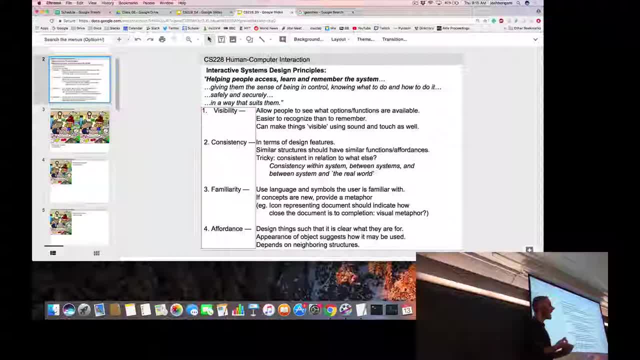 have to learn everything without you telling them what to do. How are they going to realize that from time to time, they need to do that Right? You're going to have to provide a metaphor, If it's familiar things. again, use language. 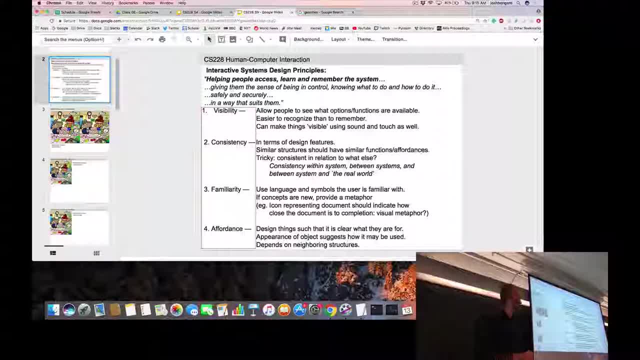 Use familiar language, if you can assume that they speak that language, or symbols, Okay. How about an icon representing a document should indicate how close the document is to completion. There's lots of visual metaphors for that. What are some of them? Some of them. 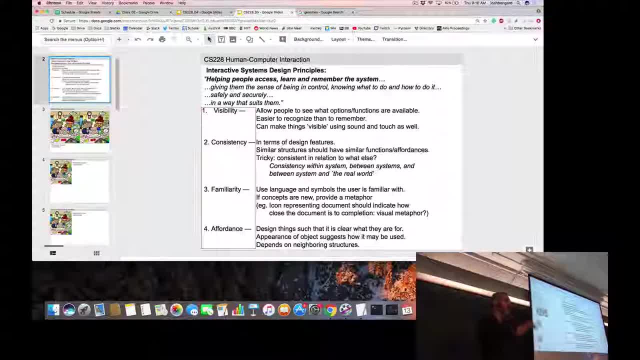 were talking about filling out forms. You're trying to do something. How do you know how close you are to completion? Progress bar- The progress bar kind of universal these days. Anything other than progress bar. If there's symbols representing each step, it might change the appearance of the symbol. 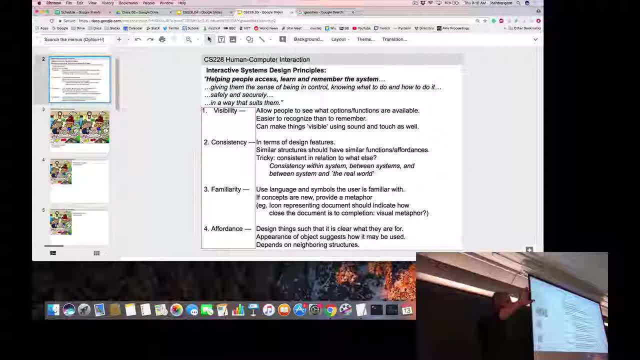 without getting repeated, Absolutely Right. So the symbol itself might change. There's some aspect that you're done, There's the slice of the pie, progress, and so on. Lots of different ways to do that. Okay, This fourth one. this is an idea that comes from psychology, the idea of affordances. 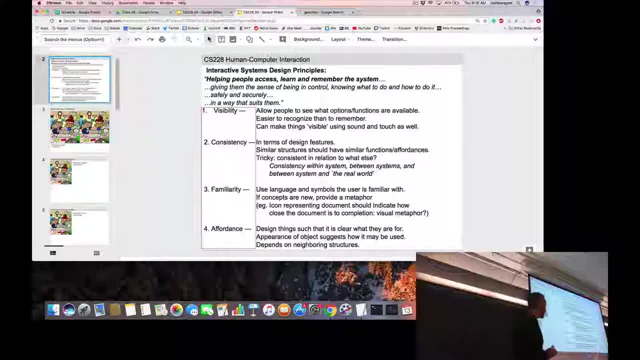 This is an interesting one. We'll talk about this in a moment. Basically, in this case, what we're trying to do is design things that are seen on the screen, or maybe physical devices that the user has to hold or interact with, to advertise what they're for Right. 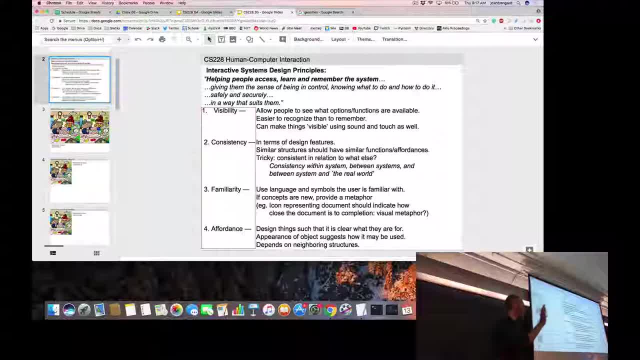 Remember our discussion about verbification. We want to focus not so much on the noun, the thing, but the verb, the way in which the person should interact with it. So the appearance of the object or the icon, or even the sound, we'll see. auditory, We'll talk. 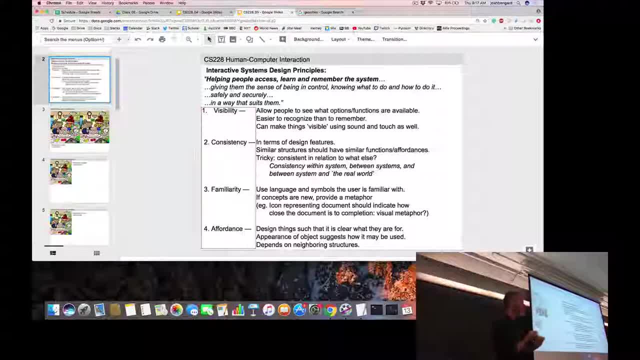 about auditory metaphors in a little while. The appearance of that object should suggest how it should be used. What's an example of an icon that suggests to a user how it should be used? Sorry, A magnifying glass, Exactly Right. Whatever it is, it's going to give you if. 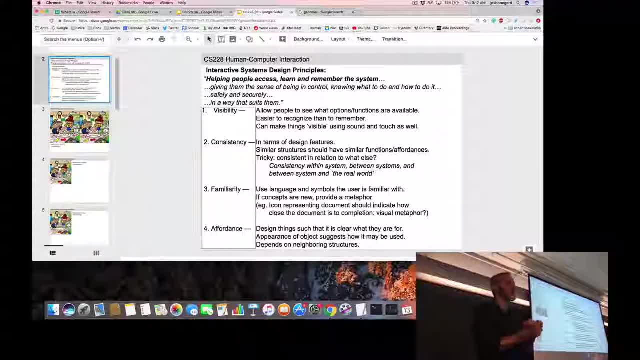 you use it or look through it. even if you're not literally looking through it, it's going to provide detail. Yep, It's a good example. Play pause and next. Play pause and next. Right, We've talked. 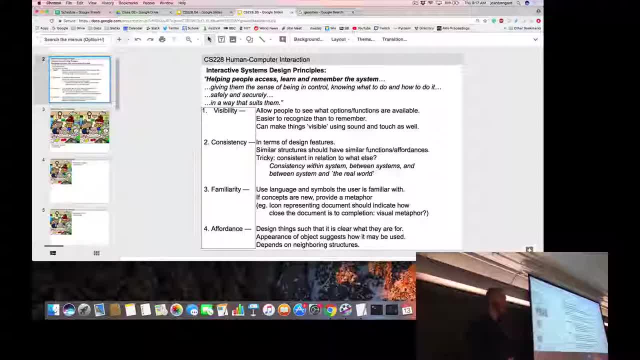 about that one a fair bit. A hand means panning A hand Right. Okay, Hand is tricky Right, Because the human hand does a lot of things. Right Now it tends to be panning, but if you see two, sometimes it means zoom in and 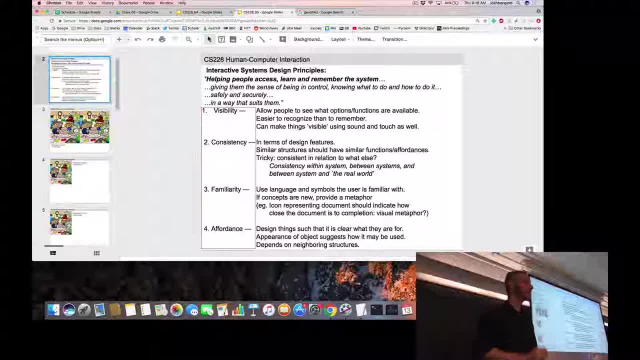 zoom out. Didn't you just start a new program? Yep, That's a good point, Right? So sometimes, with the KISS principle, you might just see a single icon which says interact with me. Right, You can't do anything else except this. 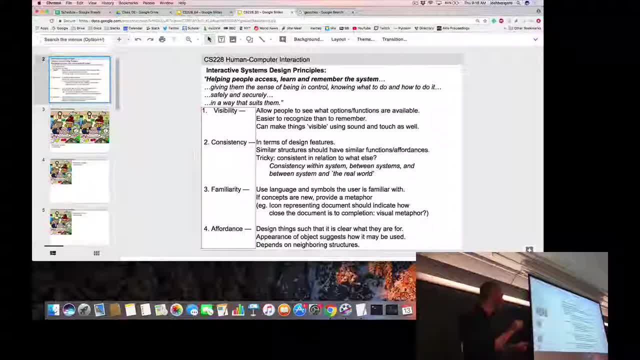 We'll talk about affordances in a moment where often what you infer about that thing has to do with neighboring structure or, in this case, the lack of neighboring structure. If there is nothing else on the screen except a green button, you can be pretty sure what. 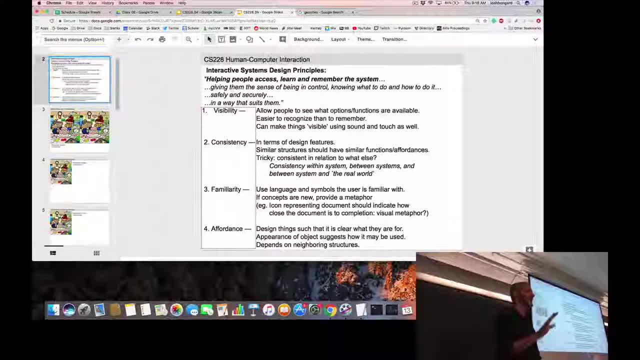 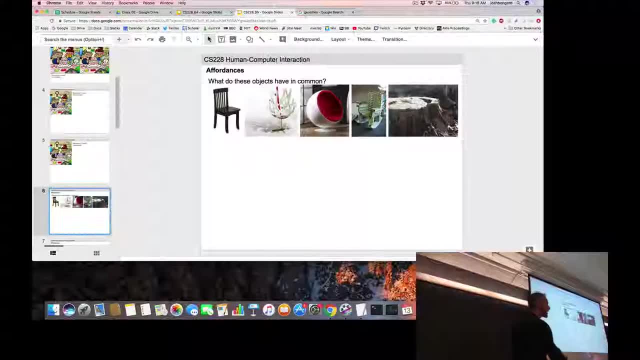 the system is trying to tell you: Don't do anything except press this button. Okay, So let's have a look at affordances Again. let's step outside HCI to try and make this point. Again, this has come from psychology. We're back now to the human system. We need to think about the human visual system. 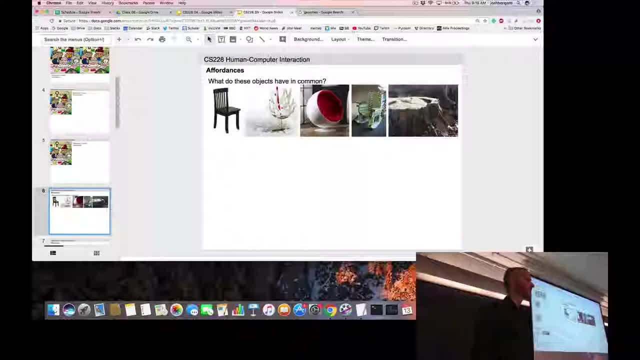 What do these objects have in common? They're all for sitting. They're all for sitting Right. Sometimes, when I ask this question, people say they're all chairs, Right. You could argue about the last one- Not technically a chair, but again. 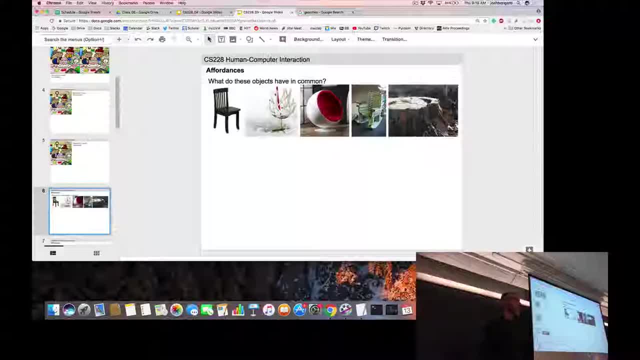 you could argue it Because chair, the noun in our minds is almost synonymous or equal to the act of sitting. So what is a chair In the old days, when people were trying to write computer vision software that would take in an image and recognize chairs or cats or whatever else you wanted? 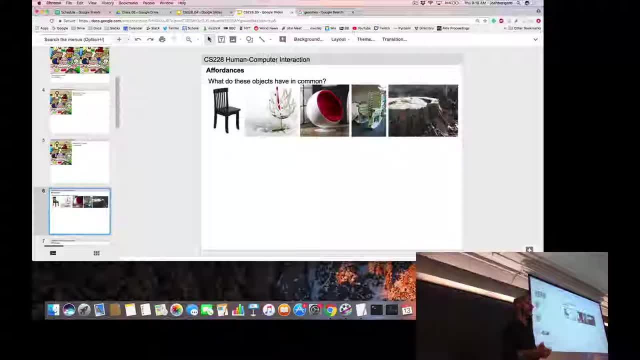 to see in the image. they wrote a lot of code that said a chair has four legs. So look at the image, find a blob of continuous color and see if there are four vertical things coming down from it. If you took that hypothetical software, it would correctly recognize this one as a chair. 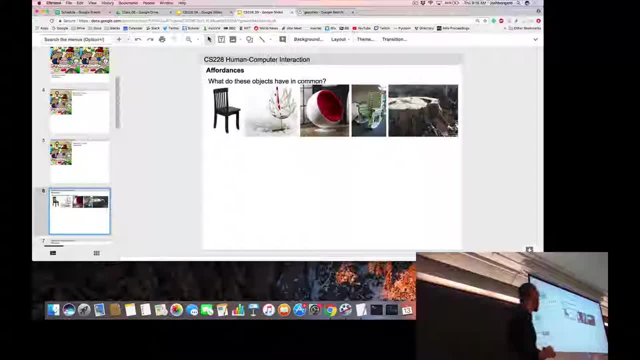 but none of the rest, Right? So then the computer vision designers went back and said: okay, okay, okay, If you see something that has four vertical prongs at the bottom of it, or three, that's a chair. Still doesn't work Right. Back and forth, back and forth. 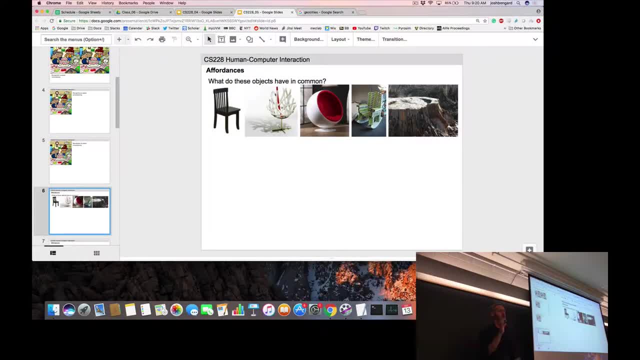 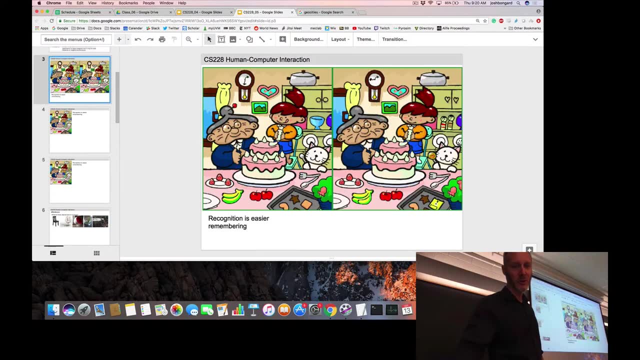 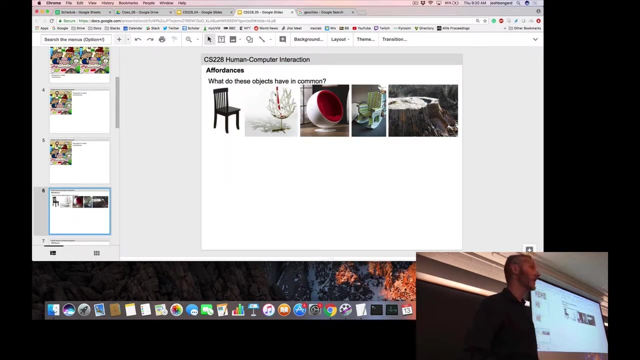 back and forth. Part of the reason why it took so long to create software that could automatically recognize objects in an image is that the designers of that software were not familiar with the human aspect of recognizing affordances. Whether you realize you're doing it or not, 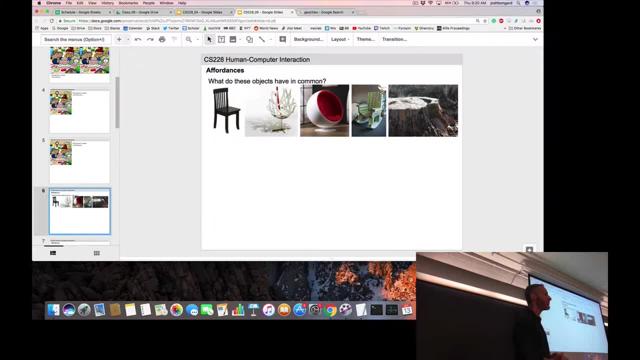 when you look at something and you start to get the idea that maybe the answer I'm looking for is chair, you're not looking at each of these and mentally saying: does it have four legs? Does it have three legs? Does it have a vertical backrest? Right, I picked these five images. 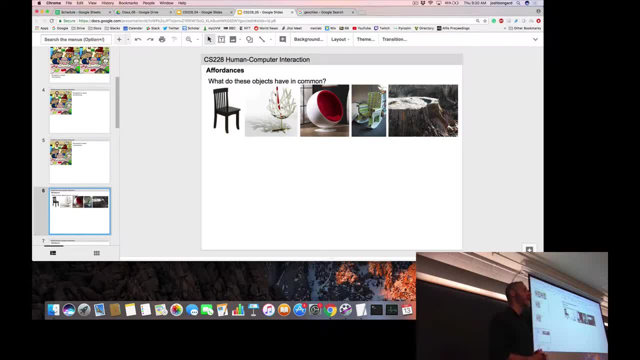 as you can imagine, now to try to explain- And I'm going to try and explode- any possible hypothesis you could come up with for what geometrically constitutes a chair, Because in order to recognize a chair, you're not really paying attention to the geometry Or, more technically, you're not relying on just the 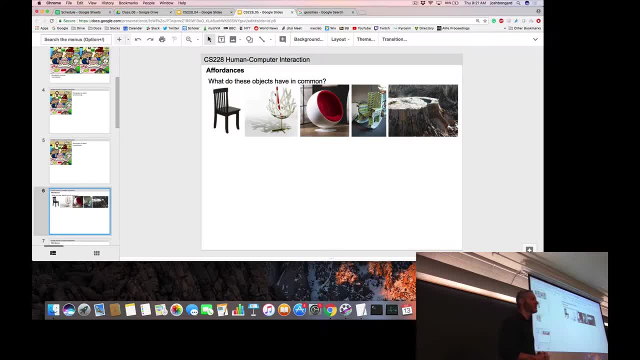 geometry. You're reasoning about the geometry of the object. you see, You're reasoning about your own geometry and your own movement capabilities And you mentally project yourself into the image And you think about what would happen if you sat on the more or less horizontal part. 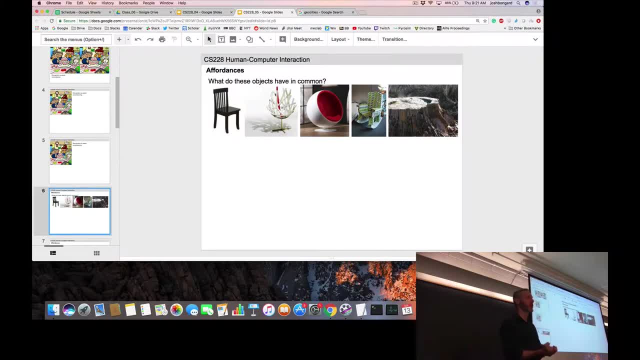 of these objects? Would the act of sitting result or not If I were to put you in an MRI brain imaging device while I asked you this question? the motor strip part of your brain, which is the part that sits right here at the top of your 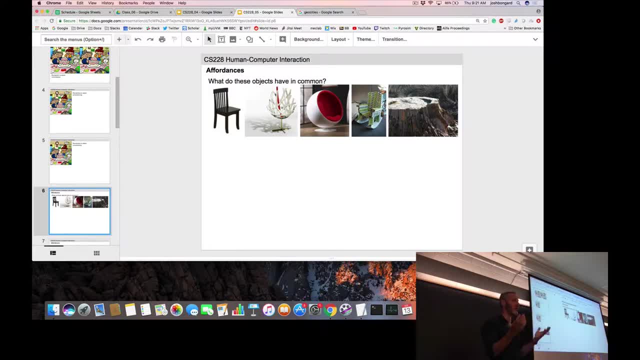 head, the motor strip would light up, which seems strange. Why would the motor part of your brain light up? Why would your brain light up when you're just being asked to recognize chairs or not? Because the same neurons in the motor part of your strip will light up when you're thinking. 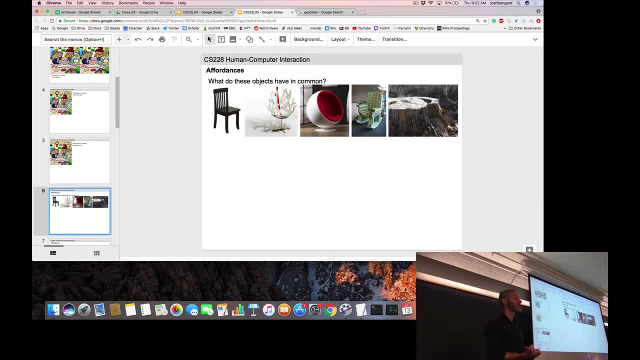 about sitting and when you're actually sitting, Or when you see someone else sitting, Or you see someone in a movie sitting. All of those acts in your brain, more or less, are the same thing: The details of whether you're sitting or imagining yourself sitting or seeing someone. 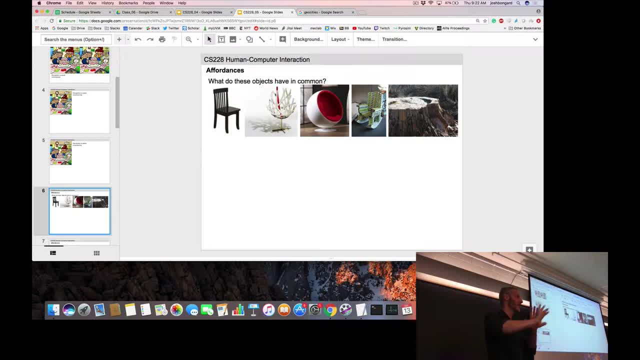 else sitting. those are sort of details that are further down the chain of reasoning. The important thing that links them all together is sitting. Five very different objects with very, very different geometries, but they trigger something in the motor strip. You imagine something When you see a big green button in your app: your motor strip lights. 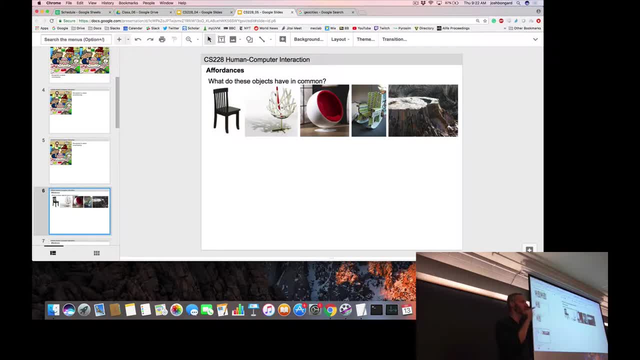 up again because, whether you realize it or not, you're visually seeing yourself pressing the button And you're reasoning about whether it will work. If the button is really small, your motor strip actually has to work harder because your motor strip knows you've got to aim very 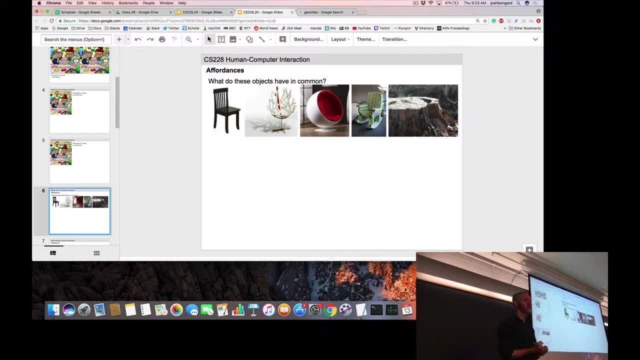 carefully. If the button is big, your user is actually doing less mental work. If you've ever wondered why, in the history of web design, the fonts have gotten larger and there's been more and more white space, In the old days, web pages used to be very packed and dense. 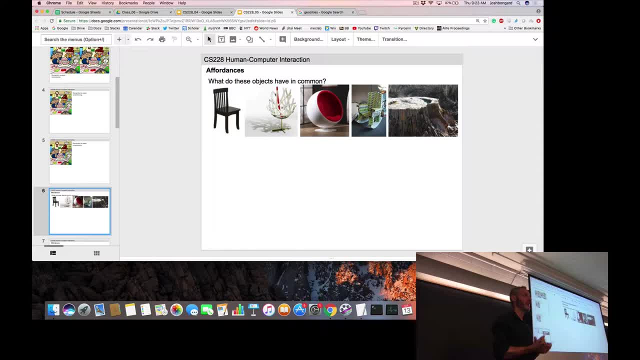 Part of the reason is accessibility. Not everyone has perfect visual acuity so it helps people read, but it also helps the motor strip A lot of what you're reading or seeing in a web page. your brain is trying to imagine how you would interact with that. Can I reach? 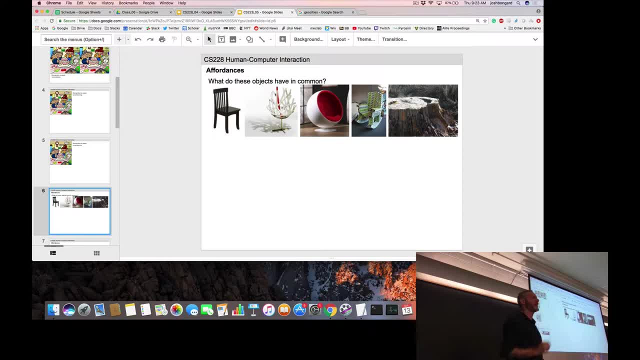 out and click on that link. Could I grab that thing and drag it successfully, right? Could I sit on that object? Okay, What do these four objects have in common? Yep, They're all energy sources. They're all energy sources, right. Again, it's obvious, but you'll realize obviously. 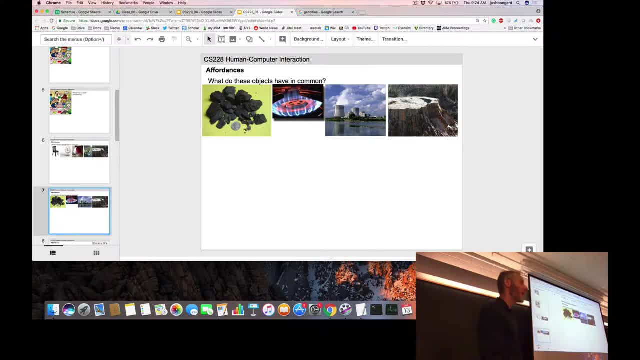 I left the tree stump in there. So a tree stump is not just for one thing, It's for many things. right, And the affordance that the object projects or affords- using old-fashioned language- affords to your visual system. You can think of an affordance as an application. 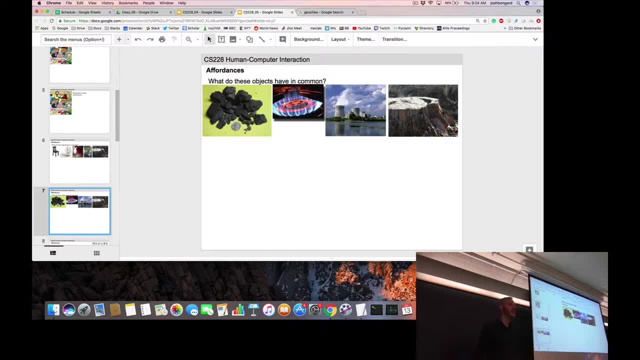 advertisement. The object is saying: you can interact with me in this way. There are thousands of different possible affordances that an object might project, And how that object is presented in what context is going to influence which particular affordance your brain recognizes? right, And that's important when you start to design your interface, right? 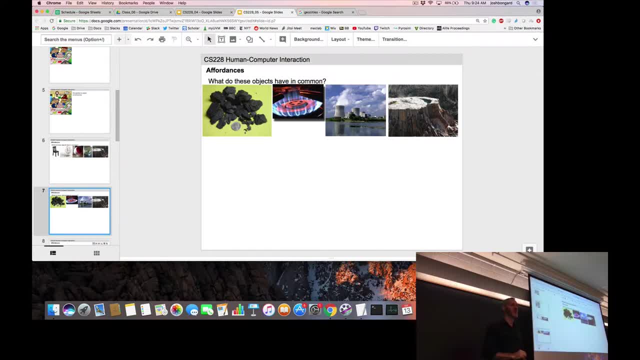 So the green button, depending on what else is on the screen, might say: oh, there's a button. The green button might say, press me now. Or it might say I'm just showing you what buttons look like. for example, It could be a completely different affordance. 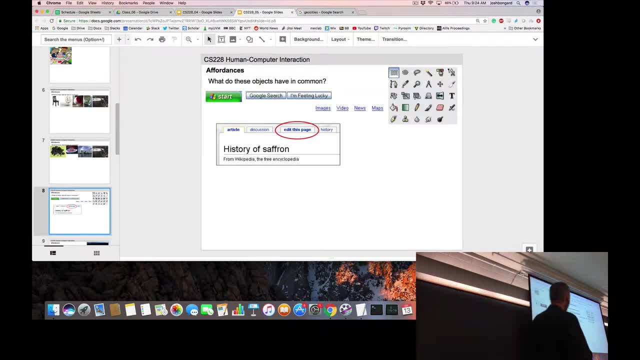 Okay, Let's come back to HCI. Here's again another four or five images. What do all these objects have in common? What is the affordance that they are all projecting to you? There you can click on them right. Another way you know that you're projecting affordances is: people will often use adverbs. 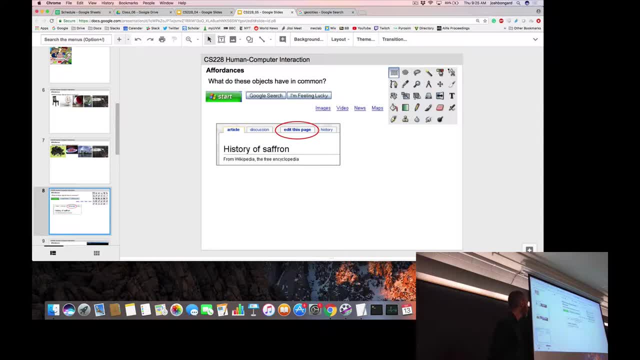 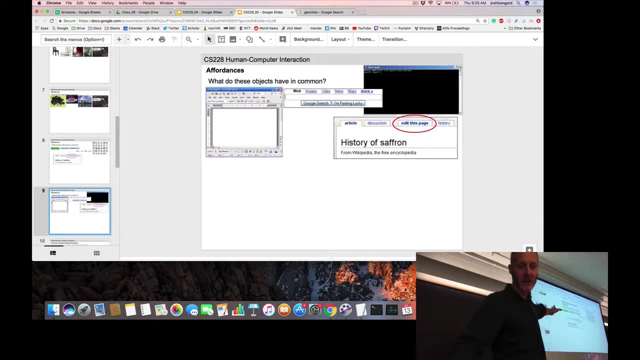 It's clickable- right You can click on them. or it's clickable, Let's play exactly the same game. I'm going to leave one of these objects the same: the Wikipedia page here. What do all of these one, two, three, four objects have in common? What affordance is? 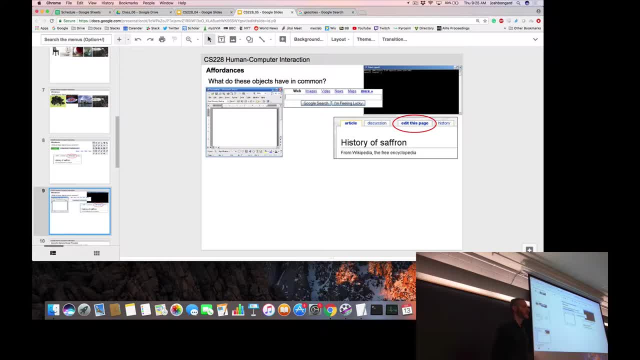 being projected. now You can type on them, right? That's a good description. You can't literally type on edit this page. It's clickable, but you got the affordance right. You know I've designed this page to try and project a particular 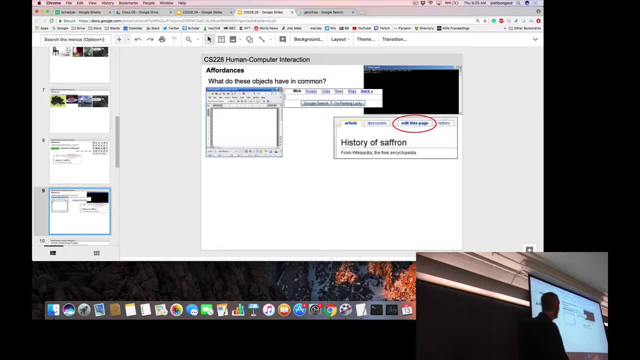 affordance to you, which is, if you click on it or whatever, you will, within the next second or two, be able to start typing in text and you'll see that text reflected back to you right. So now we're thinking about how to design something, to project one affordance. 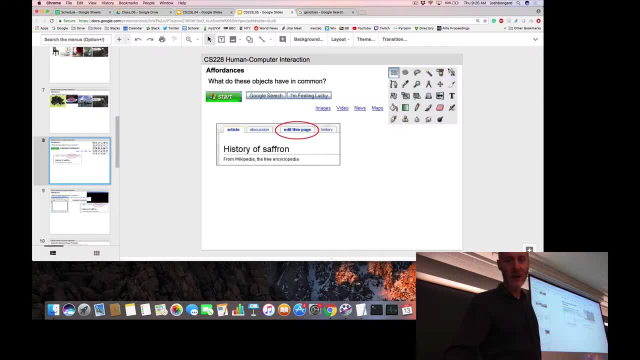 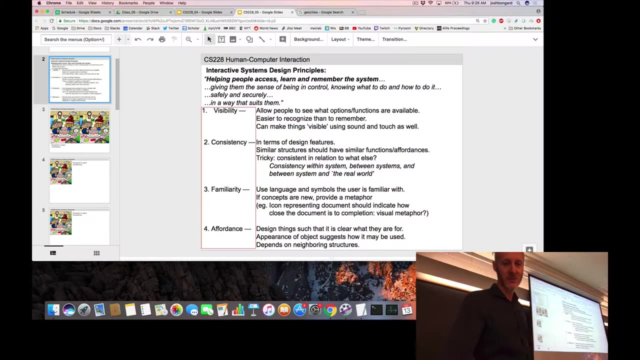 or the other, The edit this page widget. I can change what affordance you infer depending on what else I put around it. right, That's the connection between design and affordances. We'll come back to this idea of affordance as many times in this course. 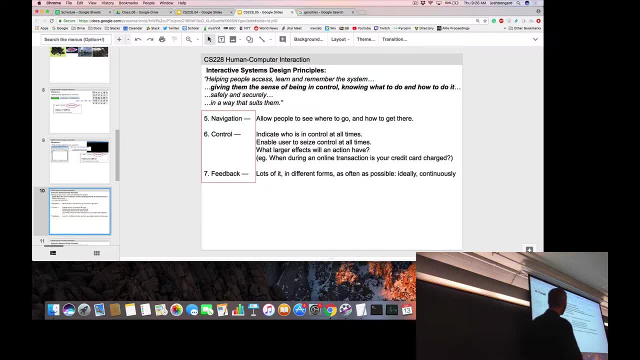 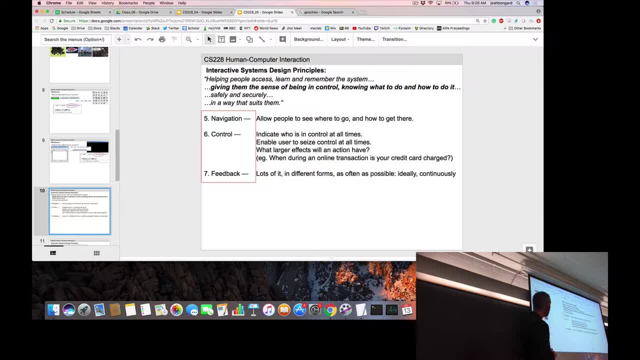 We already talked about the application. We already talked about the application. We already We want to present things to the users, to allow them so that they can see where to go and how to get there. how many different paths are available. I know where I'm going. 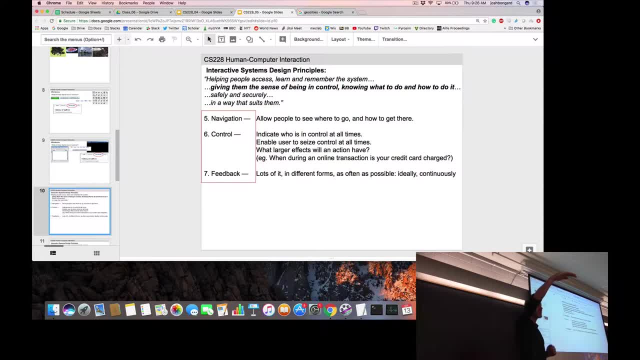 Can I see that there is more than one path to get there? Can I see that some of those paths? given my expertise or lack of expertise with the system, I can see that some of those paths are shorter than others. What are some examples of software systems? 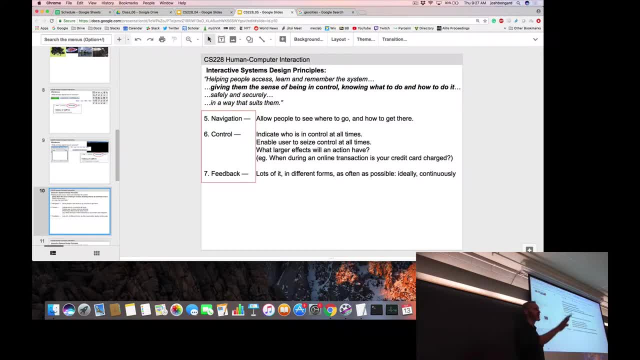 that project navigation clues. So we already talked about the progress bar. That one's kind of obvious. When you hover over buttons, in some applications it'll give you the hot keys, Absolutely right. So sometimes if you hover over a button, 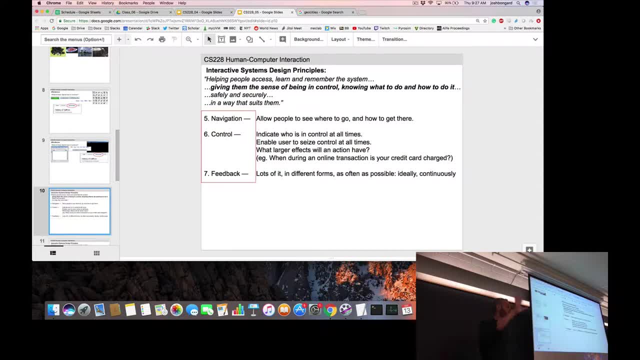 it'll say there's a shortcut, there's a shorter path, But it'll usually these days hide all that information, assuming that, again, you don't want to confuse the users If it's a power user and they're looking for the hot keys. 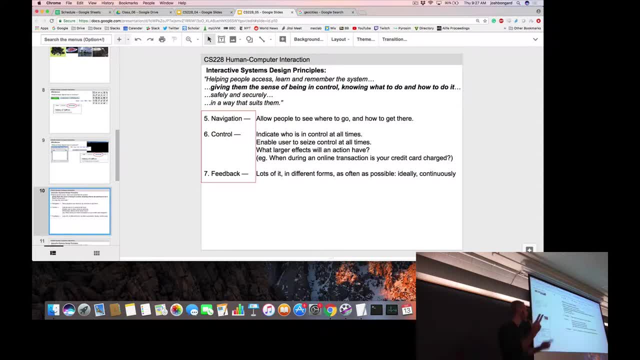 then, by definition, since they're a power user, they'll know where to go. They'll know where to go looking for those shortcuts, They'll know where to go navigating to look for it. OK, Control, This one is very important. 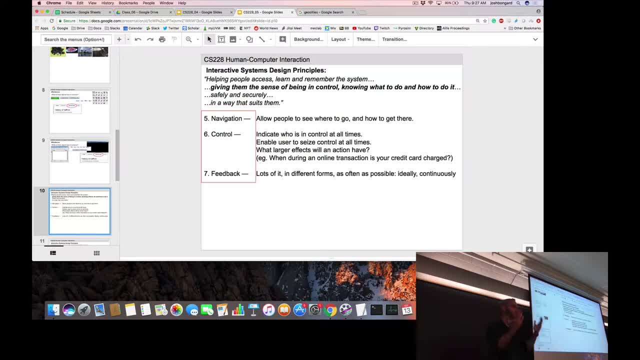 Most of the time these days, with most modern applications, you can either control or seize control immediately. In the old days, given limitations of technology, sometimes the technology said stop, I need to do something for a while before I let you take back control. 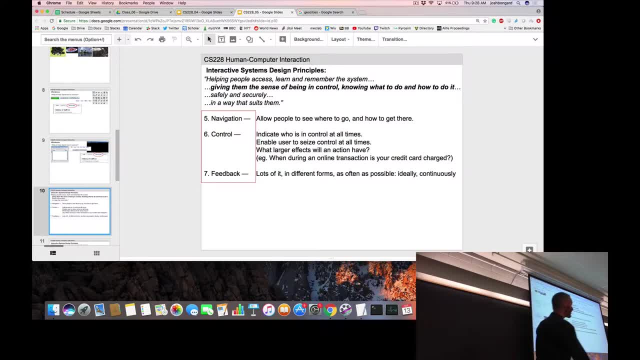 It's relatively rare these days, but it's still does exist. What are some systems you can think of where there is this advertisement, where the system says: you do something and now stop. stop, I need to do something for a while. 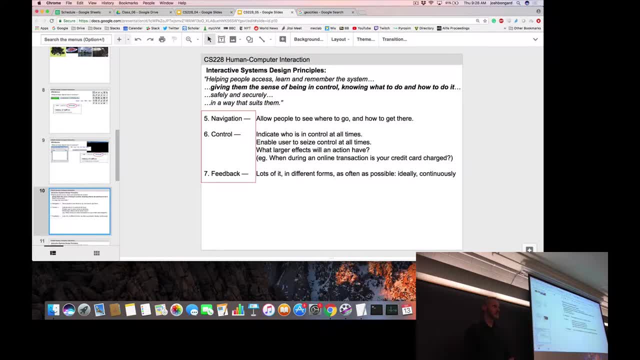 and I'll let you know when I'm ready for you to take control again. Well, like, TeamViews will allow people to use your computer and they'll let you know: hey, you can get control, or? hey, That's a great example. 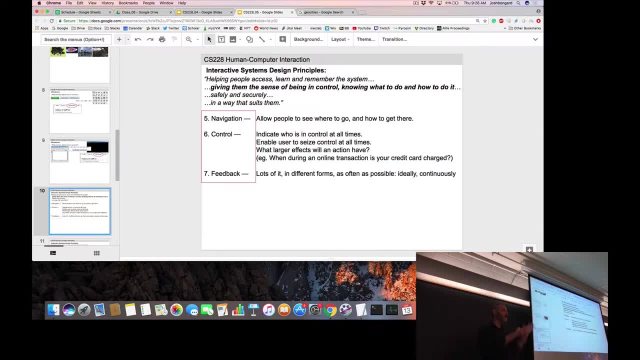 So TeamViewer, right. So remote desktop, where someone else remotely can literally take over and run your computer as if it's their own. A lot of safety and security issues there pretty important, So it's extra important to let the user know. 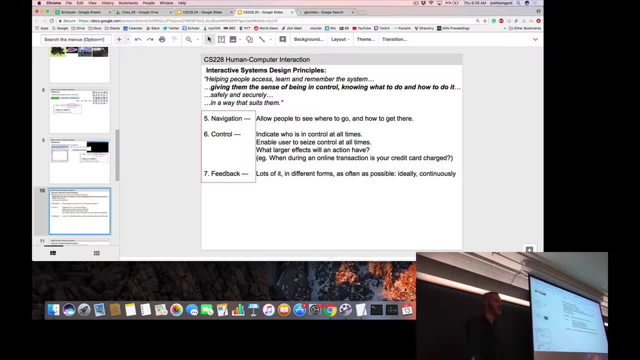 or the person who's physically sitting in front of the screen know who's in control at this time. It's a good example, Yep, Something like cut scenes in a video game, where a director takes control and shows you something Absolutely right. 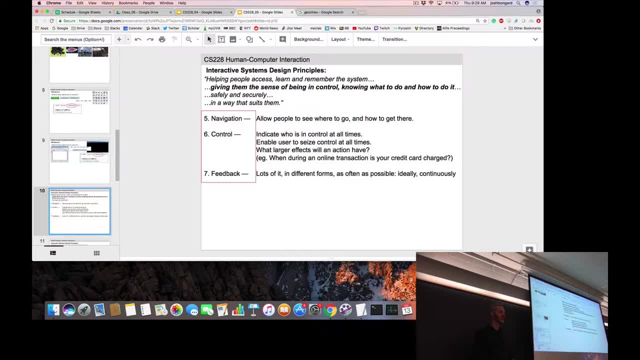 And they make sure that it's very pretty so that you're willing to sort of sit there for a few seconds and watch the cut scene in the video game. Good example: Loading screens. they'll always try to display some sort of either just like GIF icon. 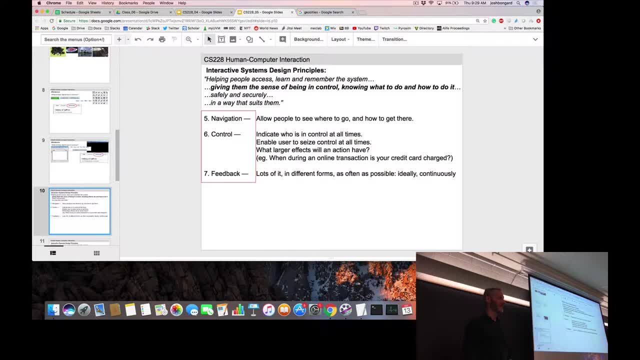 or it's better if the loading bar or something like that, so that you know that you're out of control for a reason when you're showing up at something Absolutely right. So again, rare these days, but if you have a really computationally intensive application. 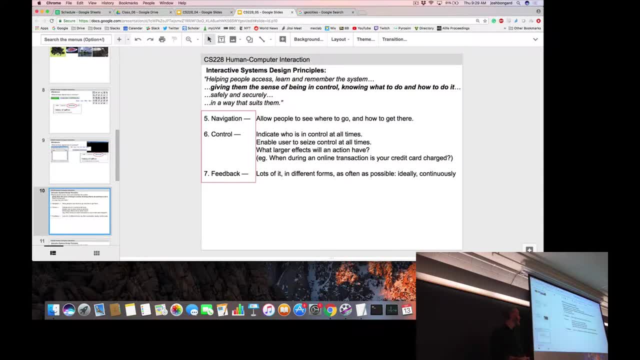 like a game or something else. there might be a load screen. They'll try and put something up there to keep you occupied, so you don't get too frustrated. Often it's: hey, you're clearly here and you're willing to wait a little bit. 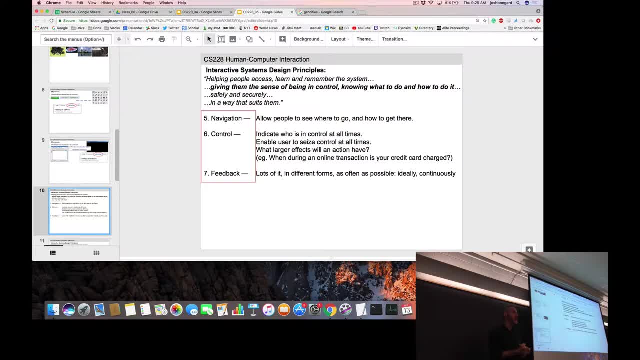 so you're invested in this system. Let me maybe show you some hot keys, or here's a hint or a tip of how to do things better, which is again a subtle psychological game that's being played here. I know you're bored or you're about to get frustrated. 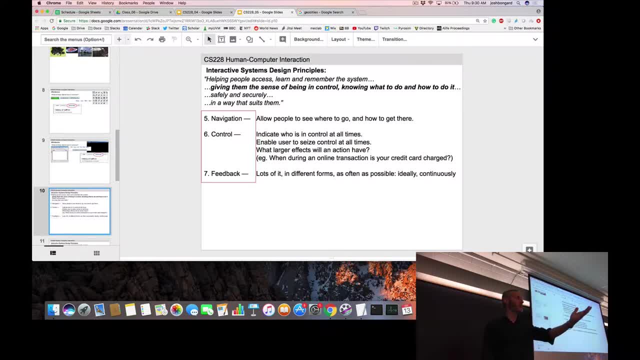 I know you are, so here's something that might help you do things faster, quicker or better elsewhere in the system. right, It's paying you back for your patience. Systems that are impolite and just put up a loading screen and nothing else and they're assuming that you're just 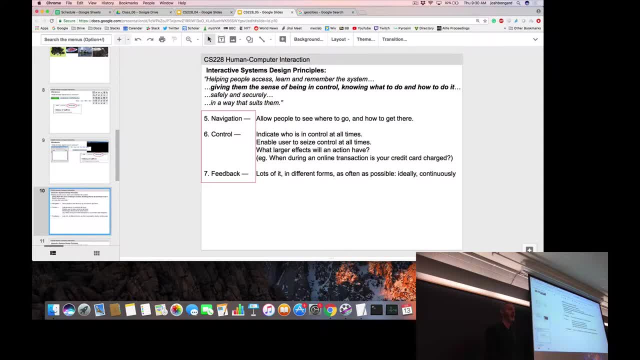 going to sit there and wait. they may not even tell you how long you have to wait. Are you waiting a few seconds or a few hours? They're rude. They're not letting you know how long. They're not valuing your time right. 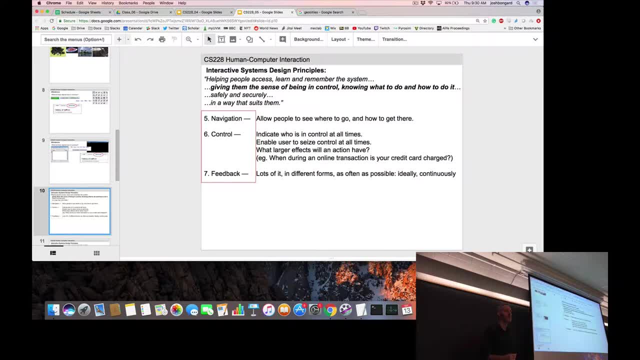 And you'll see people talk about systems like that. They will anthropomorphize, right. This system was super rude. It didn't care about me. It was wasting my time. Of course the system wasn't actually consciously wasting your time. 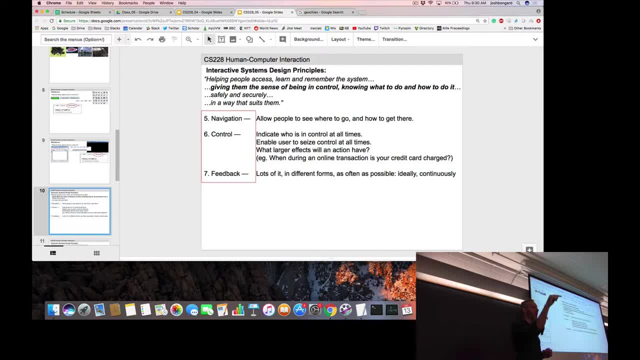 But the designers of the system fail to think about what would be the emotional state of somebody during the two seconds or the one minute of this process during which they're not in control. Very important to think about those particular aspects of the system. Yes, 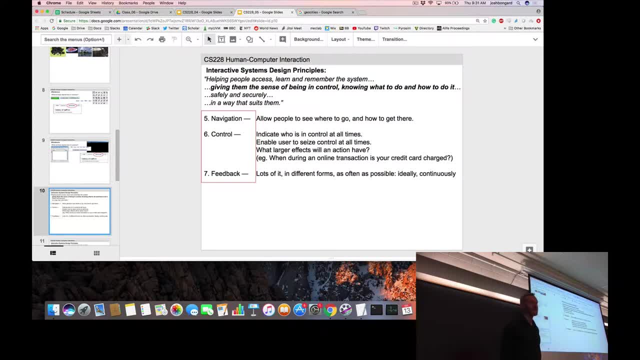 According to that, I feel like recently, in the past couple of years, I've seen progress cards, not only the progress cards that will save, but Absolutely right. So I'm assuming that if you're frustrated, you're waiting. 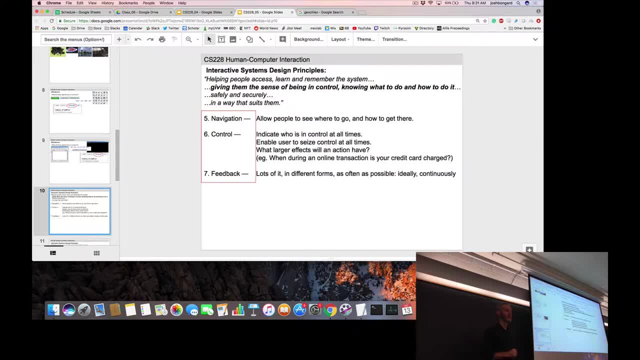 you want an explanation for why you're waiting, right, Which is again a very subtle trade-off, because often we don't want to be giving too much information, right. We're often trying to hide internal complexity away from the user so that they can focus just on the things. 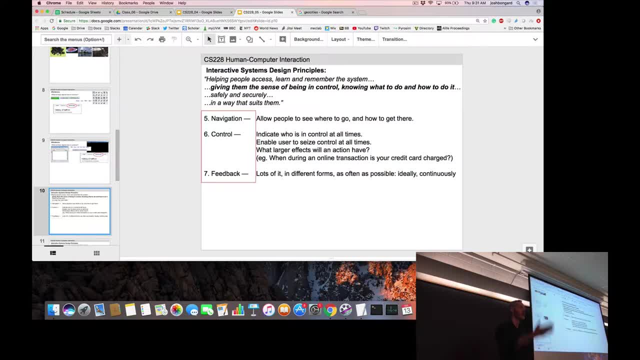 they're trying to do. But there are exceptions to that rule and it's jeringling and it's not just the way it is. I've seen those times when I'm frustrated. Why is this taking so long? I may be asking: why is this taking so long? 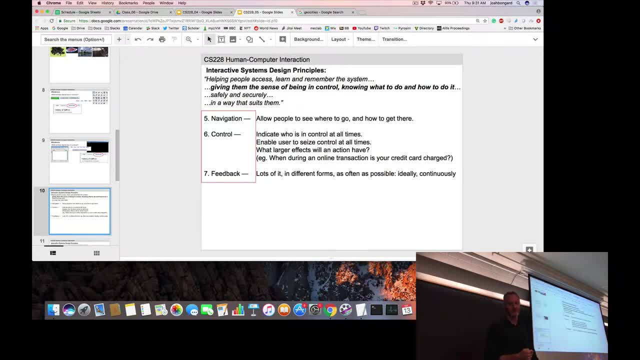 In a literal way. I want an answer. What is it that you're doing that requires me to wait? Okay, so sometimes you need to provide feedback. Again, this one is tricky. Lots of it in different forms, as often as possible. 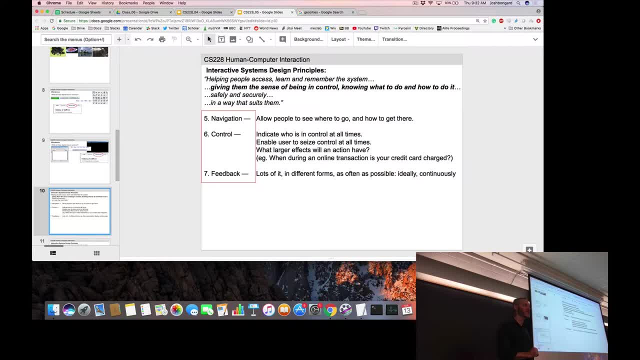 ideally continuously, as long as that feedback is also not distracting, right? It's just a matter of what the user wants to get, right? And a lot of well-designed systems fall foul of their users. for exactly that: There is feedback, but it's a little bit too distracting. 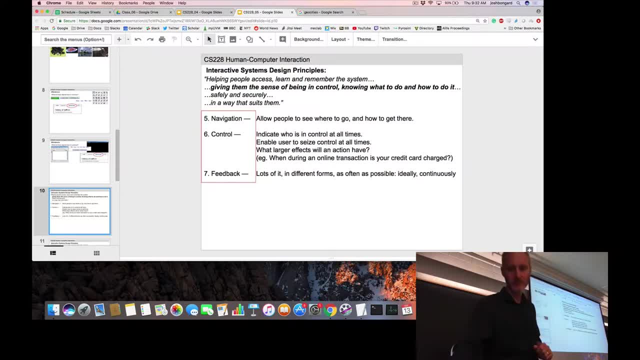 given what the person wants to do. right, It depends on context, where they are OK, Safely and securely. we've sort of talked about this before. We need to think about that. Are we going to adopt a proactive or reactive approach? 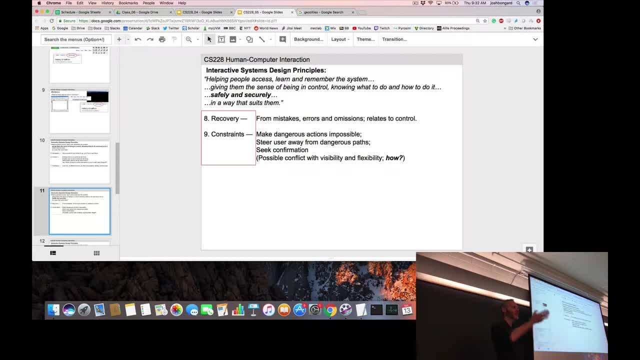 or stance to safety? Are we going to make mistakes and then give them the options to back up and recover from that Errors and omissions, leaving things out Again? this is sort of related to control. Are you going to take away my ability to make mistakes? 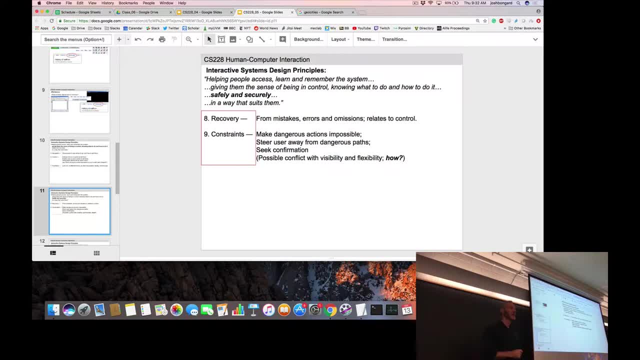 You may adopt a proactive stance to safety in which you're going to say: are you sure you want to do X, Are you double sure you want to do X? And so on. Related to that. again, this proactive stance is building in constraints. 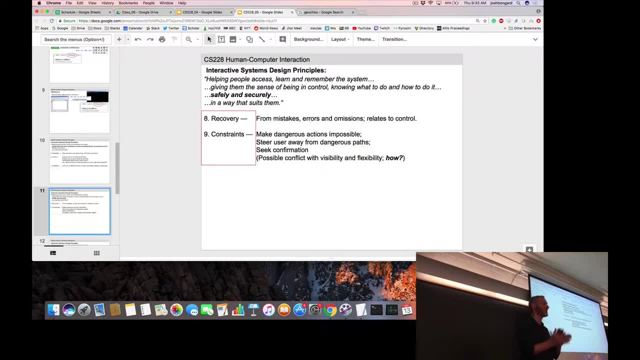 You may limit what people can do to steer them away from potentially dangerous paths, unless you give them a little test or they signal somehow through the interaction that they know what they're doing. But that's tricky because now you have a system that's adaptive. 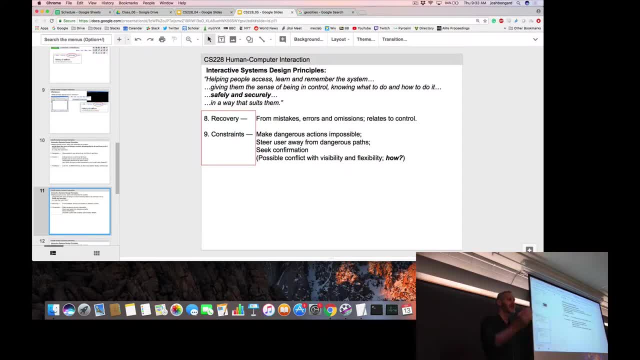 It's trying to infer the ability or the clearance level of the user before allowing them to do dangerous actions. OK, Clearly this is going to conflict with visibility and flexibility. In what ways? Obviously, if you're building constraints, they're going to be less flexible. 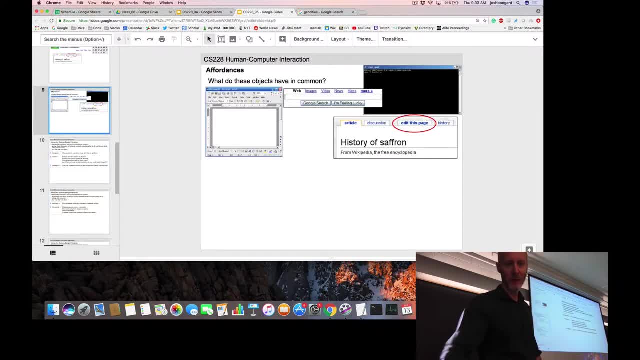 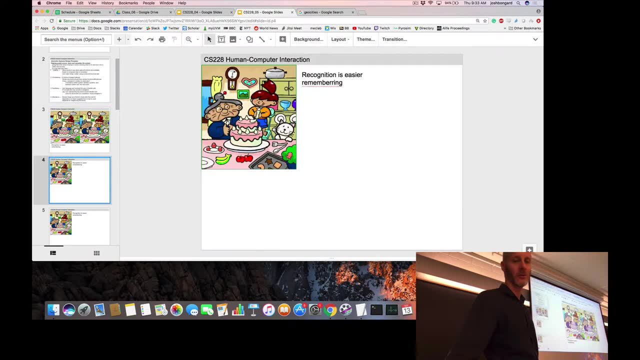 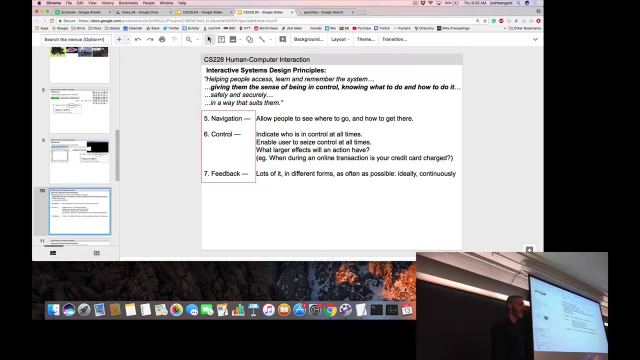 How does this relate to visibility? I'll just back up for a moment here. Visibility at the top there, Allowing people what to see is available, Yes, Well, software. You can try to put that on the web page and it will stop and will have it just say. 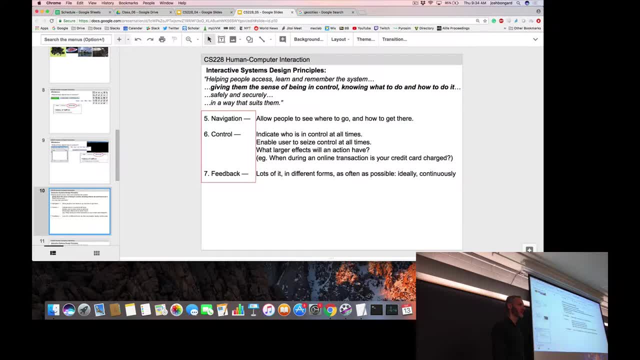 write a warning sign that says, hey, this website isn't safe. And then you have to do advanced options. Absolutely So it's Presenting a lot of information there in order to be safe. Other examples: How a lot of emails will automatically. 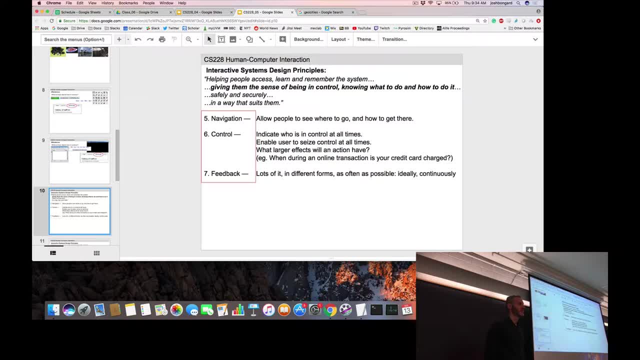 block images from certain emails that they think are suspicious. Absolutely, And some of them won't tell you that, Or at least it will be hidden away a little bit for your own good. Sometimes that's OK, But again you've got to be very careful. 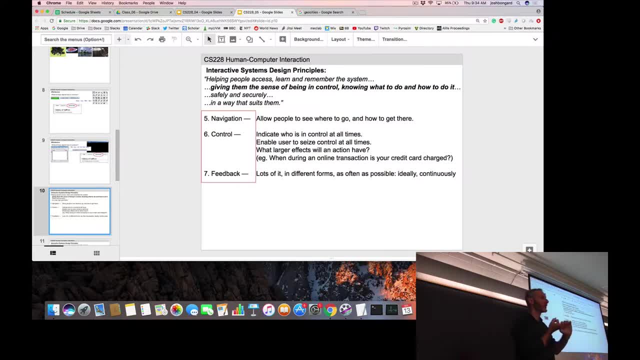 You've got to think about who you're dealing with. what are they doing and in what context. If you want to make something safe or apply constraints, often You want to hide potentially dangerous options. But again, are you sure that the user doesn't want to know? 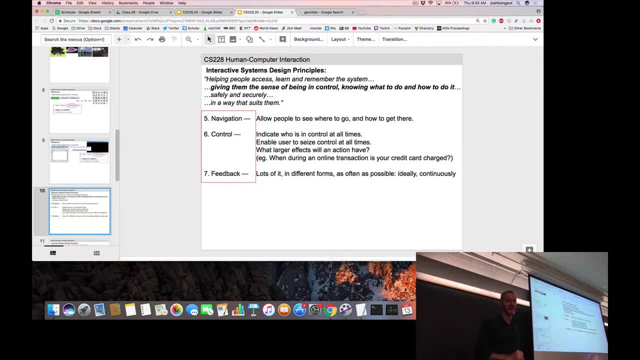 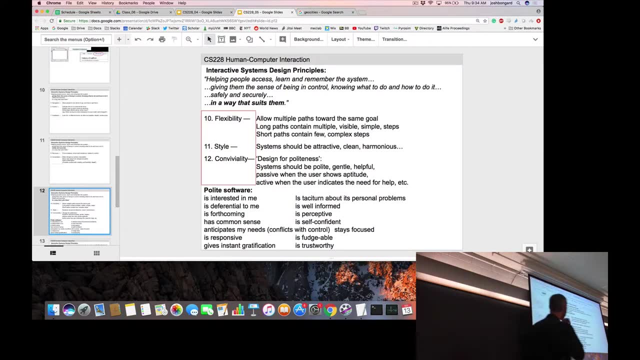 Or can you make it relatively easy for them to bring that stuff back and make it visible if they request it? OK, Let's finish off the last ones here. Again, as always, we're thinking about these sort of design principles or rules of thumb. 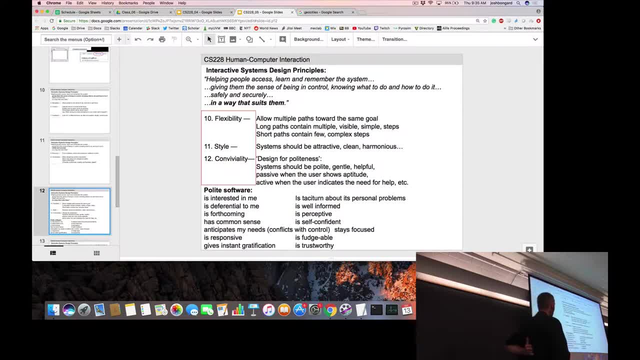 And as we go we're getting into more and more subjective territory. Often We want to try and make our system as flexible as possible so that people can carry out whatever it is they want to do in the way that suits them. We've talked about two obvious paths that usually 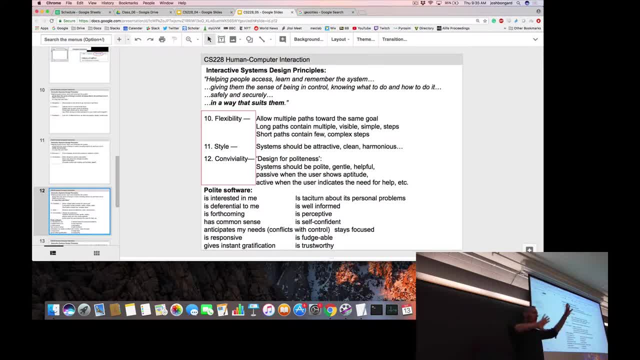 exist in most software systems, which is the menuing or the icon or the graphical path, And then there is the hidden, the cryptic, the efficient hot keys or remembered commands path, the power user path and the novice path. What are some other applications you can think of? 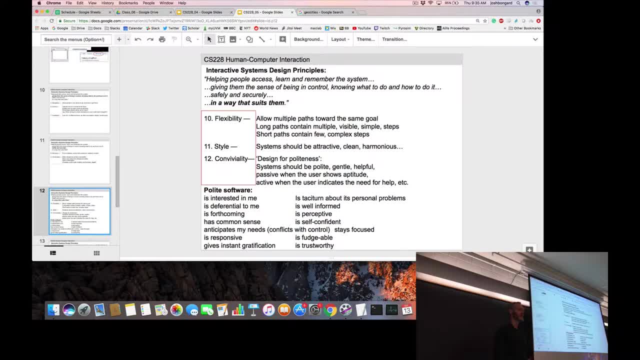 where there are many, many different paths to accomplish the same thing. In either a Google or in an operating system, you can either get the files with the command line or through the file pattern meter. Absolutely So. on most operating systems there are usually two paths. 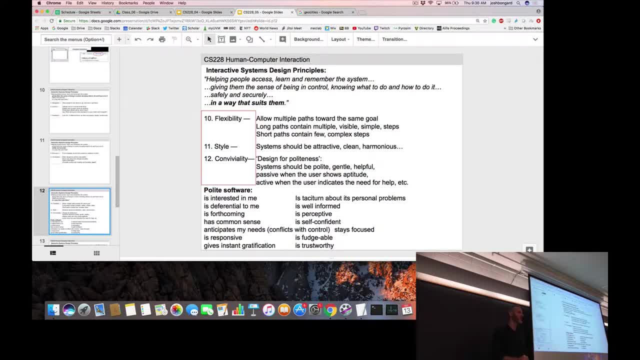 I can click through to find it or I can type something in to find it. Those two paths tend to be ubiquitous. Can you think of examples where there's more than those two paths? A lot of really basic functions like copy and paste? 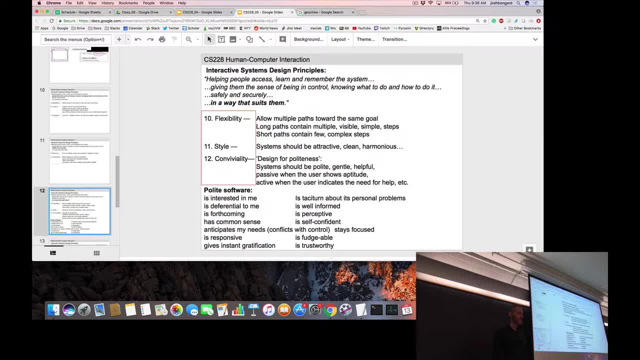 You can either do it with a mouse or you can do it with any keyboard. Yep, OK, So again we're back now to through the mouse or the keyboard right, So sort of clicking on things or typing in commands Saving a file. 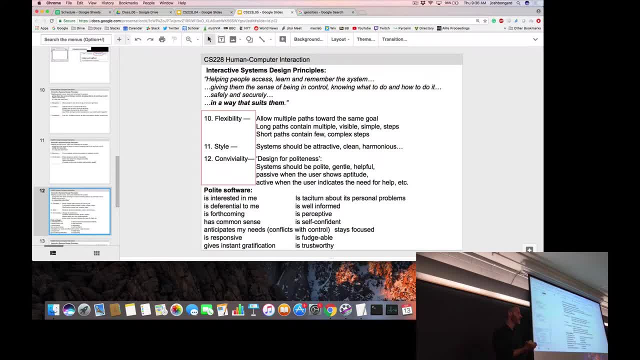 Saving a file. There's multiple ways to save a file, right. You can do the drop-down menu and do the save and then select what you want to save it as. Or you can just like you talk, you read, you press and save. 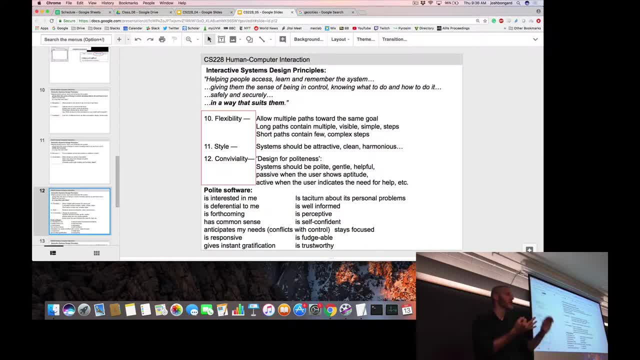 Save button. OK, So you can just press the Save button, navigate through the menus, hit Control-S, three paths And, in a non-technological example like cooking, OK, So you could like. there's tons of ways to make a meal. 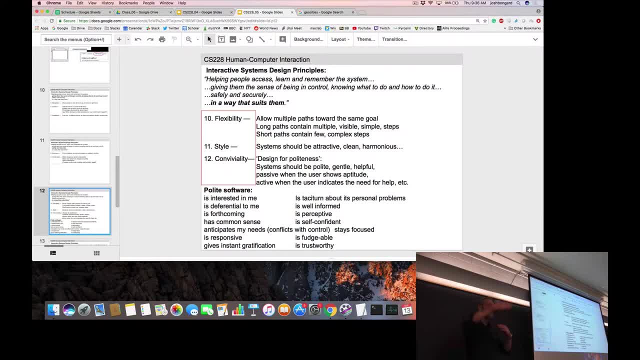 but like just cooking. That's a great example, right? So if you're thinking about a sequence of steps like a recipe, right, and a lot of those in software systems, does the order matter In the deliverables for this class? 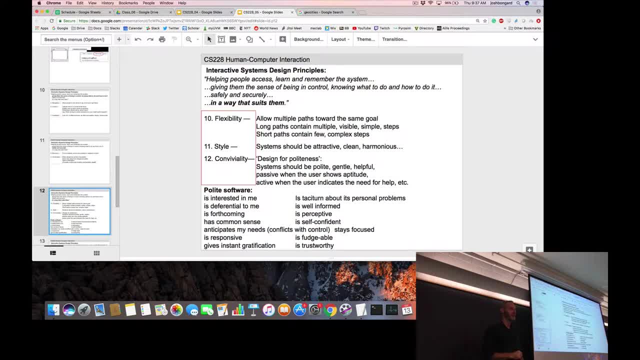 absolutely order matters. right, You can't jump to step 23.. You know you're going to get into trouble. That one's kind of obvious. But there are other situations where order maybe doesn't matter so much And there may be sort of signals saying 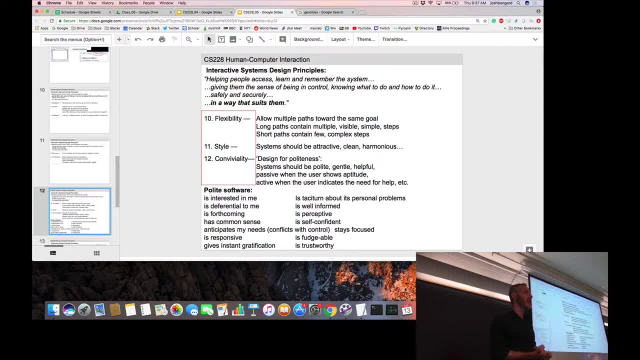 here's the different ways you can do it: Option A, B, C, D and E. Let's link this idea of flexibility to navigation. Think about the internet. You're trying to go from page to page on the internet. There's lots of different ways to do it. 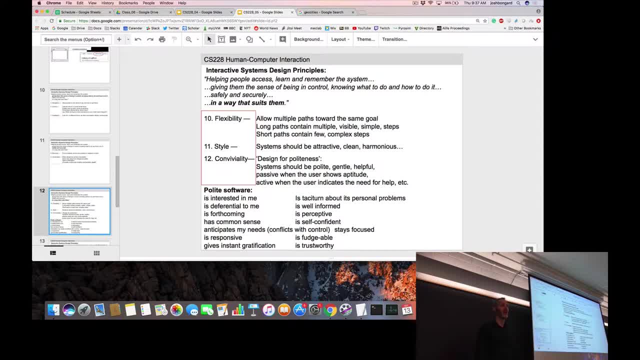 That's the beauty of the internet: It's a network. There are a lot of paths from point A to point B. What are the different ways that you navigate from point A to point B on the web? You could click a hot link. 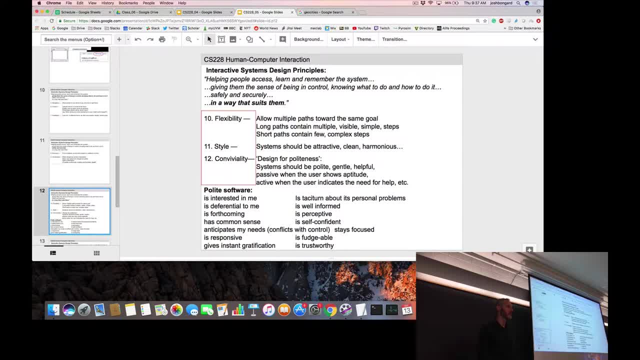 You can click a hot link right. I click and go from A to B. What else It could be in your history? Go to history, right. Maybe there are places that I visit often, So again, we're going to talk more about navigation, right. 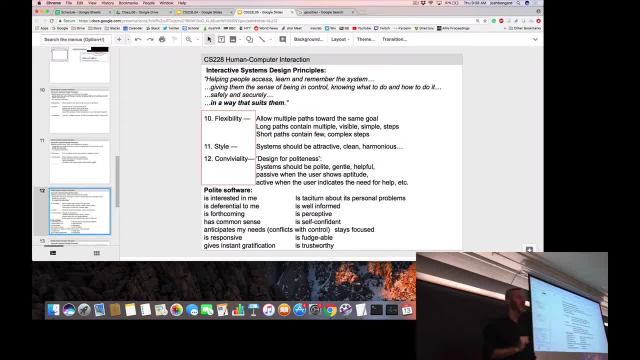 So often. systems these days are annotating automatically Places that you visit often, and they're making it easy for you to call up those annotations, like in your history, and go right there. There's two paths. I know that smartphones now based on your location will recommend apps, at least. 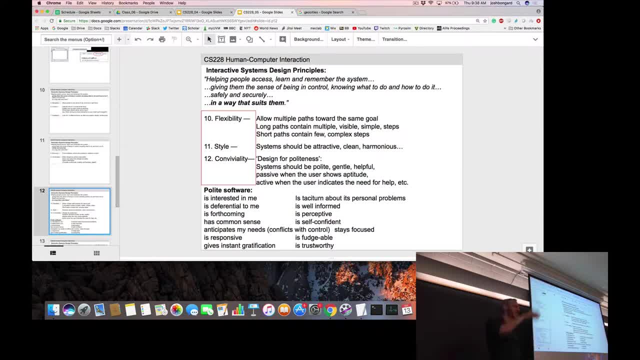 Okay, That's right. So let's imagine, though, we're trying to get to a specific page, right? So, again, geolocation is a good one, right? It might say the location, the thing you're trying to pull up, is relevant to this position. 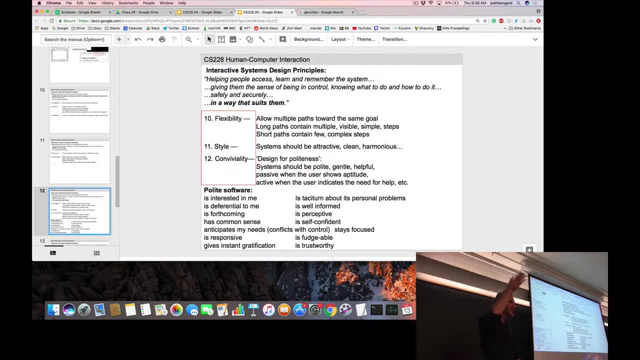 or not. So I know you're trying to get to B, but maybe B is not relevant at your current location. You can type in directly to the server from the command line, right? So there's sort of direct paths. Sorry, You could Google it, right. 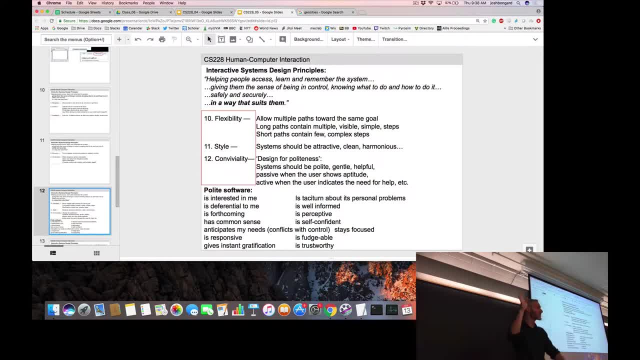 We could search for it and click on it. So search is another option. What else? If you know the IP address- right, the hardcore way of getting there- you could type it in or type in the URL or the IP itself. Okay, 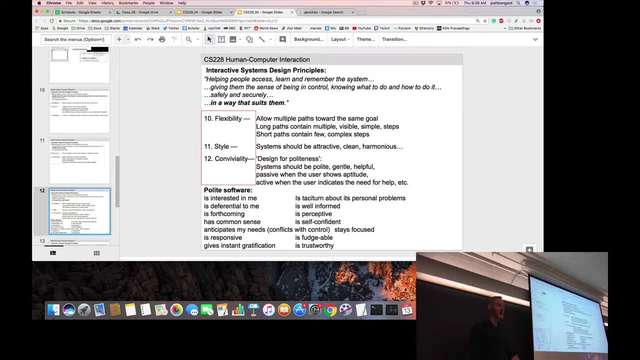 So there are lots of different ways to travel through the internet, which again might seem obvious, but that's part of the reason why the net is so popular. There are a bunch of Wikipedia games you can play. So, for example, I can give you two random Wikipedia pages and I can tell you you can. 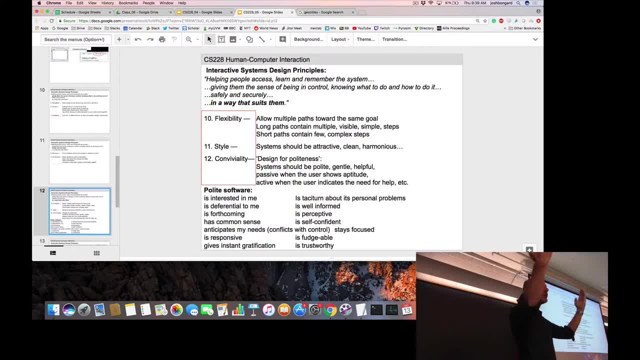 only click on links in page A. What are the fewest links you need to click on to get to page B? Right, There are a bunch of games like that. There's another game where, on any Wikipedia page, you have to click on the first link. 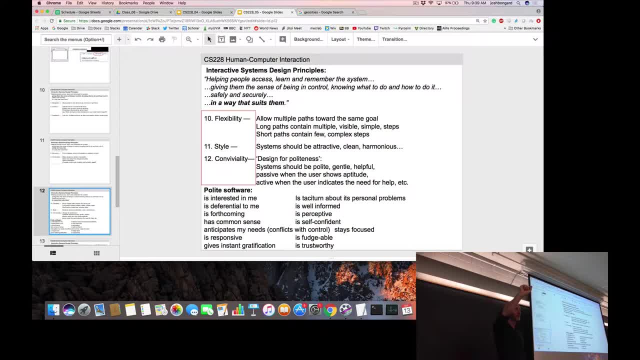 in the text And the new page that comes up. you click on the first link in the text on that page And, amazingly, which nobody designed, you will eventually end. no matter where you start, they all converge on one page. What is it? 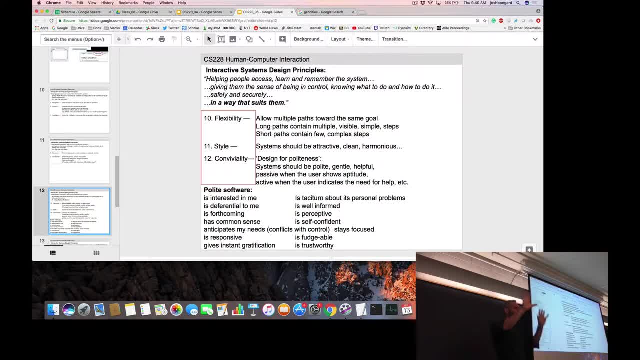 Not menu. Now you've got to click the first link in the text. So we're trying to restrict our movement through one page. We're trying to restrict our movement through one page. What is it? We're trying to restrict our movement through Wikipedia to semantic space, right? 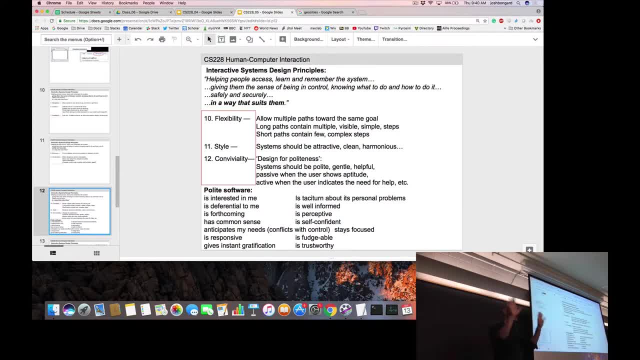 All the topics of human knowledge. If you know, don't say it. I know you don't have your device now so you can't play it After class. go play that Wikipedia page and you'll see where you end up. 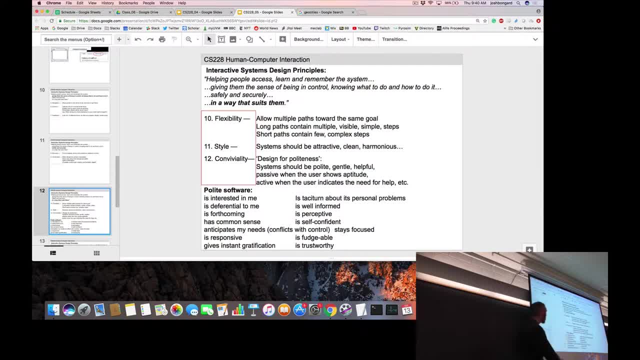 Kind of interesting. Okay, Style- This one is kind of obvious in HCI. We want things to be attractive, clean, simple, harmonious. Again, these are kind of vague. What exactly do we mean by that? Later we're going to talk about ways of trying to actually measure. 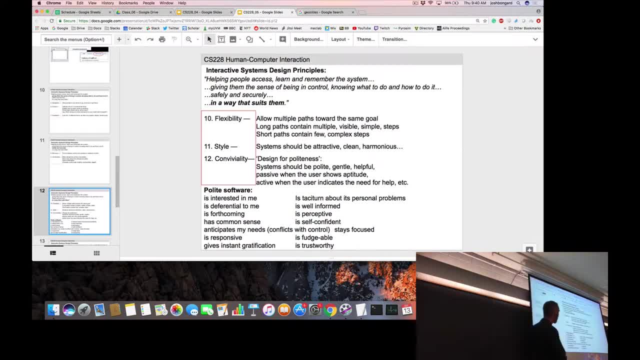 Okay, These aspects. We've spent a bit of time now already talking about convivial software, right Software itself. unless you're an animist, the software is not actually polite or actually rude, but people will attribute those human qualities to the software. 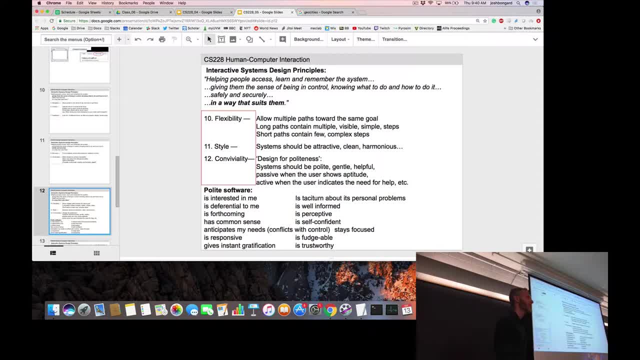 So often, if people have a good experience with your software and you ask them to describe it, they'll say: oh, the system was interested in me. The Duolingo owl really cares about my education. There was a reason why he or she was so adamant in trying to get me to come back right. 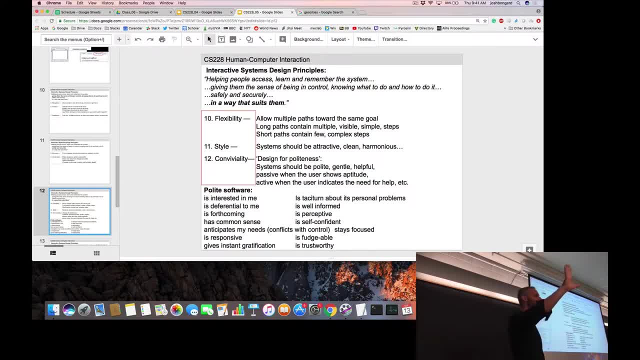 It's deferential to me, So if a notification comes up, it should provide an easy way for you to get rid of the notification. I know I'm bothering you. I know you're in charge. If you don't need me, just say so, right. 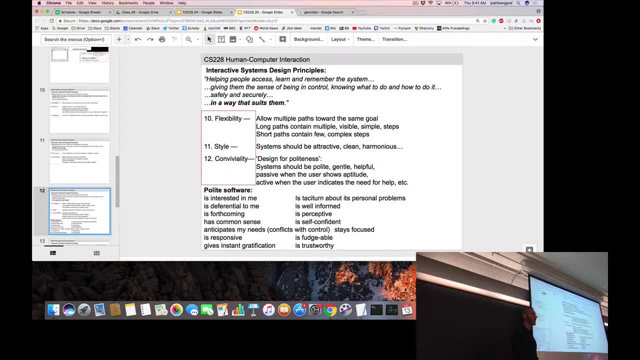 It's forthcoming. So if you say, listen, I want to know why I'm waiting so long on this load page, it immediately has an answer for you. Software has common sense. It's a good thing It has common sense. What does that mean? 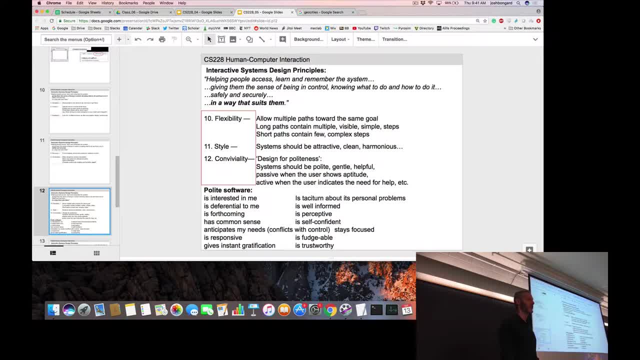 A lot of software does not have common sense. What examples, what aspects of software might cause a user to come away saying, yeah, that system had sort of common sense. I would say it has common sense if it conforms to your own common sense. 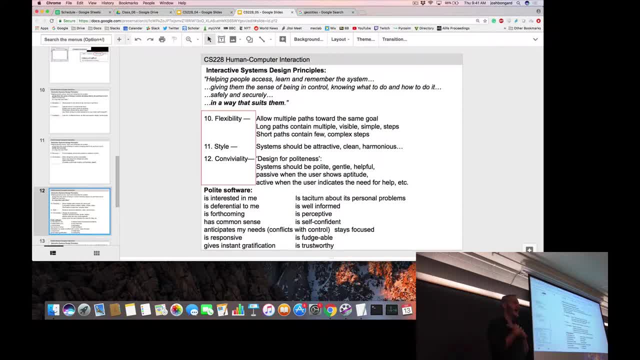 OK, Right, So we talked about that before. Identity: I have common sense. I don't blindly follow the rules. even if the rules don't apply in this situation, I can sort of adapt, And this system does as well. What are examples of systems that actually do that? 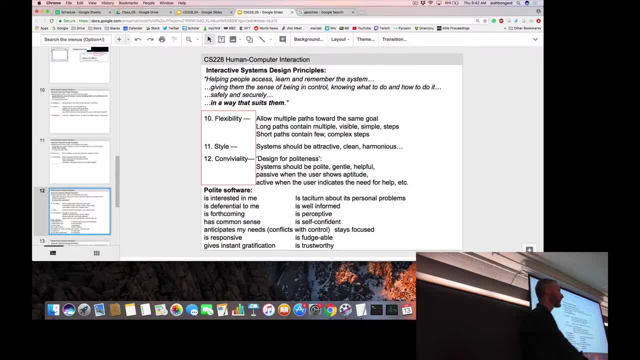 They sort of exhibit common sense. That's a great example, right? So imagine you write an app where, if the person closes it without saving, the system just throws away what you were working on and doesn't tell you: right, You didn't say save. 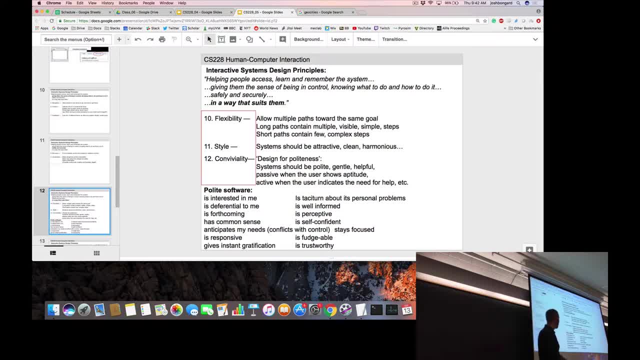 I did exactly what you told me to do. Right, It's perfectly logical. Not a lot of common sense, Right, It seems so obvious. you probably wouldn't program a system to do that, But there are more subtle examples of that, Right. 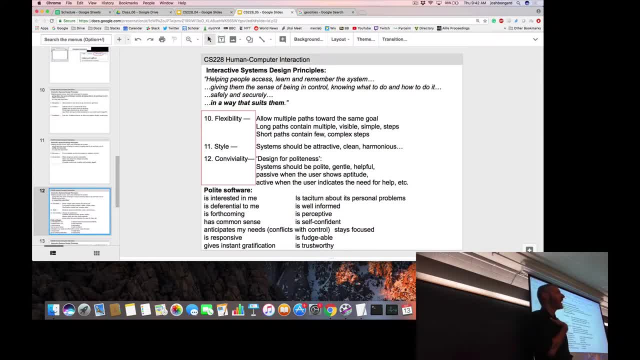 Where the user has expectations. Right. I'm human, I know I'm fallible, I'm going to forget things, But there's some obvious things that I'm usually going to forget that I expect you, the system, to remember and do. 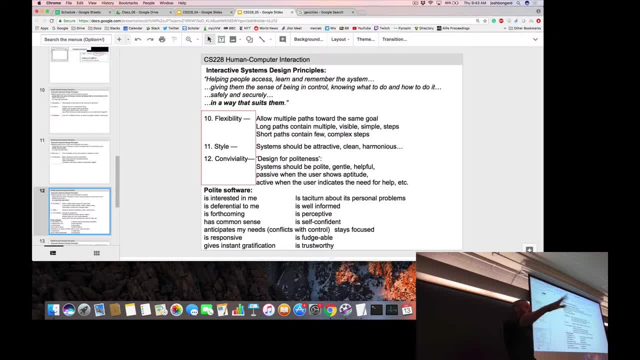 Right, You have common sense, And the common sense I might want you to have is that you have common sense, Right, And the common sense I might want you to have is that humans are fallible. Okay, It might anticipate my needs. 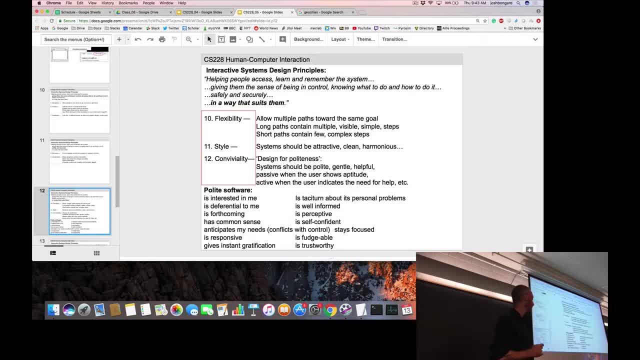 But this one is pretty tricky. It can often conflict with control. It's responsive to me, It gives instant gratification. Right Again, you don't want a system that says: wait a second, I'll give you an answer to your question in a minute. 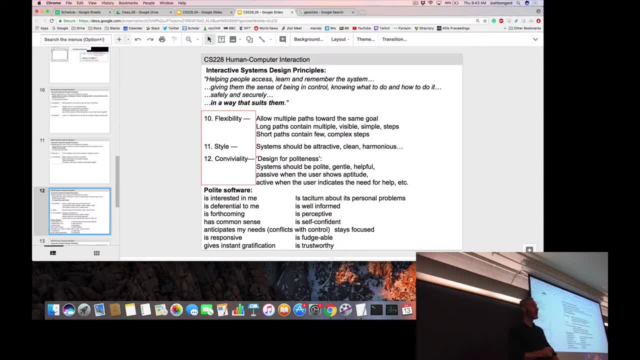 Right, It's taciturn about its personal problems. If you remember the Windows blue screen of death, whenever the computer died, it would come up with an error message. Right, It would say: wait a second, I'll give you an answer to your question in a minute. 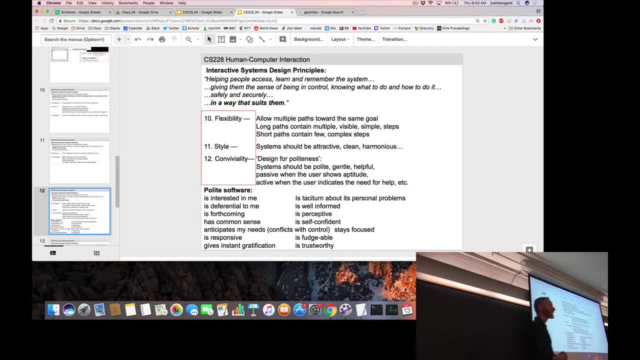 Right, It's taciturn about its personal problems. If you remember the Windows blue screen of death, whenever the computer died it would come up with an error message. Right Same thing, but with an error message Warning. I failed because of error 13672.3, which, as you obviously know, is about some. 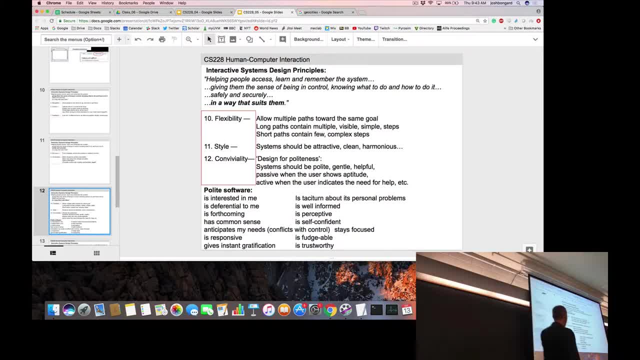 BIOS detail I've never heard about before. Right, Most users of Windows machines at that time did not care which particular error caused their computer to crash. What they cared about was: fine, you crashed. You're not perfect. Shut down and restart as quickly as possible. 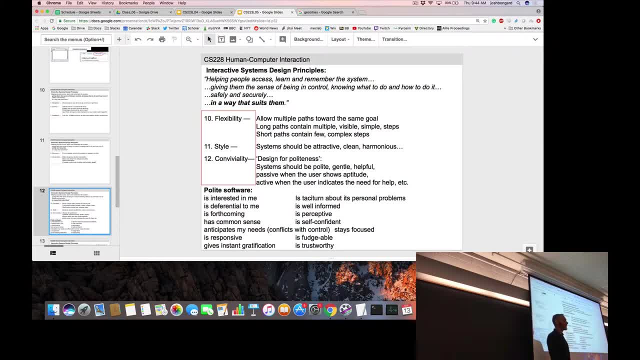 Don't spend time telling me about what your problems are. are, I don't care, but on the other hand, sometimes you may want to know why are you taking so long? as long as your ass, then it might be forthcoming. it may be forthcoming. you give you information about what's. what's going on. it's well. 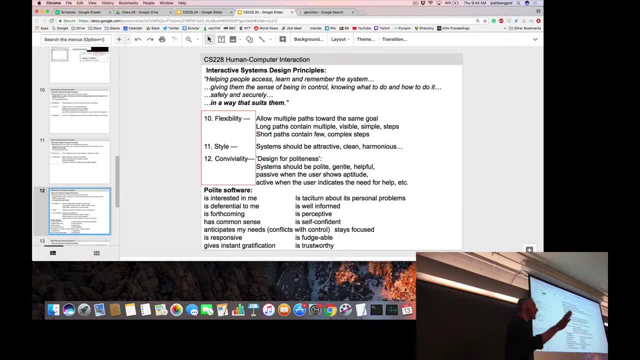 informed. it sort of knows what's going on and so forth. it's self-confident. it doesn't ask you at every moment. did you mean this? do you want me to do a or B? do you want me to use this widget or that widget? just get on with it, right, okay? 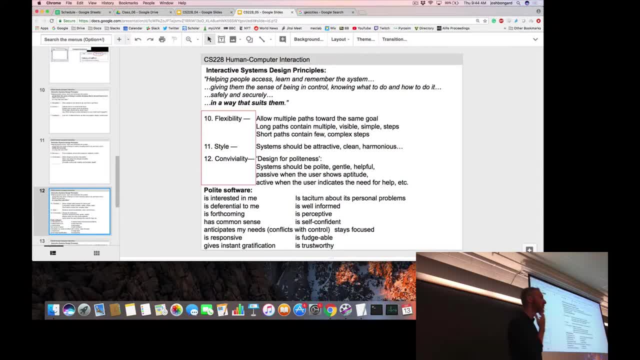 it stays focused on the task. it's fungible. let's end with that one. what is fungible mean or what are some obvious examples of fungible software? autocorrect- absolutely right. autocorrect, again, took a long time to get right and it's not perfect, and the web is full of hilarious examples of where it was. 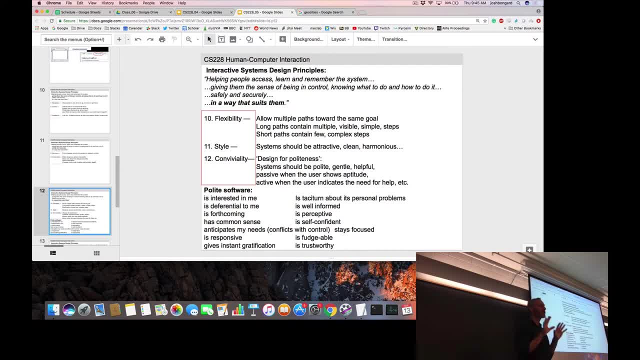 it right, but fungible humans don't type words perfectly all the time. clean things up, okay, leave things there. you have a quiz due tonight. no office hours for me today, but Jack does have his office hours and I'll see you on Tuesday.